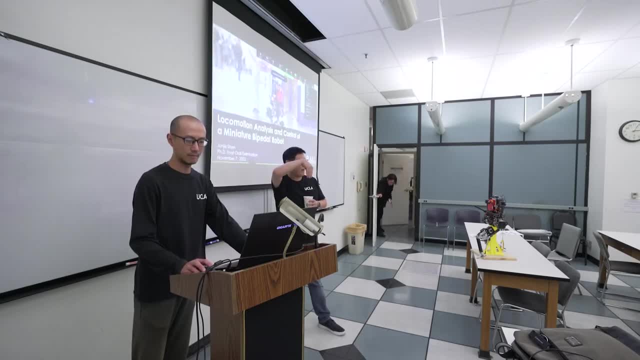 contribution. His main baby was that single wheel balancing robots. You probably remember that Umbro thing, but we decided to change this topic. We want to attack some more challenging topics, so we changed it to a bipedal locomotion robot. So yeah, without any further ado, it's all yours. 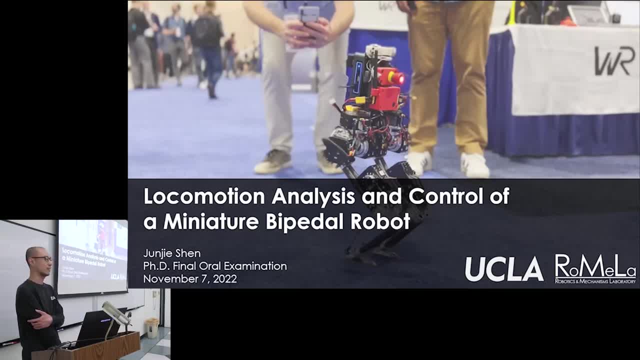 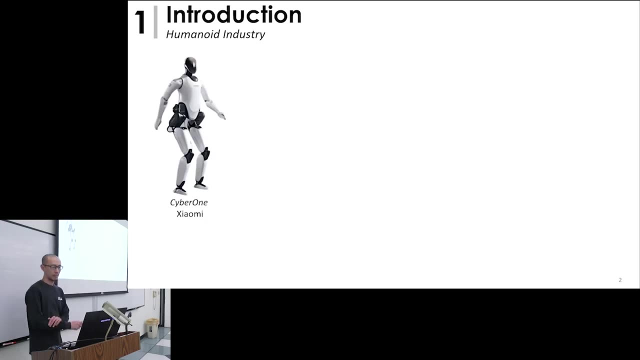 Okay, good afternoon everyone. My name is Junjie and welcome to my dissertation defense, And the topic is locomotion analysis and control of a miniature bipedal robot. So recently, the topic of humanoid robots has been placed under the spotlight. Cyborg One, Xiaomi's first humanoid robot, debuted this. okay, so Xiaomi's first. 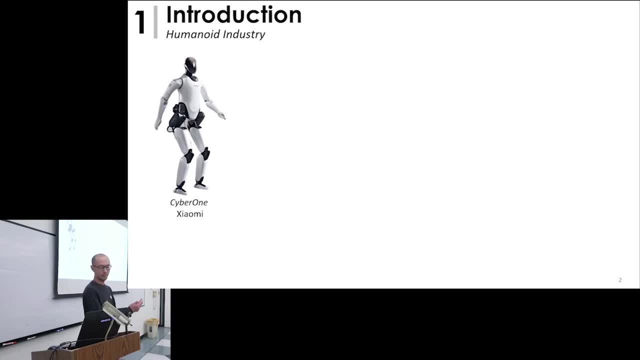 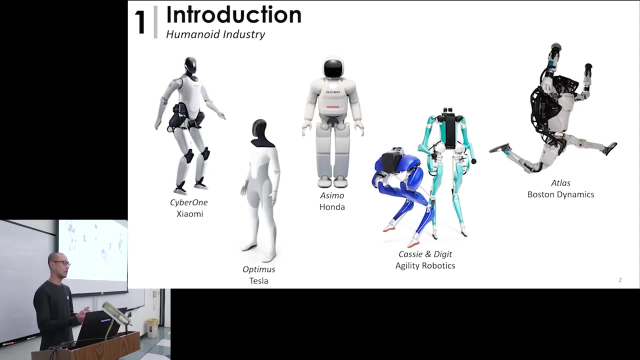 humanoid robot debuted this August in Beijing. Just a month later, Optimus was unveiled at Tesla AI Day. And, of course, there are many, many remarkable humanoid robots that we are already familiar with, For example, Ezmo from Honda, Cassie and Digi from Agility Robotics and, of course, Alice from Boston Dynamics, And more and more. 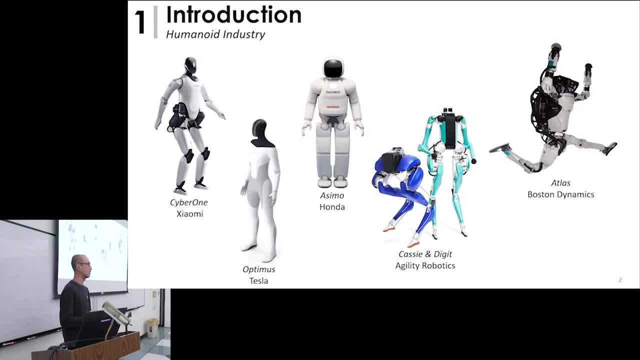 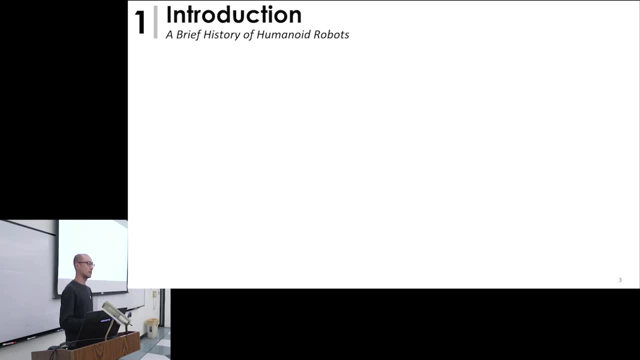 companies have been working on humanoid robots. People are just so crazy about it lately, Yeah, and actually it's not just now. From the dawn of time, humans have been trying to recreate themselves using the technology of the age. The history of humanoid robots can be roughly. 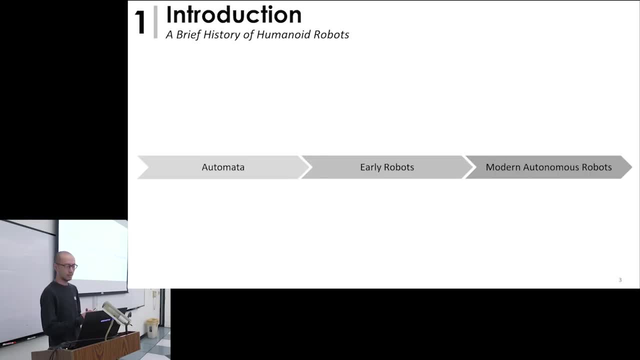 broken down into three phases of Meta, early robots and modern autonomous robots. So first, automata are known as the early ancestors of robots, But technically they are not robots because they are, you know, just mechanical devices, automatically following a sequence of. 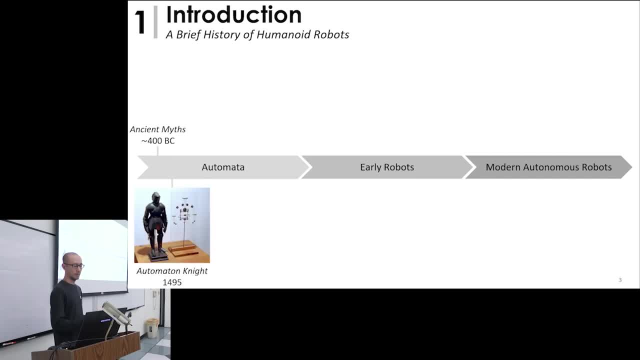 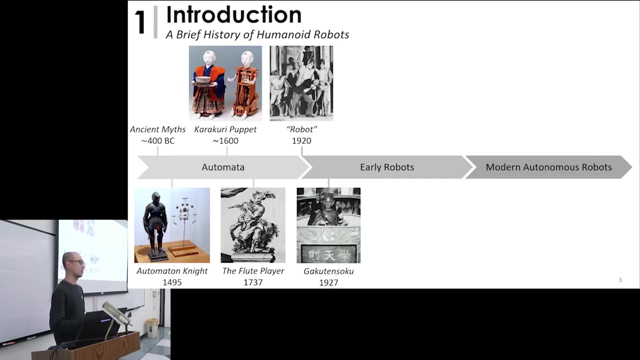 move motions, And there are many good examples, but unfortunately most of them are just sketches or works, And the term robot was first used to denote a fictional humanoid robot in a play in 1920. And the robots in the early hundreds, although they are equipped with more advanced. 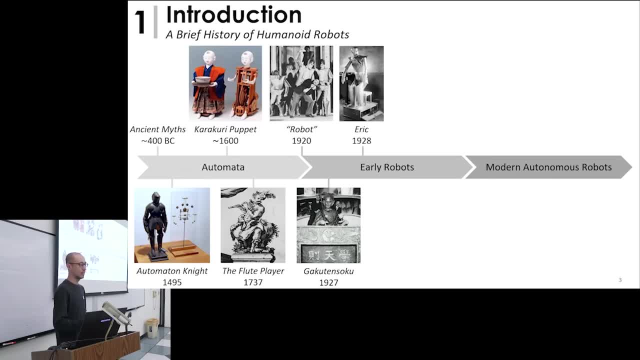 physical structure capable of more dynamic, more complicated behaviors. However, they are considered more as automata because, at its most basic, they lacked a sense of autonomy And the term robotics was not called until the year 1942. And later, in 1954, with the 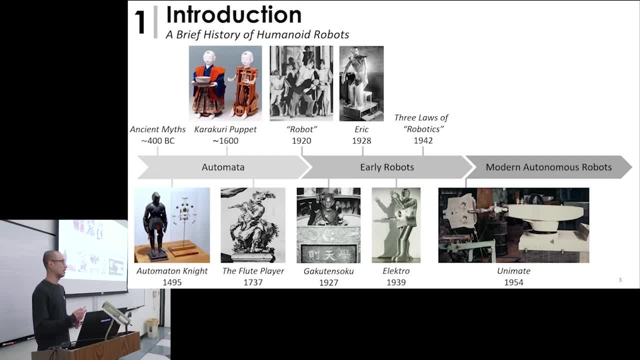 rise of modern computers. the world's first digitally operated and programmable robot, Unimate, was invented in the foundation of modern robotics industry, And later, in 1973, Professor Cato from Waseda University introduced the world's first humanoid robot, WAP01. 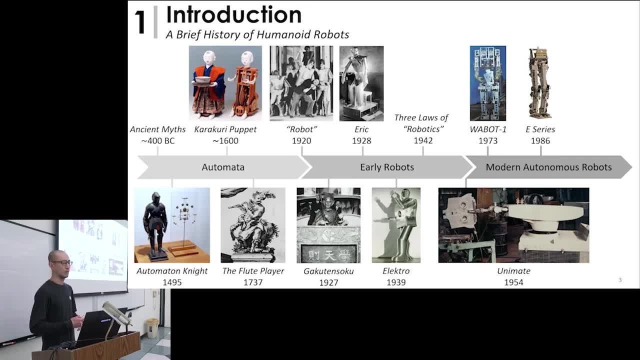 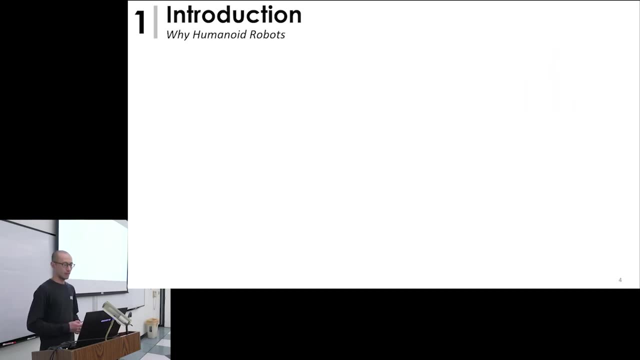 And later, you know, Hongdae just studied their well-known E-theories and then P-theories, which eventually led to the Asimov robot you just saw previously. So that's a brief history of humanoid robots. So why people are so crazy about human robots? 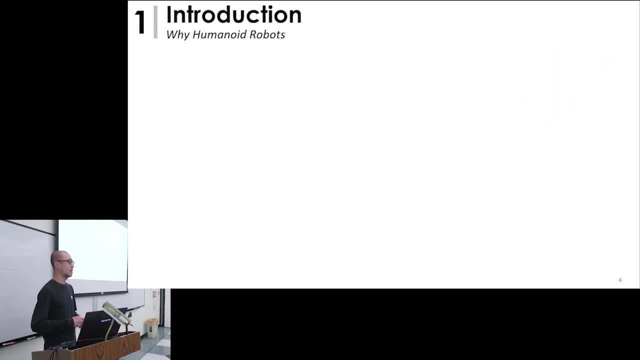 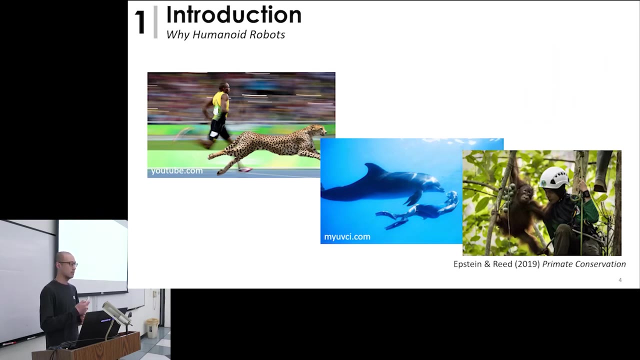 Why the human form right? So what is impressive about humans is their capabilities of navigating the world and manipulating the world around them. People can run, People can swim, People can climb. People can pretty much go anywhere and do anything they want. 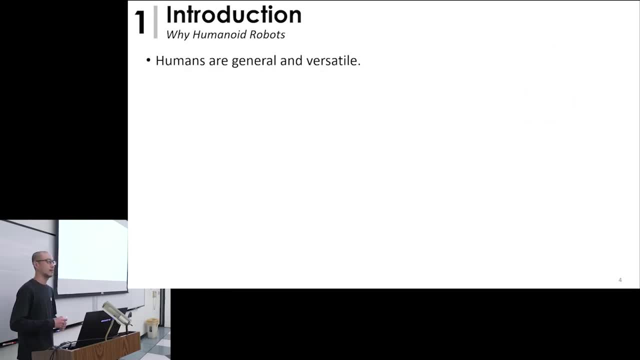 It is this ability that we wish to replicate in machines that someday can potentially overturn our daily lives. And meanwhile, there's no denying that the human world is designed for humans. I mean the door size, the step height and all the tools. 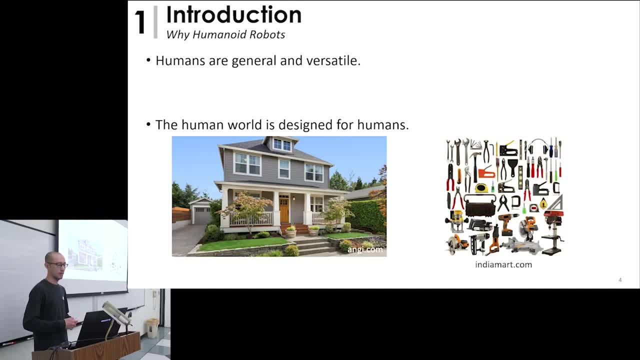 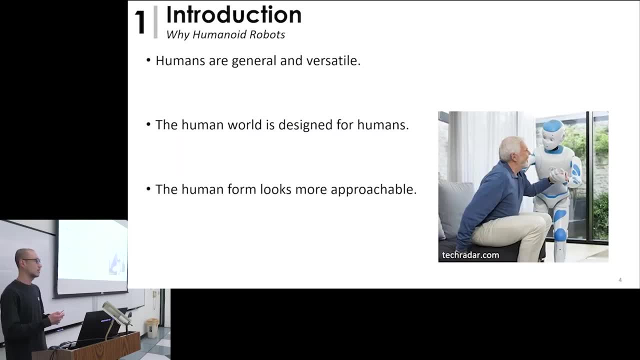 we use right. So if the robot is not of the human form, then we might have to recreate all of this for robot use only, which may take too much effort. And finally, psychologically, the human form also looks more approachable as living and working partners. 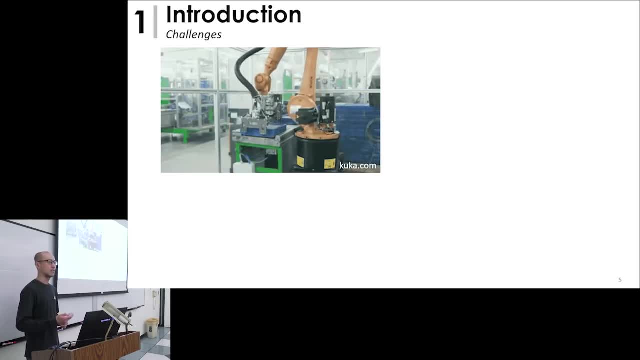 So. for decades we have seen the incredible performance of automation robots in the factories. However, we have yet to see human robots be utilized to aid human in the real world. This is due in part to the fact that the approaches to effectively navigating these two environments are different. 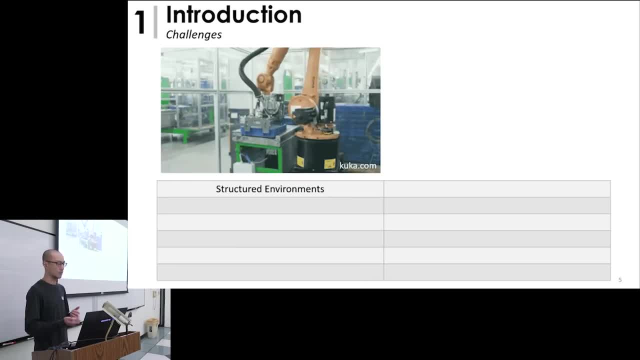 So in the factories, the environments are structured and controlled. The robots are typically fully actuated with a fixed base which grants them full control authority at all times, And the states can be directly measured with high accuracy, And meanwhile interaction with the environment are not required. 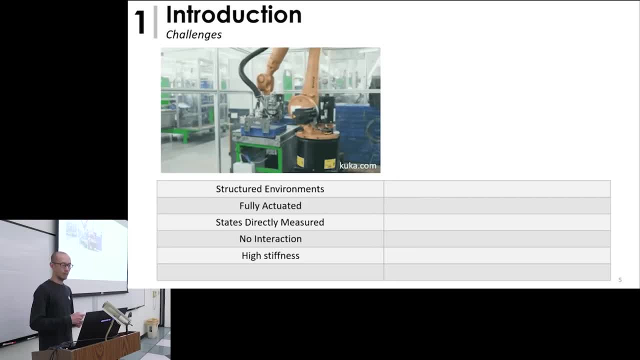 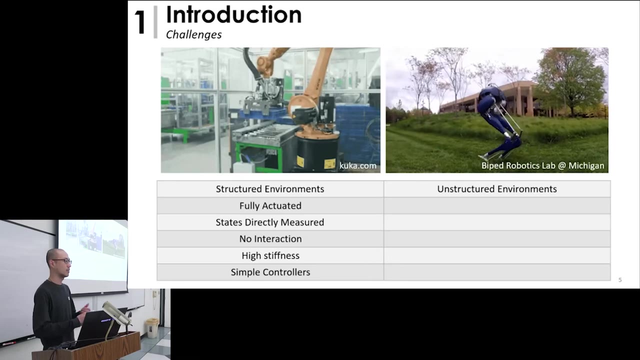 And instead high stiffness, high precision, high strengths are preferred. Under these conditions, simple control strategies can be used. Unfortunately, this is not the case with the robots in the real world, where the environments can be unstructured and can be changing all the time. 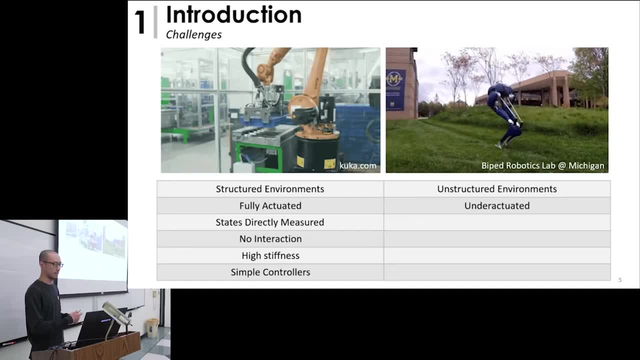 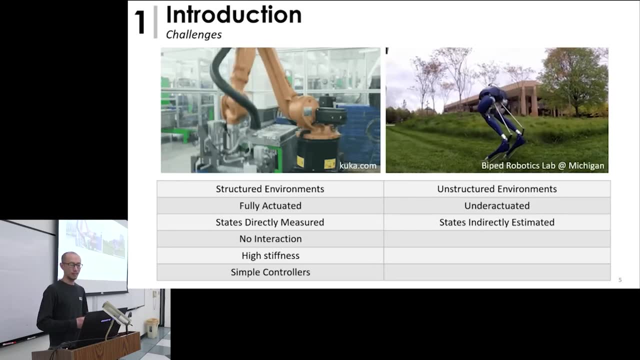 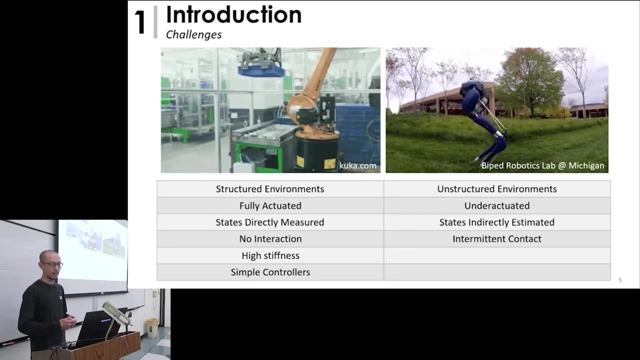 And by removing the fixed contact with the ground the robots can become, the system can become under-actuated And the states can now no longer be directly measured. Instead, sensor fusion, advanced fielding techniques are required, And whenever a robot makes a foot contact, 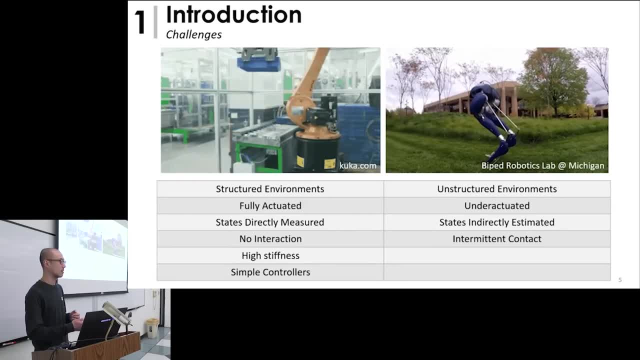 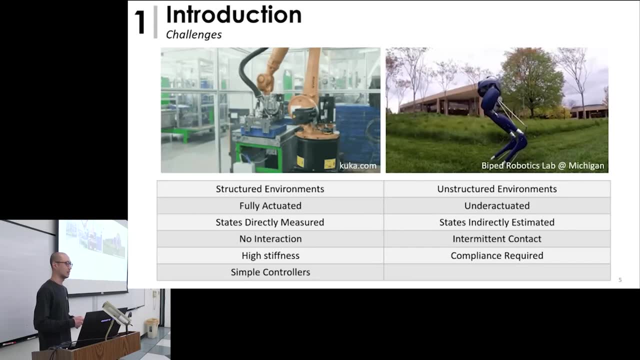 whenever a foot makes contact with the ground, a collision occurs, imparting an impulse to the system, And these collisions need to be carefully, effectively mitigated for the sake of system stability. Under these conditions, more advanced motion planning and control algorithms are required. 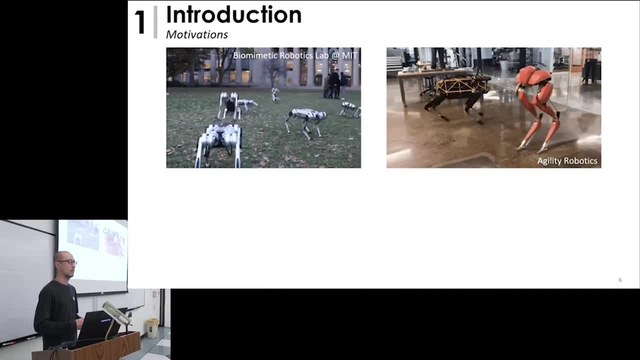 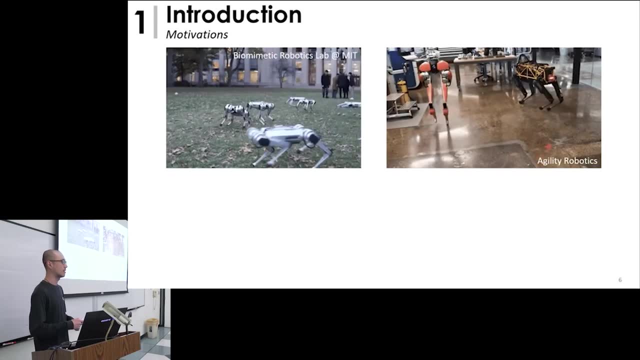 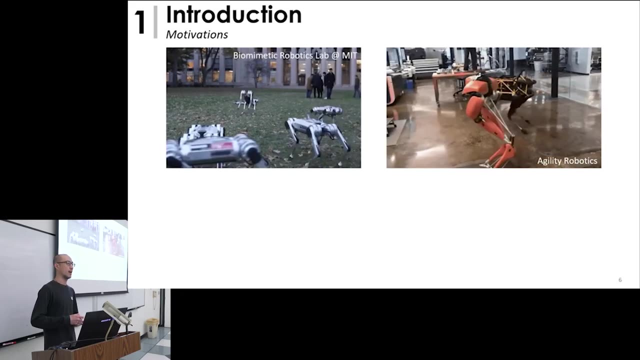 And technically, a quadruped robot faces a similar difficult position. However, recently, significant faster development in quadruped robot has been witnessed. Compared to a quadruped robot, a bipedal robot is more mechanically complex, requiring more powerful actuators, more degrees of freedom. 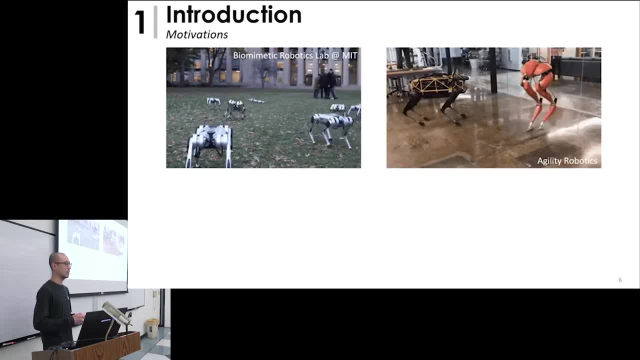 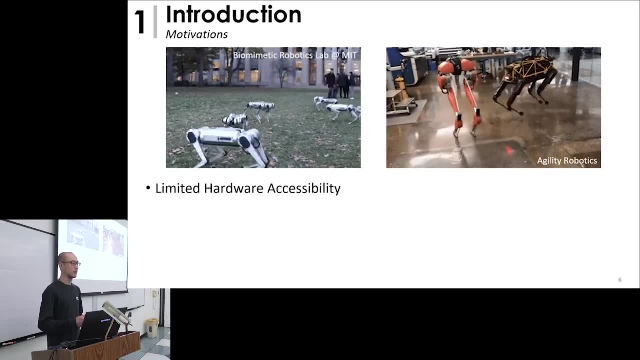 and they are more intrinsically unstable. So this poses two critical challenges in the study of humanoid robots. The first one is accessibility to the hardware. platform is not for the human is limited, as it either takes too much effort to develop a human robot independently or the 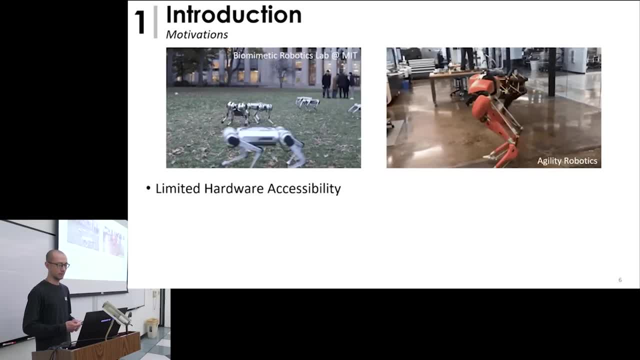 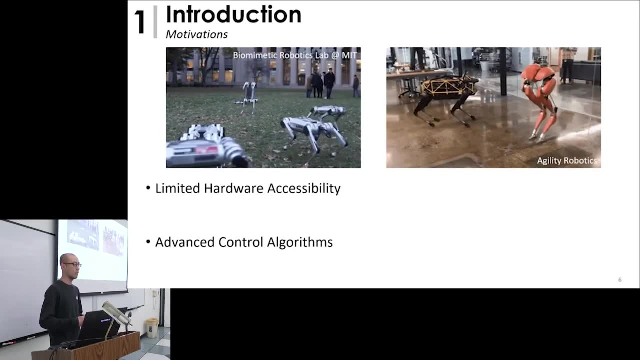 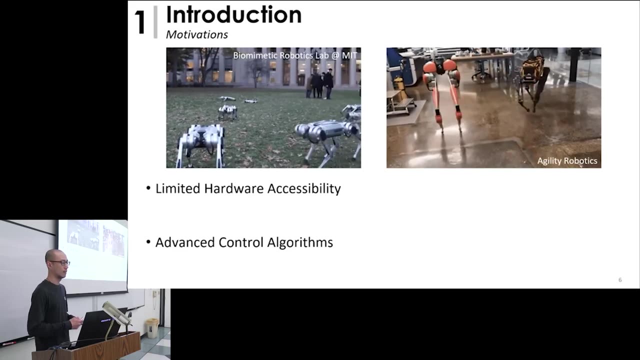 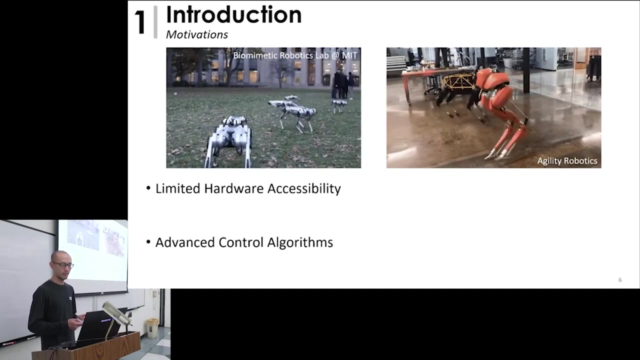 commercially available ones, if any, are too expensive to afford. and second, as a bipolar robots. as the bipolar system is considerable, considerably more challenging than a qualified robot, more advanced, more efficient control algorithms are essential, especially for the locomotion. so this dissertation aims at solving some of the problems in these challenges in 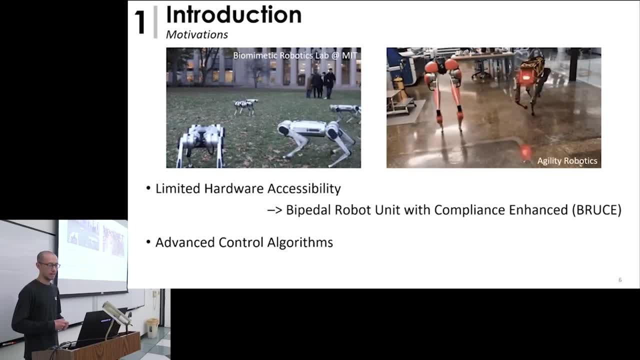 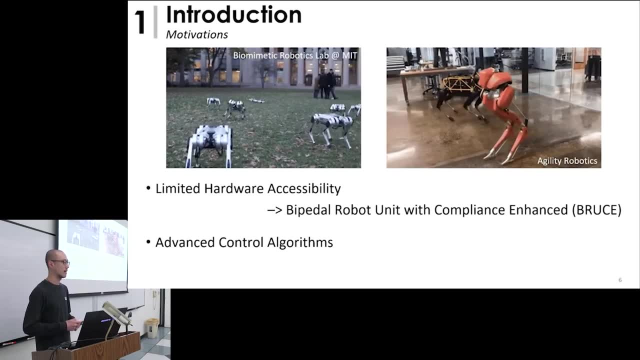 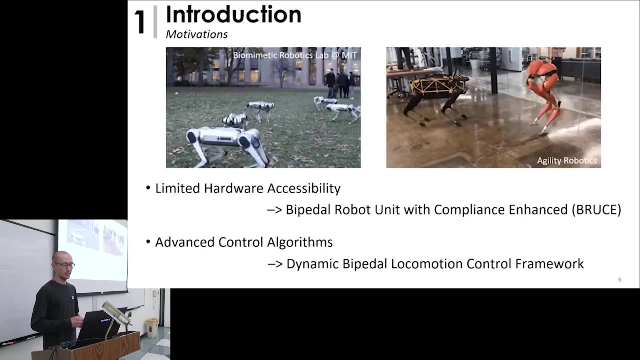 particular: first, a miniature bipedal robot capable of dynamic behaviors is being under development. the robot is named bruce bipedal robot unit with compliance enhanced. it is expected to be an open source platform for the robotic community in the near future. and second, a state-of-the-art dynamic bipolar locomotion control framework is being studied. 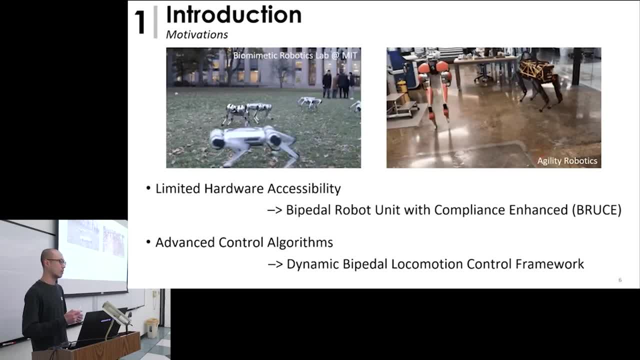 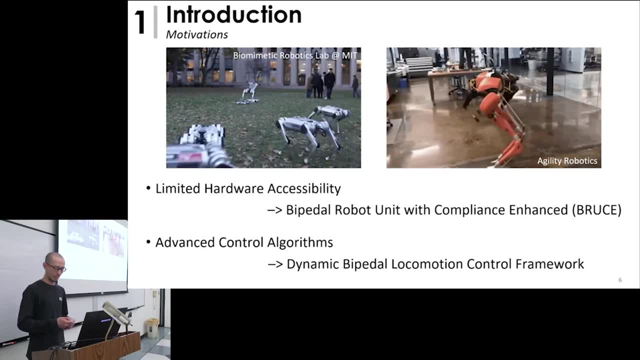 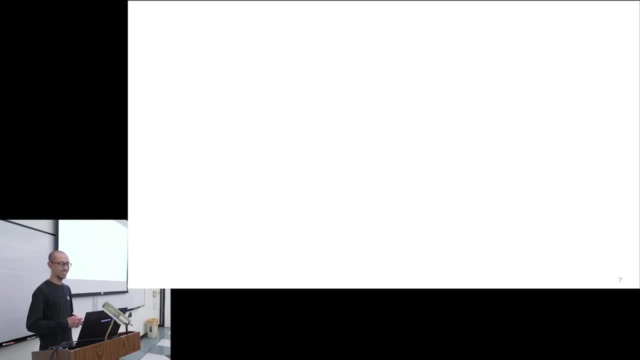 the framework is general and versatile as it intends to achieve a strong robustness of stabilizing a wide range of bipolar locomotion gates, including walking, running and hopping. okay, so let's take a look at the overview of this, of this dissertation. so first we have our 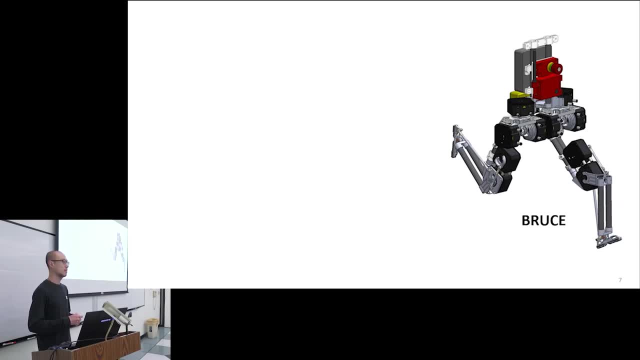 robot bruce. bruce is of 0.6 meters height, adapting an average human body propulsion. it has a total and two, five degrees of freedan legs. each leg of blue, each leg of bruce, has a spherical hip joint, a single knee joint and a single acorn joint. 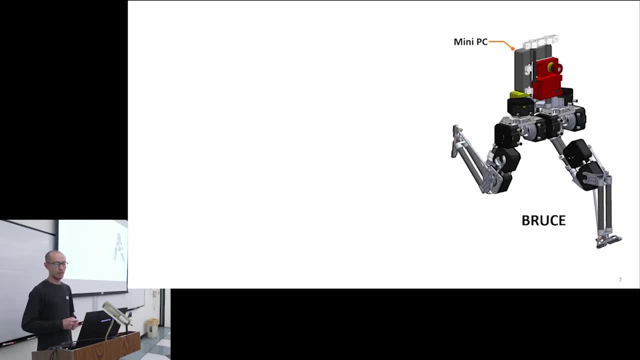 it also has a line contact with the ground. the bruce robot is fully actuated, controlled by a mini pc, powered by the lipo battery and equipped with a wireless e-stop, you know, to cut the power in emergencies, to have better top transparency and compliance to the unknown environment. 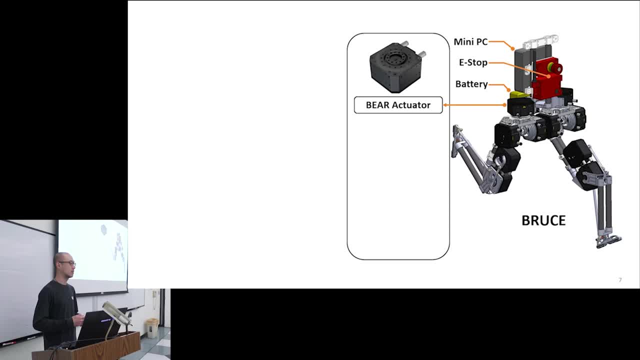 progressive actuation are equipped using the deactuator developed in our robot robot robot unit in our lab. The actuators are essentially high torque density brushless DC motors due to a large gap radius and therefore only a small amount of gearing is needed. It also equates with joint encoders. 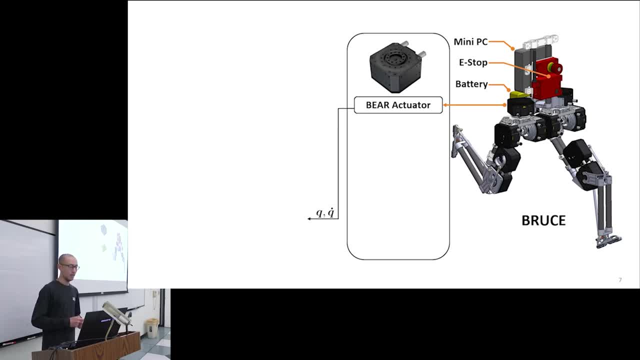 for joint position and velocity feedback. An inertia measurement unit is mounted on the torso for acceleration and angular rate measurement. For Bruce being able to detect when the contact between the ground and the field is created or not, a sensing fluid is designed based on the working principle of electronic switches. 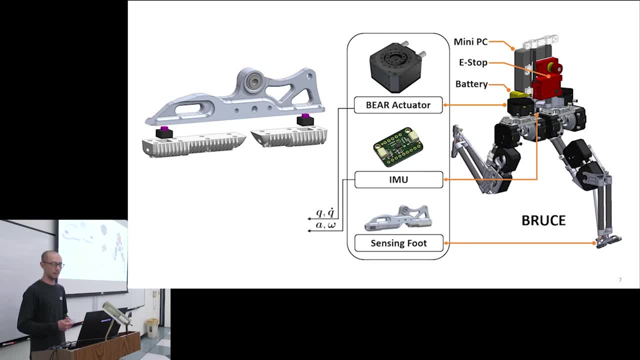 which is directly inverted into the robot contact layer. All the sensory information is fused into the state's animation And based on that we can derive the kinematic and dynamic model to get all the robot states ready for feedback control And, on the other hand, based on the user command. 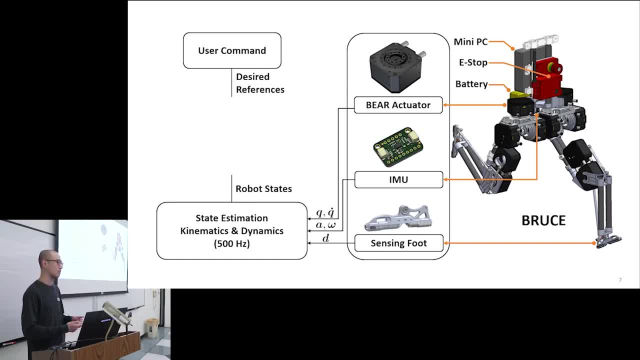 we can generate the reference for our controller, For example the working speed, the working velocity and the working speed, the working direction And the locomotion control is divided into two layers, where the high level plans the footstep, while the low level controls the whole body motion. 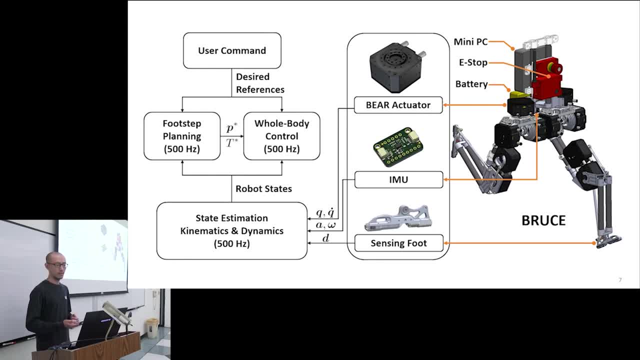 while establishing the full contact as planned And eventually the joint torque command is sent to the actuator to close the loop. Okay so we will have time to go over each component and let's start with the Bruce robot design. Okay, so conventional humanoid robot, usually, usually. 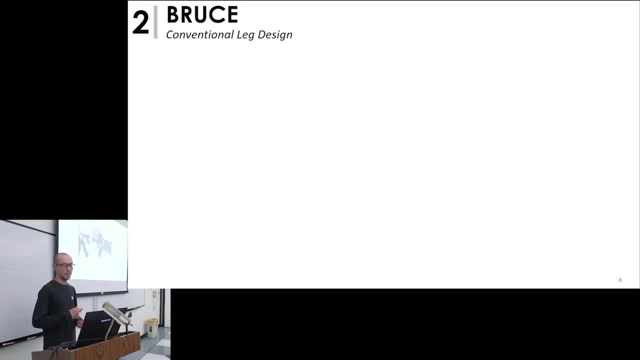 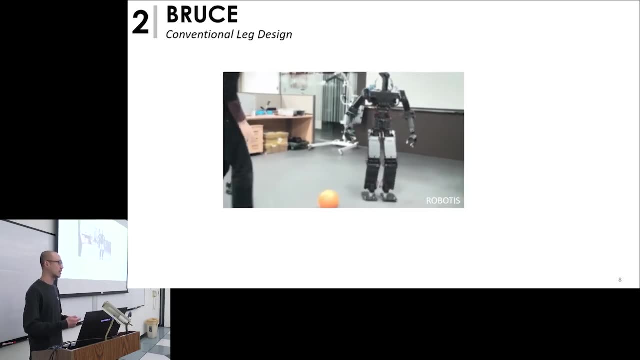 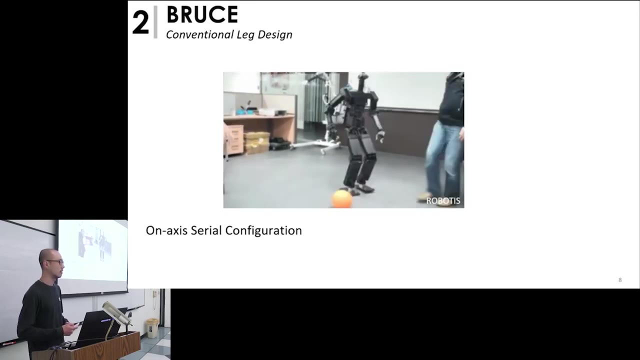 Okay, so conventional humanoid robot usually usually have very bucky legs with a minimum of six degrees of freedom in order to in order to achieve any arbitrary foot position and orientation in 3D, And these robots typically have rotary joints with several motors in a serial configuration. 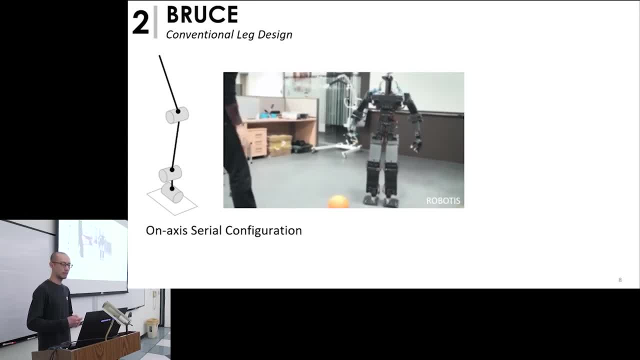 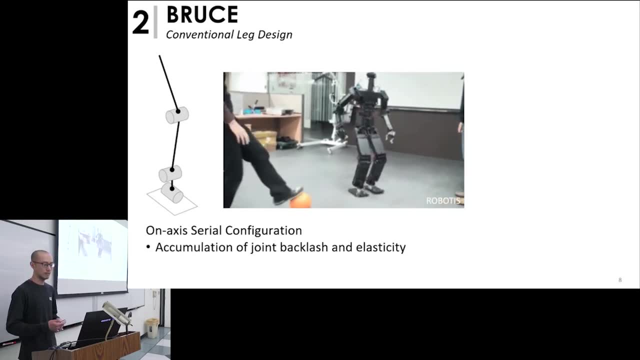 That is, the actuators are directly located at each joint And it's strength lies in, you know, the simplified structure and analysis. However, it comes at the drawback of limited capabilities, For example, accumulation of backlash and elasticity from each joint to the end. 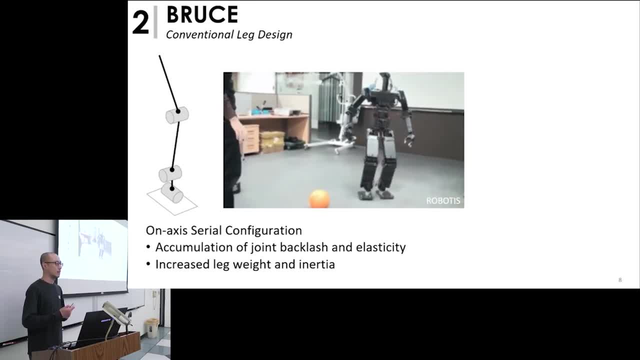 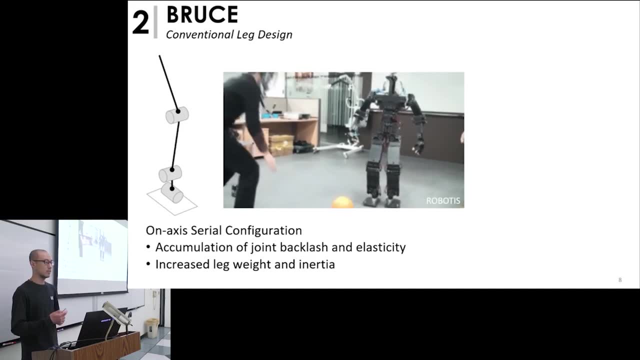 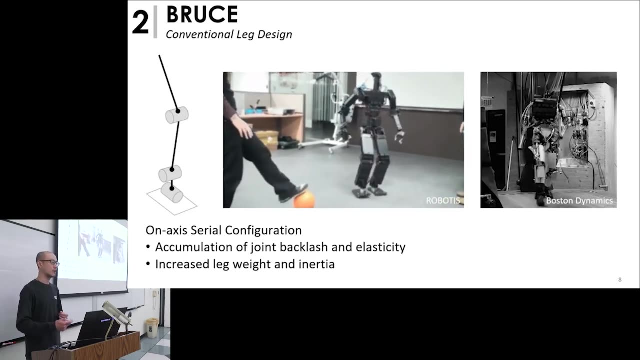 and, more importantly, increased leg weight and inertia. The effects of reduced joint rigidity and increased leg weight and inertia can be substantial when it comes to dynamic leg motion. However, at the time it was not necessarily appreciated, because the robots move so slow. 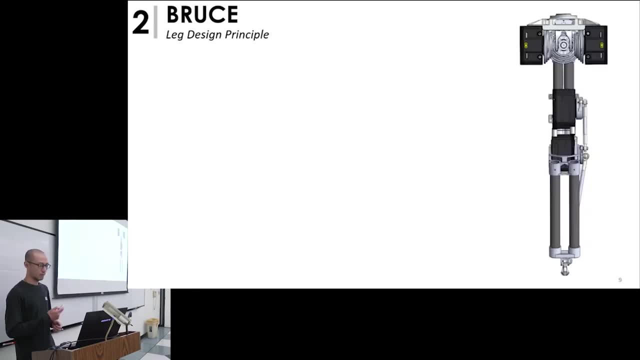 that the dynamic effect can be fairly neglected. So nowadays the popular trend on humanoid uh design is using lightweight leg with small foot, Okay um- which can lower the inertia and in the process, uh reduce the control effort. There are many different approaches. 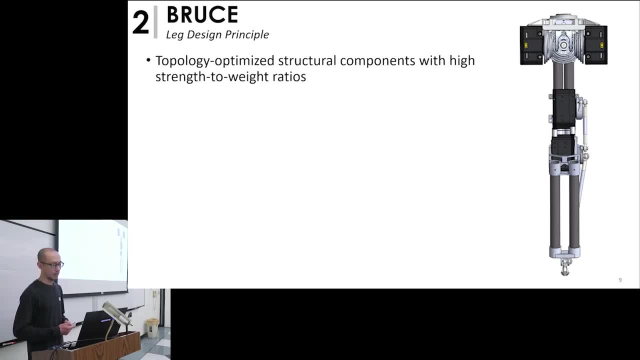 to achieve this paradigm in practice. For example, uh topology, optimized structure components with high strength to weight ratio. That is suppose we have a part like this at the beginning. Uh, we can have some. we can do finite element analysis and based on the simulation result, we can just remove the strength. 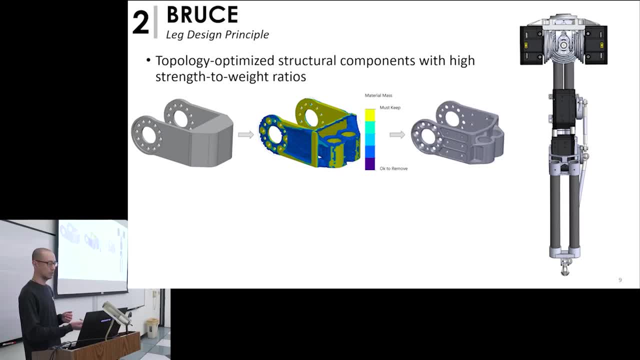 Uh, we can do finite element analysis. We can just remove the structure that is necessary to reduce the weight. And of course, we can try, uh try, to use strong and light materials, for example carbon fiber and titanium, And, of course, the most prevalent option. 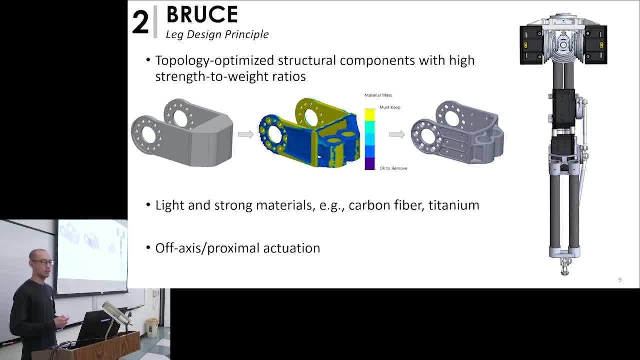 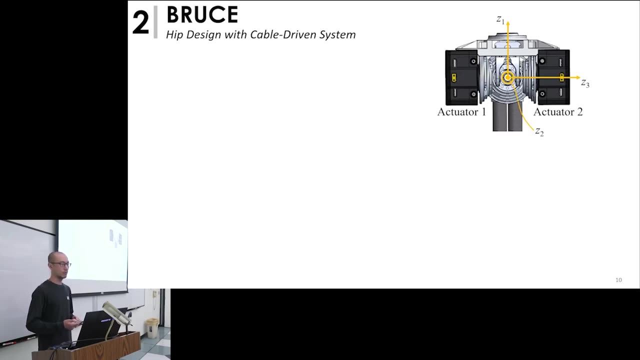 is to place the actuator off axis as close to the torso as possible, And which also uh. this can also lead to some interesting uh joint design where parallel mechanisms can be involved, For example um a two degree of freedom cable driven pulley system. 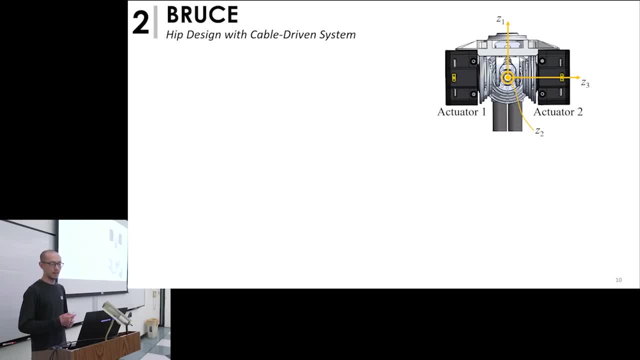 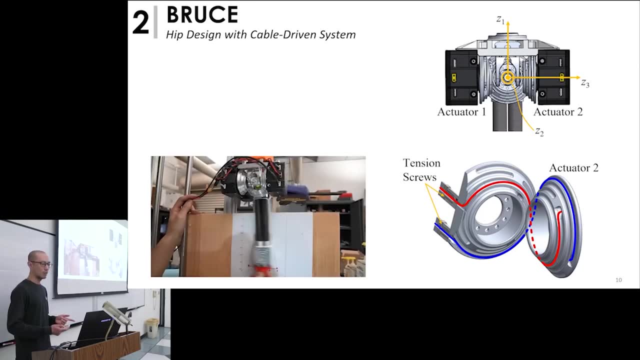 is applied to the hip pitch and roll motions. Uh, the parallel configuration leads to the coupling of the two actuators, So when they are moving in the opposite direction we can have the roll motion, When they are moving in the same direction. 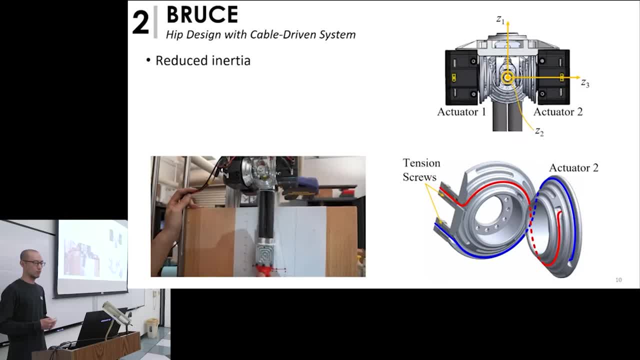 we can have the pitch motion The scheme leads to. uh can reduce the inertia of the female link. It also expends high stiffness as as the uh, due to the mechanical power. uh coupling of the two actuators. 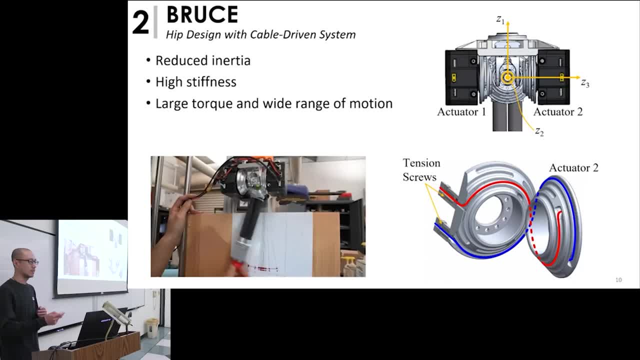 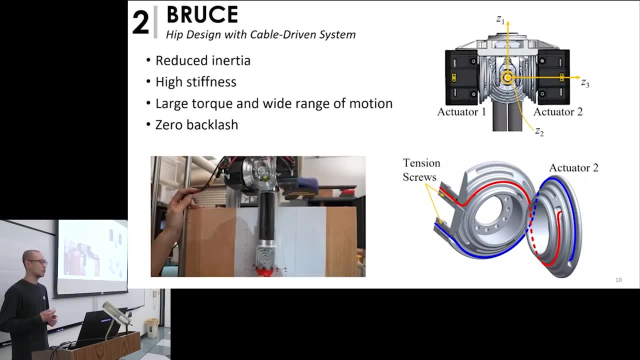 It also can produce large torque because the two actuators are essentially powering the same joint. It also comes with a wide range of motion. And finally, cable driven system is well known for its uh zero backlash feature, Because previously we are using a bevel gear. 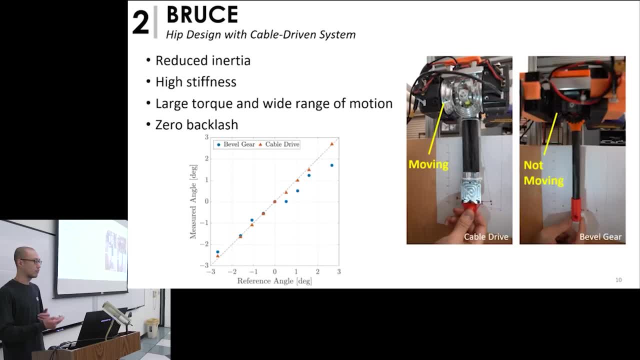 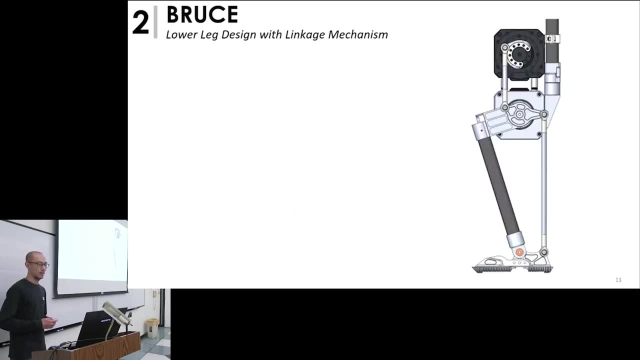 to achieve a similar configuration. However, as you can see, the joint performance, the joint accuracy is very bad. The proximal uh actuation principle is also applied to the lower leg design, So the knee actuators is at the knee joint. 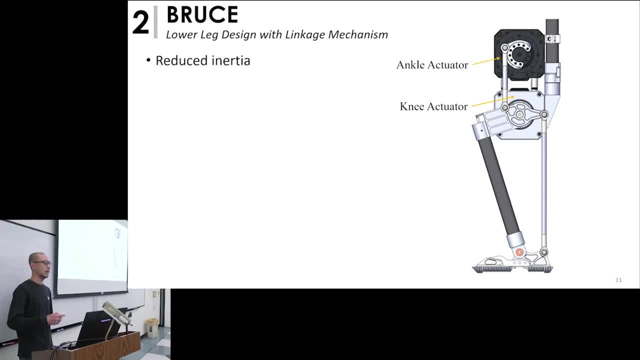 which is fine. However, for the ankle actuators, instead of placing at the ankle, which is uh way too distal, we relocated to the female link to reduce the inertia. As a result, two pairs of four bar linkage mechanisms are applied, uh to deliver torque to the ankle. 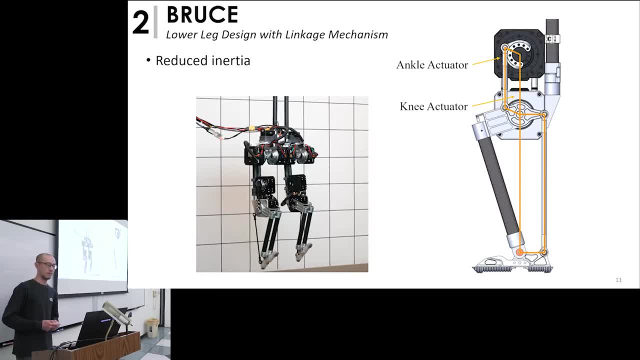 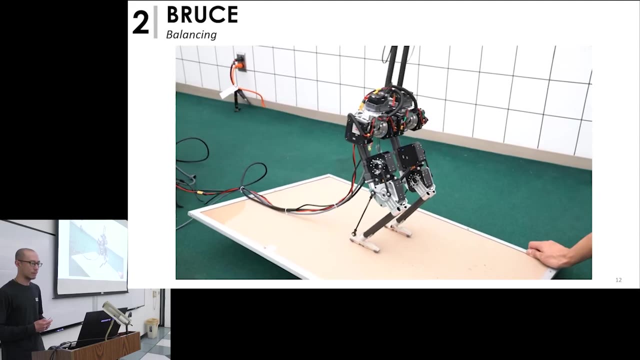 Uh, both of parallel ground shape with a one-to-one transmission ratio. So, uh, that's just some design highlight of Bruce. And once we have the robot, we just play with it. We test its basic functionalities. For example, this is CISO balancing. 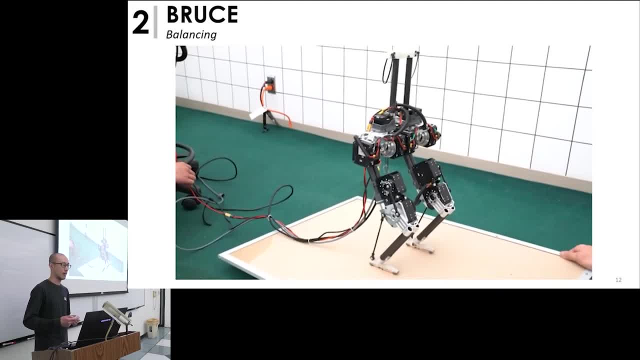 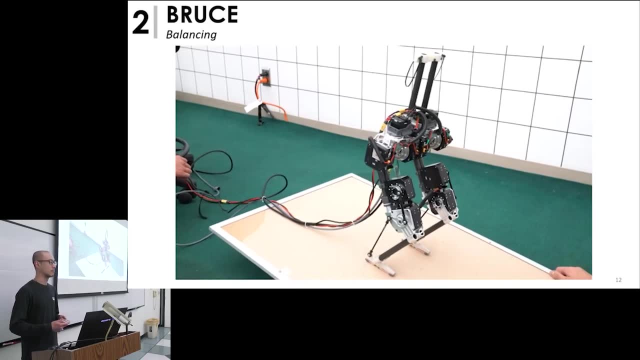 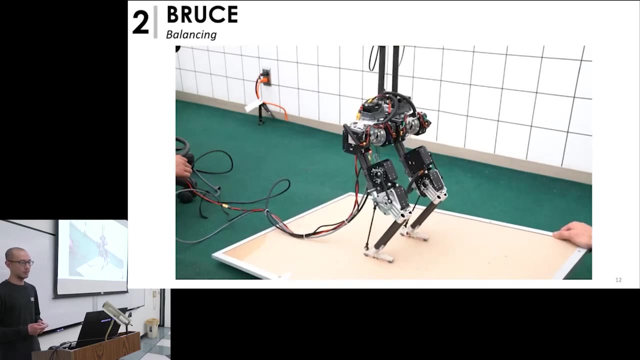 where we use an inertia measurement. uh, use an IMU to estimate the ground orientation And uh, Bruce can keep his torso in the upright configuration. based on the kinematic model, And to verify dynamic capability of the robot, a vertical jumping test was conducted. 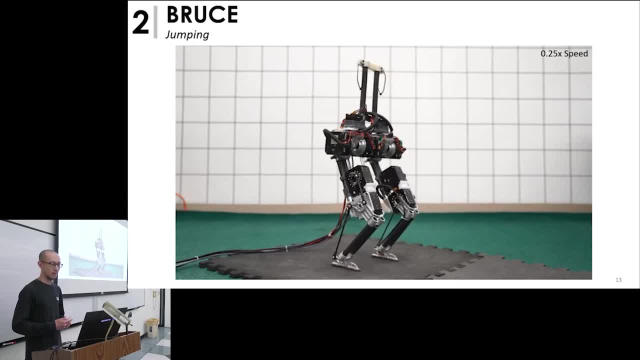 and at that time, the, the trajectory, are only hand design. So, uh, it might not even be dynamically consistent, but Bruce was still able to jump, and it was, uh, almost a year ago And just recently Bruce can already perform jumping. 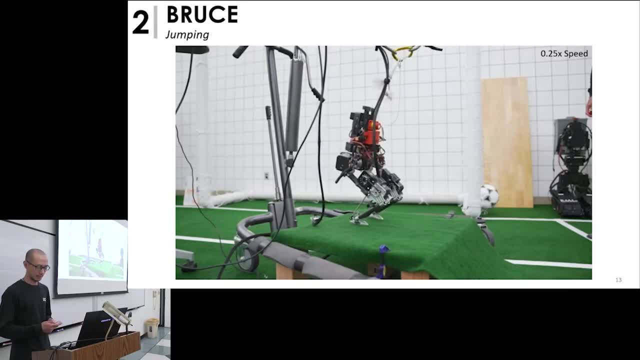 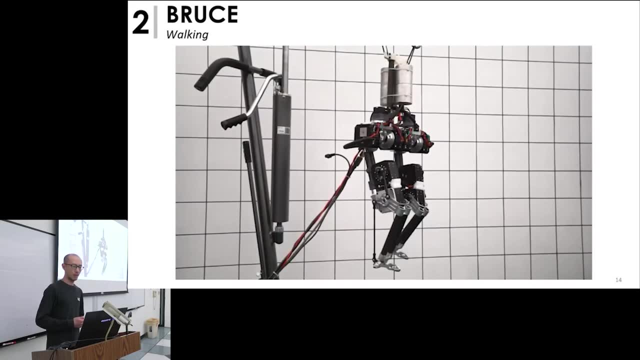 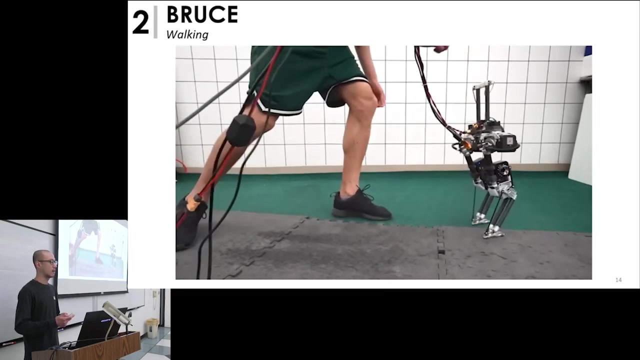 with an optimized trajectory- Just the showcase of the dynamic capability of the robot. and of course we also do a preliminary working test where the trajectories are designed to be both chemically and dynamically consistent, and with an open loop trajectory, Bruce was able to work a considerable amount of distance. 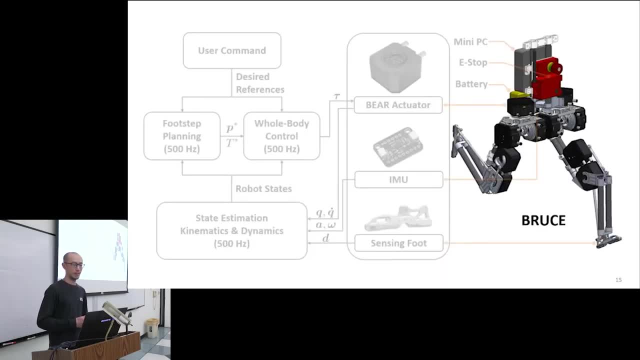 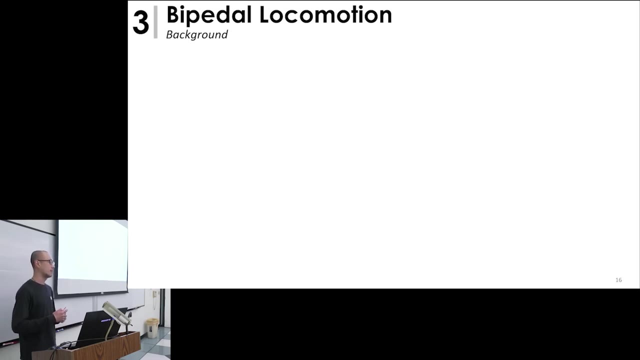 okay, so that's pretty much about our robot Bruce, and now let's shift our focus to the problem of bipolar locomotion, and we will start with some background. Bipolar locomotion has been, you know, studied for decades and yet it remains an active research field. The first control paradigm, using the notion 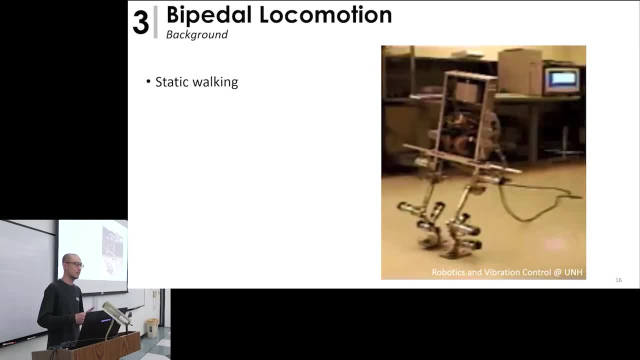 of static walking. that is, the center of pressure, a center of mass of the robot projection on the ground is always contained within the support polygon of the robot. The robot will not fall down if the motion is suddenly stopped. and ever since bipolar locomotion has become more. 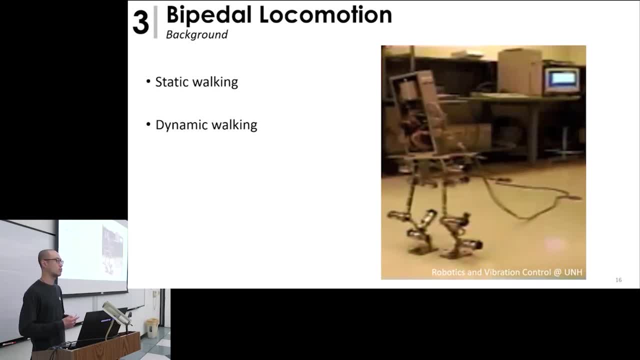 and more dynamic and natural. this is due to the continued progress in three key aspects: the mathematical understanding of bipolar locomotion, the computational ability to encode this mathematics and, of course, the hardware capable of realizing this understanding in practice. we have just talked about the hardware perspective. now let's talk about the 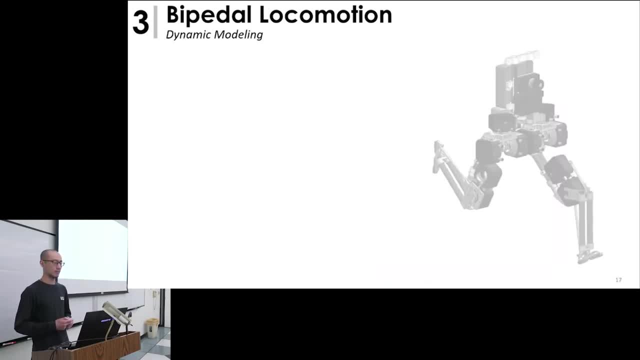 mathematical modeling of bipolar robots. Bipolar robots can be considered as a tree of a tree of rigid body, one of which can serve as the base link, typically the torso, you know, because interaction with the, with the interaction with ground, is always changing during locomotion. so one 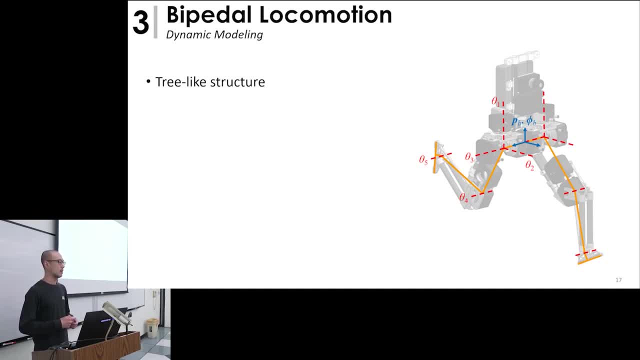 convenient way to model the system is to construct a general representation of the robot floating in the air and then in for strong contacts at the stance feet. this is typically known as the floating base model, where the configuration space is the position and orientation of the floating affluent base joint, as well as the joint angle. 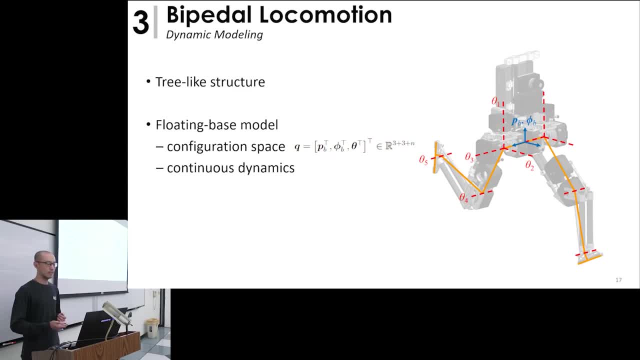 dictating the shape of the robot. the continuous dynamics can be written in the Lagrangian form, where H is the inertia matrix, C is the Coriolis and centrifugal terms, G is the gravity, the constant. matrix B defines how to control the joint torques and to the model, and the J and F are respectively the foot. 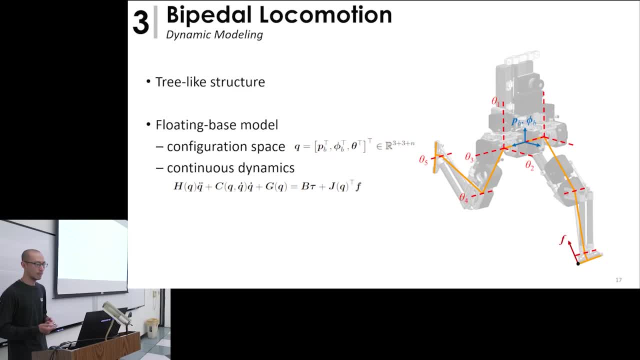 contact Jacobian and the contact force at the contact location. and whenever a foot is making a contact with the ground, it's assumed to be stationary and differentiating much more. yes, the axillary constraint on the robot and meanwhile the contact force can not be arbitrary right at first. it is unilateral. 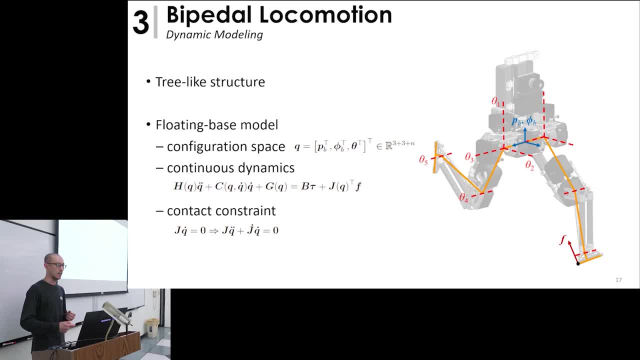 meaning it can only push the ground, not pull the ground. and second, it also needs to respect the current friction. so in the end the feasible work space of the contact force can be represented by some cone shape. so the resulting dynamics is also called the full order dynamic model of the robot, because it actually 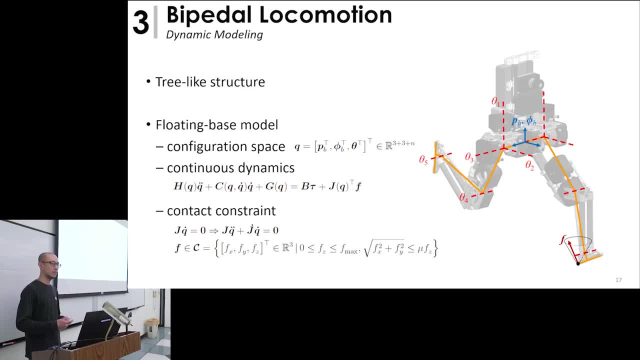 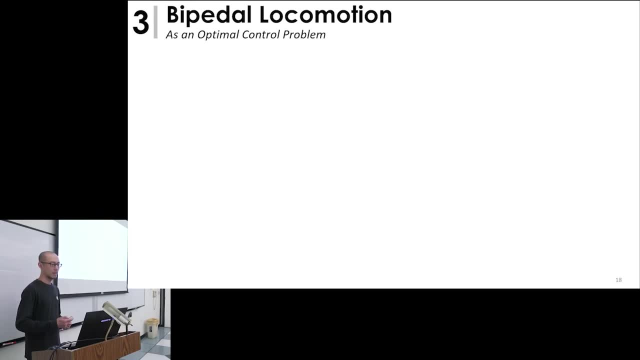 consider every single detail. it is highly nonlinear, high dimensional, time varying, multi-input, multi-output, strongly restricted. it's really a mess. so, due to the incorrect complexity, we can't actually consider the contact force in this example. so the main challenge we find is that we can't really 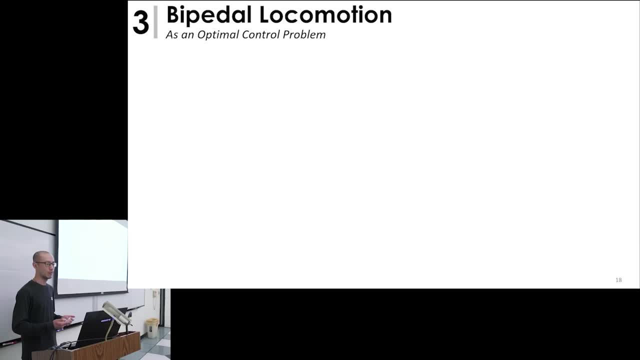 measure and know the fine-grain formation of the main structure of the robot, in order to be able to process all the phenomena that we can see now using a mathematical optimization. we can actually learn a lot from this example. because of the overall function of the optimization, we need to have the 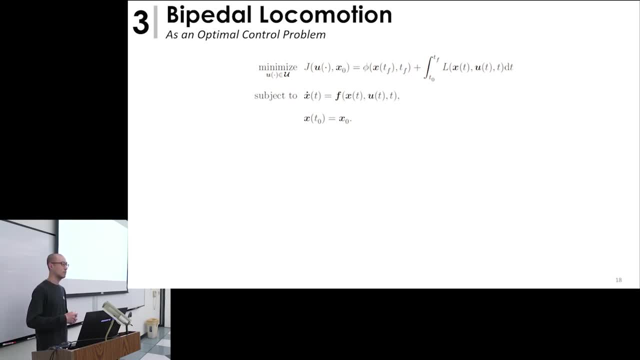 same log of the control that we need to be able to measure it. we actually need to be able to measure the form of the control of the robot so we can get the And because it's not possible to generate the analytical solution for any general nonlinear system. therefore, the technique of trajectory optimization is widely adopted as a numerical 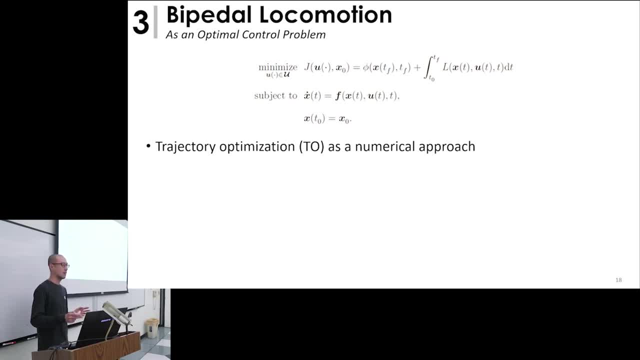 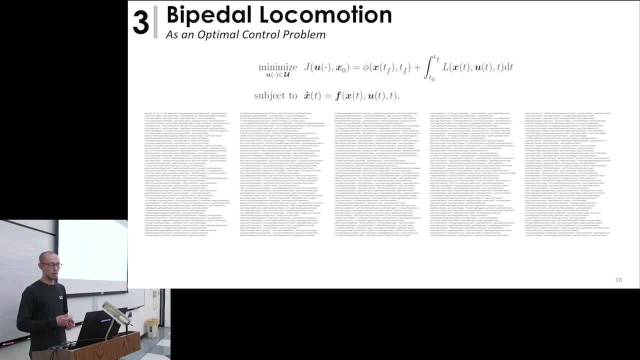 approach which computes an open-loop trajectory instead of trying to find an optimal control role for the entire space-space. However, trajectory optimization of bipedal locomotion in its most complete form is still extremely challenging, even offline. So we once tried to derive the dynamics. for a simpler robot like this. however, the dynamic 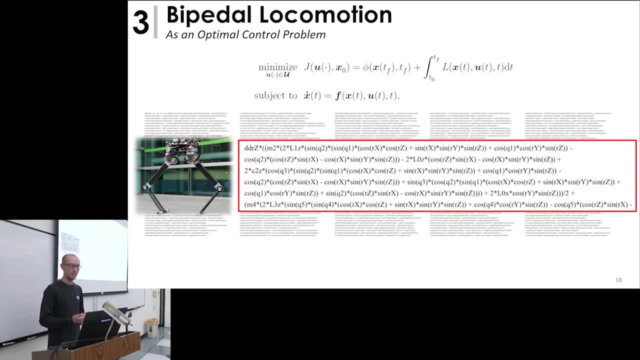 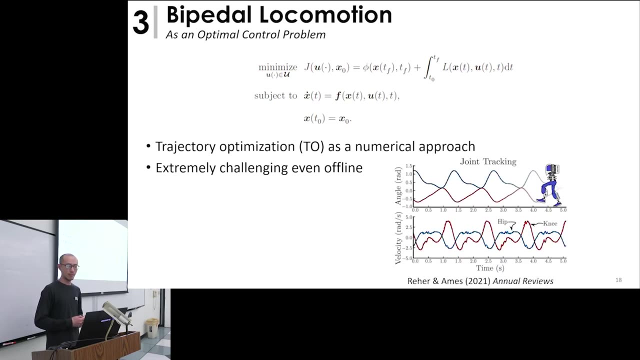 equation is already hundreds of pages. It's really really insane. So due to limited computing power of the early devices, this approach was still stuck with simple planar model by the end of 1990s. It was not until the year of 2000 that the optimal working motion of a complete 3D robot 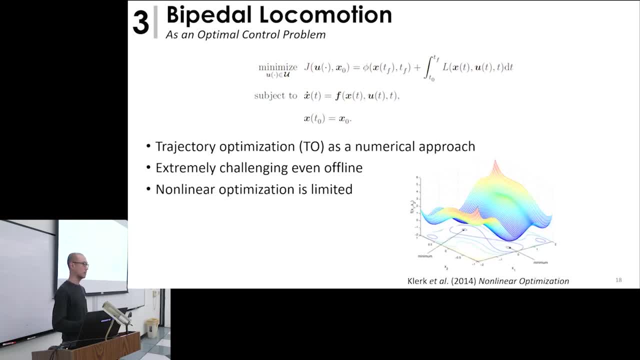 can be solved. However, the curse of nonlinear optimization still limits its performance. So, first, the solution is highly sensitive to the initial gas- A very bad initial gas can easily cause the problem infeasible- And second, even if the problem is feasible, often at best a locally optimal solution is. 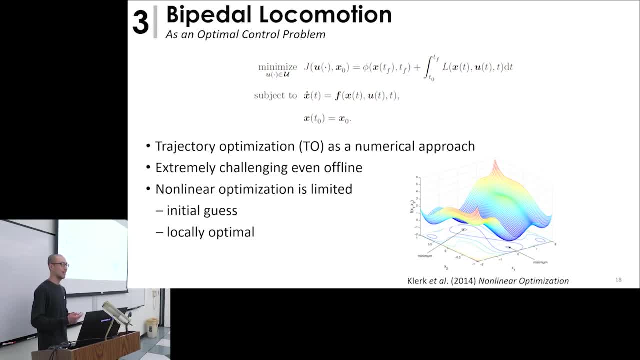 provided. So not being able to generate the gate online efficiently limits the robot to a predefined set of pre-computed actions, potentially ruining its reactivity in the presence of even small perturbation. So one way to alleviate this serious limitation is to generate a database of trajectories. 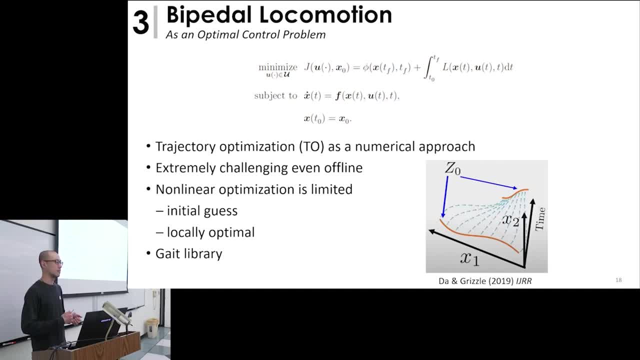 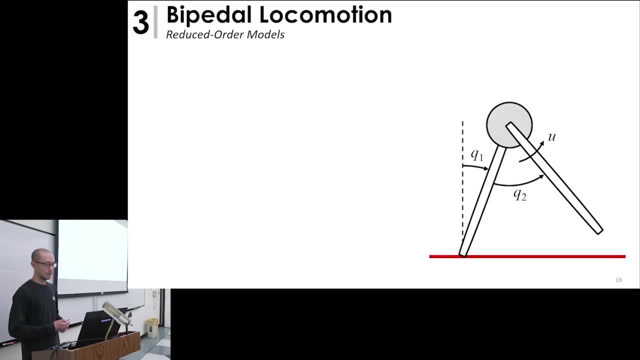 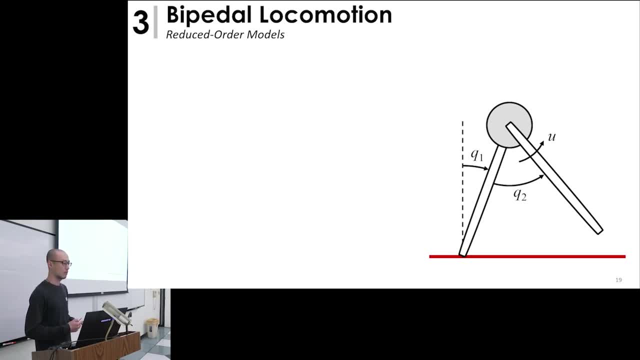 Thank you, Thank you, Thank you. Yeah, Thank you. So, to ease the computational burden of 4-order approach, another branch of bipolar locomotion is using simplified or the Reduced-Order Model, which only focuses on the most saving aspects of the system — for example, the center of mass of the robot, as well as the 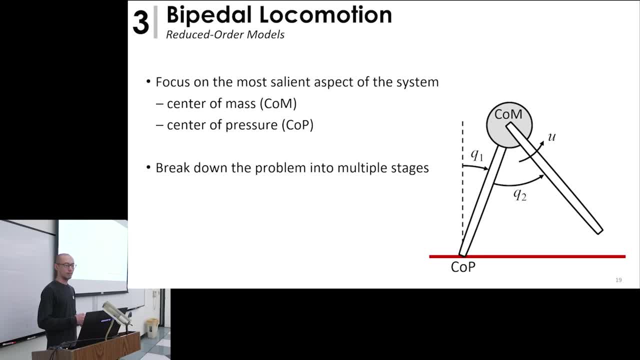 center of pressure on the foot — without you know, considering the complicated joint dynamics stage, as it does not consider every single detail during the planning. and a practical paradigm is to have two layers, where the high level plans the footsteps and the low level controls the whole body motion, while establishing the 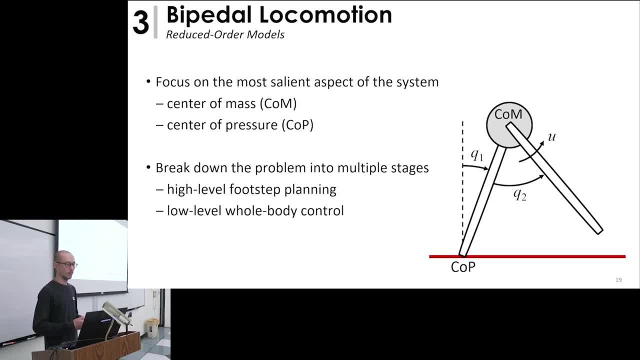 foot contact as planned, and in this presentation we're gonna use the reduce order approach because the derivation is neat, which can have analytical solution and therefore it's computationally efficient, which can be performed online, able to mitigate issue related to reactivity. the disadvantage is that by 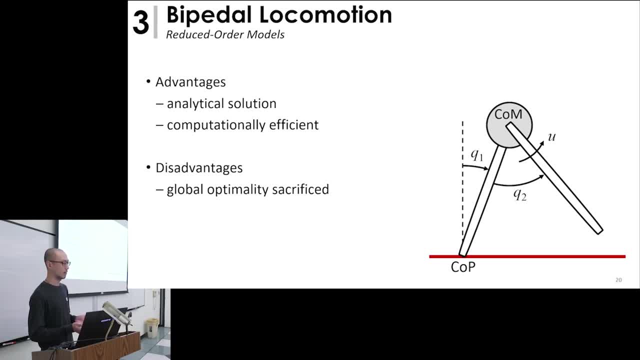 breaking down the problem to several stages, the global optimality is sacrificed and, in addition, it is not guaranteed that any reduced order plan can be feasible to execute on the forward dynamics. this is because it can happen that the robot operating condition can break assumptions of the reduced order model, as we will see in a second, but often, but often, it. 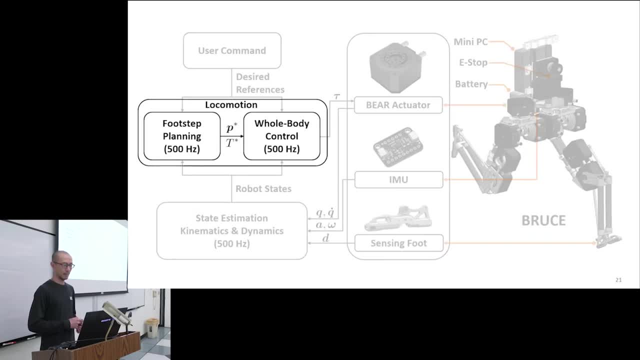 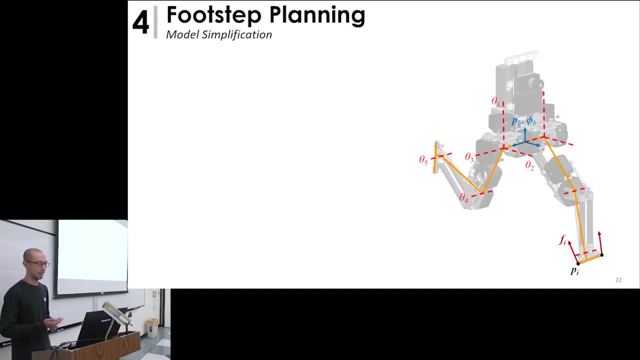 works pretty well in practice. okay, now let's see how we can actually tackle this problem. we start with the first step: planner. okay, so, as I mentioned, we're going to use the reduced order model. okay, so how do we go about, you know, deriving a reduced dynamic model of a bipedal system like this. so one way to 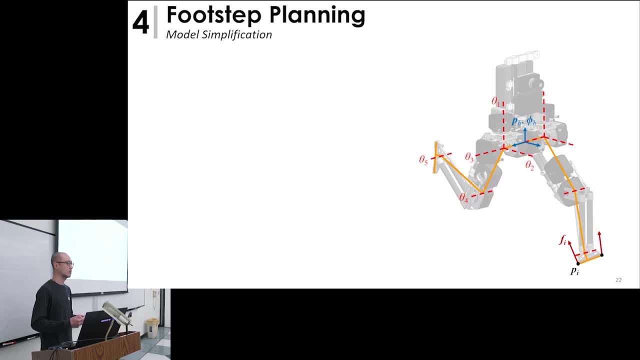 do is to think of a chain of reasonable physical assumption. one thing people typically do to start is say I don't want to worry about the torque saturations. okay, this is actually a not bad assumption, because beer actuators are quite powerful for a miniature bipedal robot like Bruce. and what we and 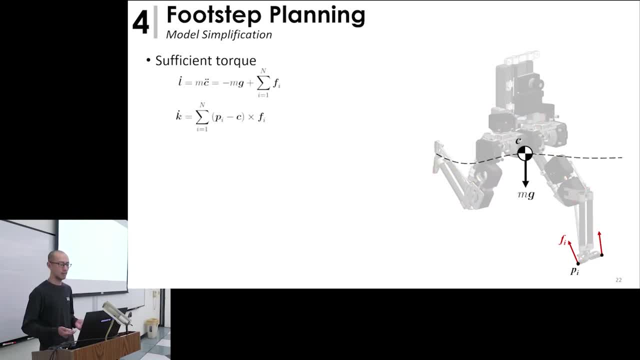 what happens then is you already have a significant simplification of dynamics. now we are not writing down the equation in the complicated 16 generalized coordinates. we can just write down the equation in the complicated 16 generalized coordinates. we can just write down the equation in the complicated 16 generalized coordinates. we can. 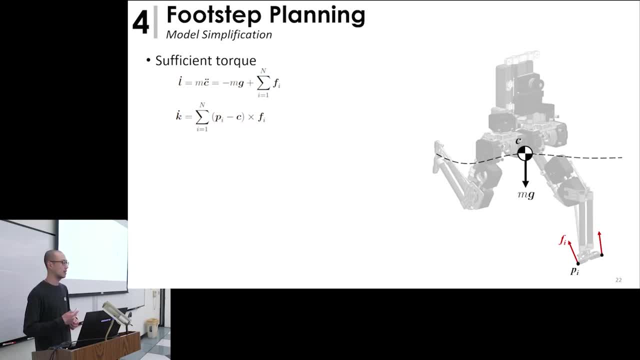 reason about the net external range acting on the system correspond to the rates of change of linear and angular momentum and the so-called centroidal dynamic model. we can go further and say that if the contact of the system is sort of locally planar, then we don't have to worry about some set of ground. 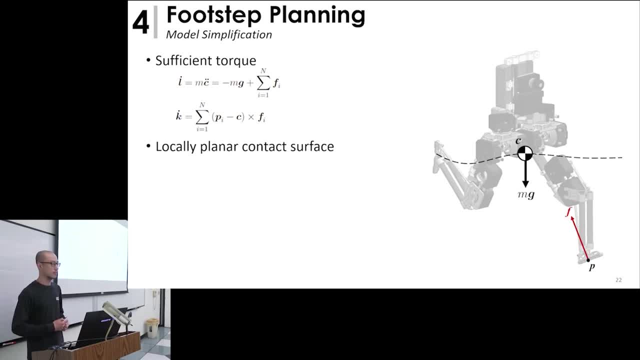 reaction force. we can just focus on the center pressure, just sort of a weighted average, and ground reaction force, on that form and the net ground reaction force as a point, and we can say further that the angular momentum of the system is is negligible, as small, which is often the case and verified by 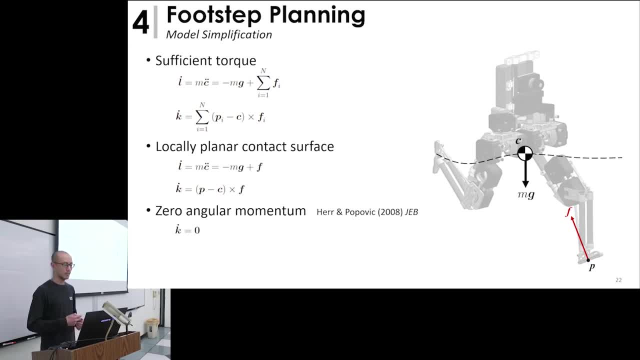 some biomechanics study, then we simply have this term equal to zero, and what we get back is the ground reaction force has to be pointing towards the center mass, and it would be in this form: okay, and here Omega is. just some parameter needs to be determined. 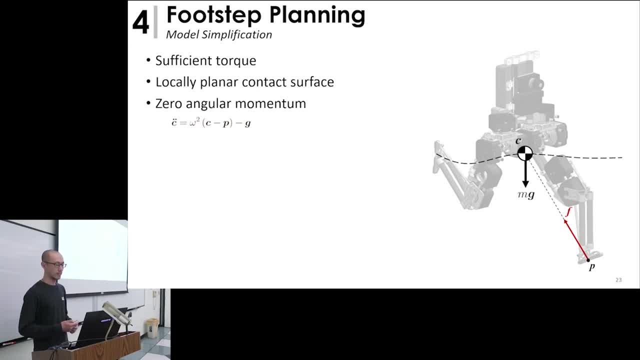 we can make one more assumption that you know. you know we know something about the center of mass height. either is you know, following some nominal trajectory or it's simply constant on the flag wall. then we can solve this Omega value okay. so the resulting dynamics is called the linear inverted. 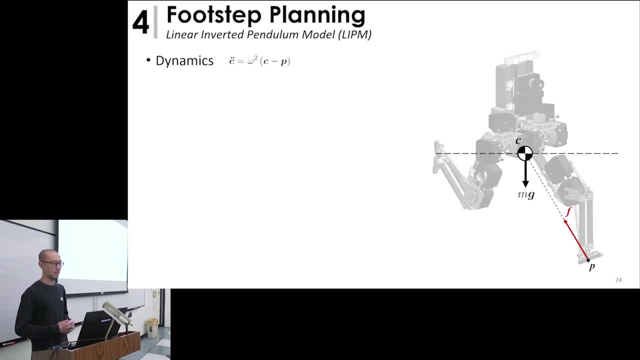 pendulum model, as the system dynamics is linear and the robot, you know, supported instead of on a single leg, resembles an inverted pendulum. the system states is the horizontal COM position because the vertical motion is constrained. the control input is the center pressure, which corresponds to the 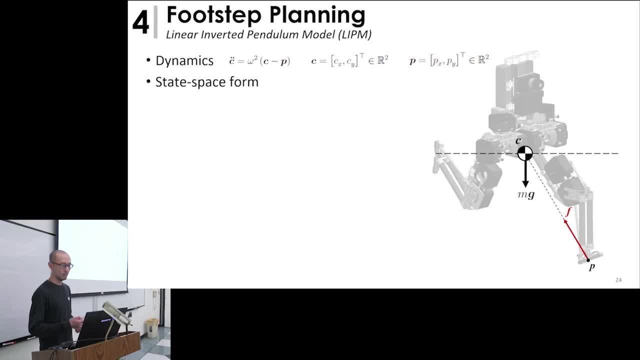 selection location. we can easily convert it into the state-space form and to analyze the system, we can perform a colleen transform. if we can define a transform equation in a clever way, we can derive a new state of C, which is just the linear combination of the COM position and the Tunnel equation. so this is all. 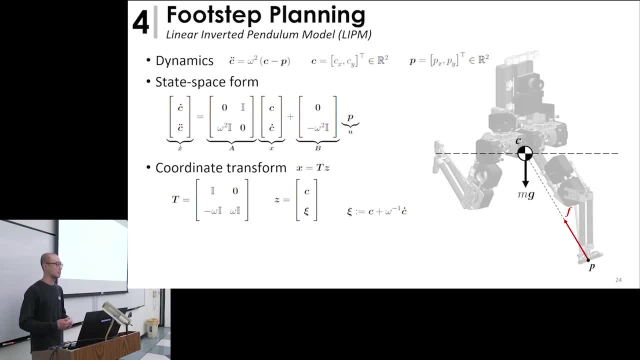 We tried to usual integrate the system conventionally and now we have equal y of three units. another example: Cé, the мехic civilians, are just linearées for one component which is a linear combination of the COM and velocity. and here's our new system. and apparently we can see the new system has 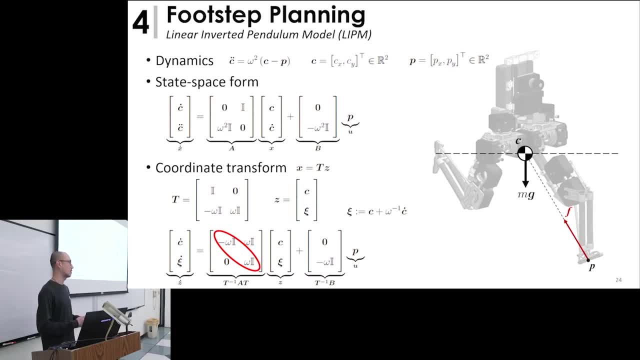 one unstable mode and one stable mode, which suggests that instead of focusing on both modes, we can just focus on the unstable mode. as long as the unstable mode is well controlled and bounded, the robot will not diverge, meaning the robot will not fall down, and due to this reason, this 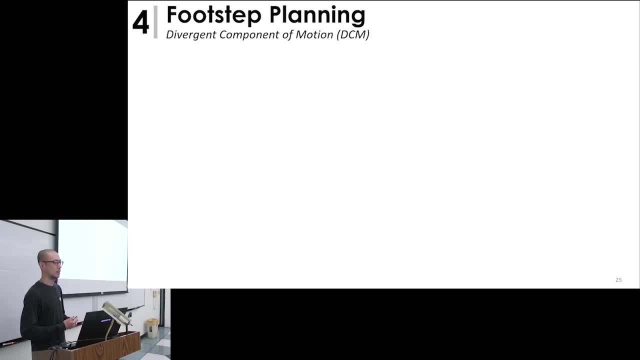 new state, c is called the divergent component of motion. we can have a diagram to better illustrate the system dynamics. so the new system has two states: the com and the dcm. the com dynamics is stable, as it's always, you know, following the dcm. the dcm dynamics is unstable because it's pushed. 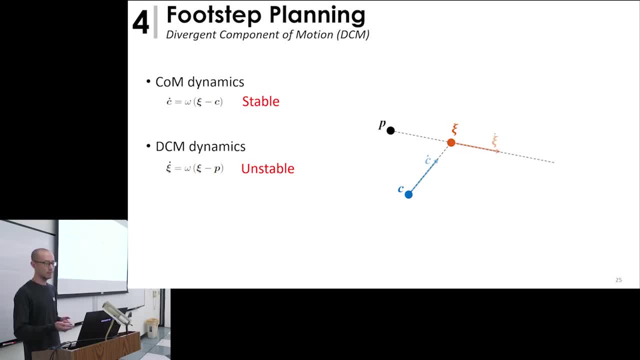 away by the cop. so as time passes, the dcm will just diverge and the com will follow and diverge at will. so to prevent the system from diverging, we can try to manipulate the cop with that. our dcm will be pushed away by the new cop. 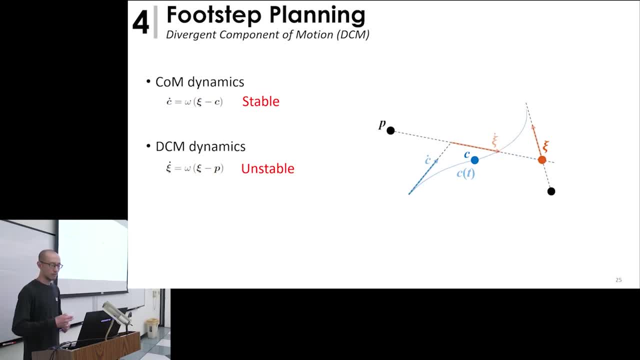 position and our com will follow as well. so from this illustration we can see that if we can control the cop in a clever way, to the right location at the right time, we can not only make sure the system is bounded, that is, the robot will not fall down, but also we can try to create some. 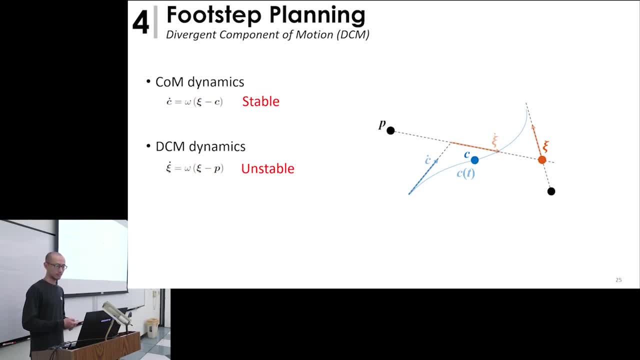 stable period orbits for working. okay, so let's have a quick summary of the reduced order model we're going to use for our footstep planner. so far, we have been talking about the stance phase, that is, one foot is contact with the ground. however, in order to achieve running and hopping, we also need to consider a flat phase. 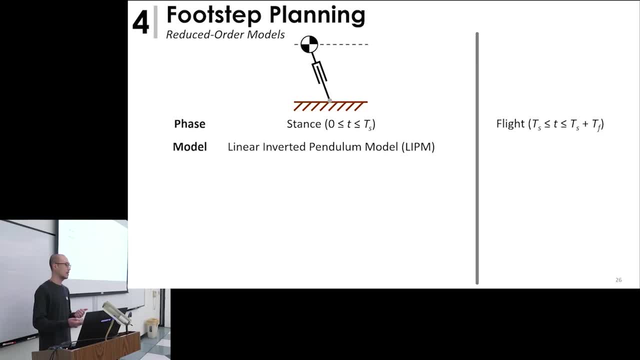 and fortunately during the five phase no external force except gravity can affect the clm state. so we can simply using a ballistic model to describe the motion and we derive the dynamics, the com and the dcm, and similarly, in during the flight phase, we can also derive the serum dynamics. 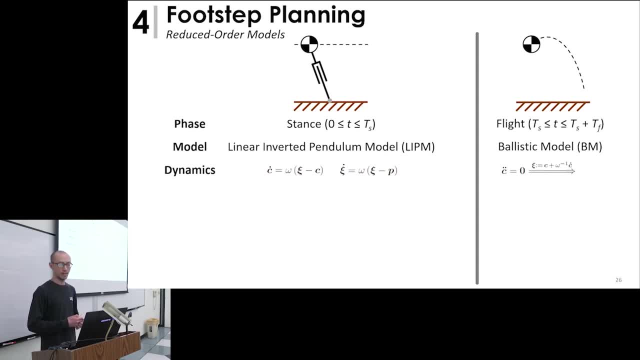 and, based on the dcm definition, we can also derive its dynamics. what's more, these dynamics are simple enough to be analytically integrated, so we don't need to worry about the granularity of the discretization of the model during during the planning process, which can be computational. 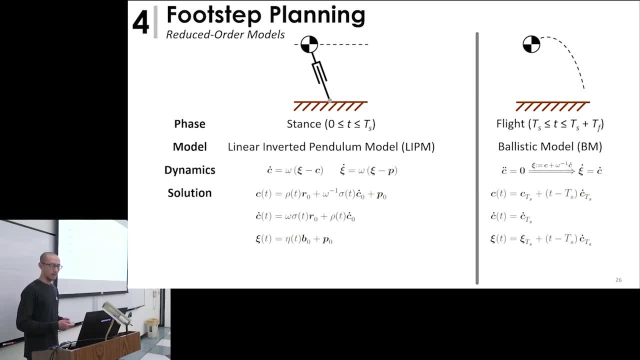 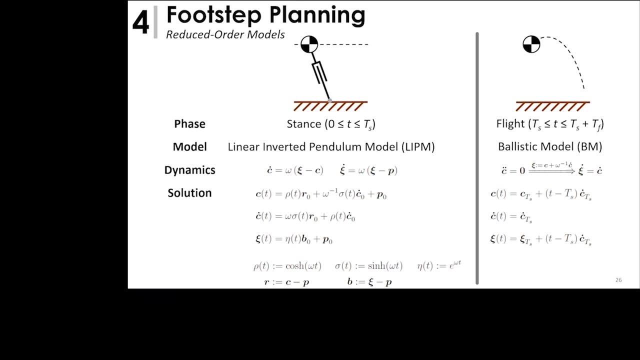 which can be computationally expensive. and here law, sigma, eta are just some known functions, and r and b are just a change of variable to make the equation more compact. and here r is the clm offset, e is the dcm offset relative to the sample pressure. 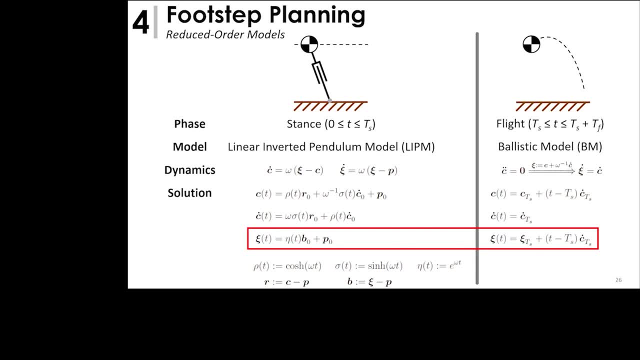 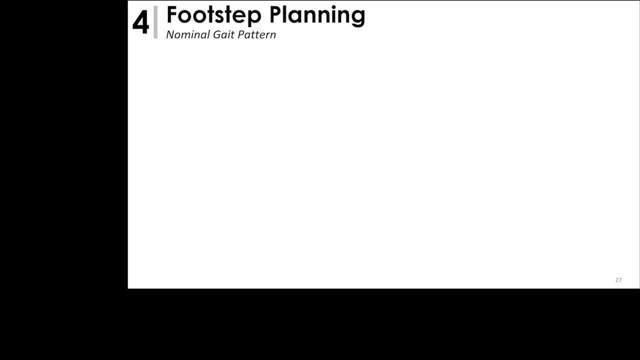 and of course we're going to focus on the dcm because it's the important mode. okay, so now we have the analytical dynamics mix, which makes easier to derive the nominal big pattern which is, you know, just some periodic trajectories of the reduced on model which will actually serve as the reference for our first step planner. so here's the diagram. 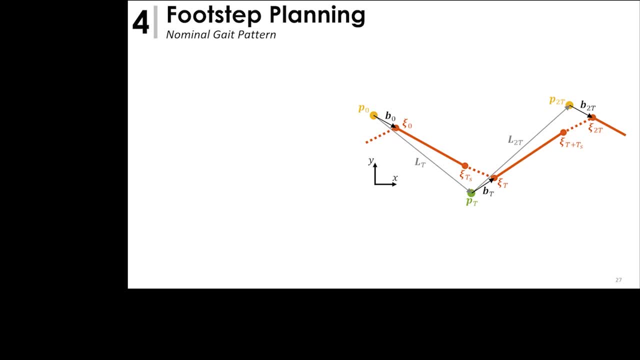 which, uh, you can consider, the robot is moving in the positive x direction. uh, the the yellow dots denote the left foot, the green dot denotes the right foot and its 2k cycles. so to sustain periodicity we need to have some constraint on the states, which is the displacement of the robot here, the zawd. 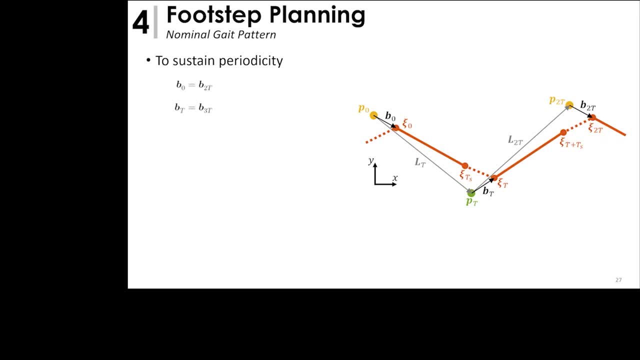 right. This simply means the robot state needs to equal to itself up to gate cycles. if we are automating left and right groups And using the analytical dynamics, we can easily solve for the nominal values. OK, And this one is for the DCM offset. 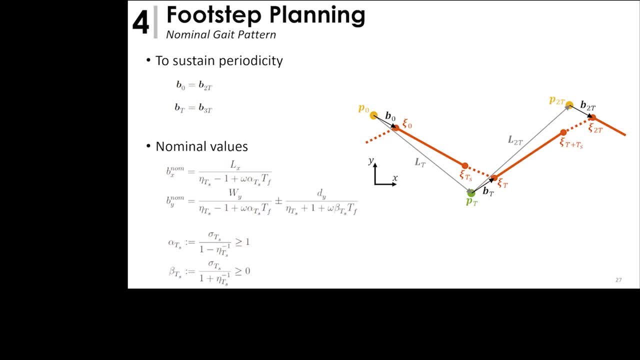 And here, alpha beta. I just change the variable. We can see the nominal values depending on the step length, Lx, and the step width, W1, which can be computed simply based on the design velocity And meanwhile, in the lateral direction. 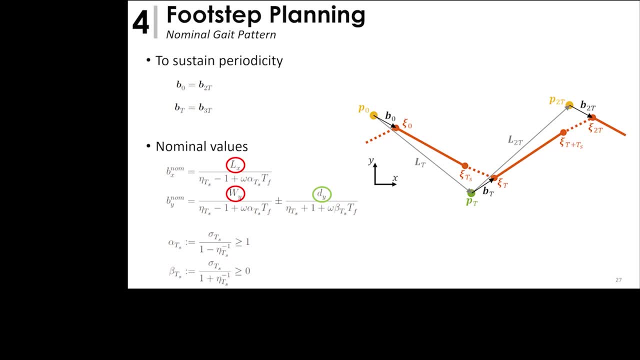 we also need to consider a Vy, which is due to the pivot squeeze, Because you know when the robot is moving, we don't want the two legs too close to each other to prevent collision. OK, So can I just ask, just to make sure? 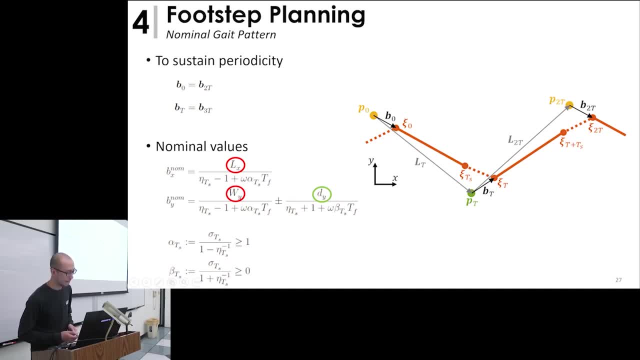 when you're talking about this. the first two equations basically ensure periodicity, right? Yes, yes, These are kind of like bound boundary conditions, Boundary conditions, Yeah right, So OK, so you're going to ensure the periodicity by having initial and terminal boundary conditions, which? 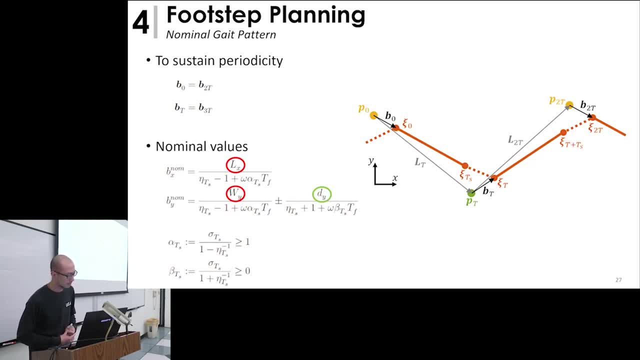 you have to satisfy: Yes, exactly, OK, Yeah, And once we have the boundary and once we have the analytical dynamics, we can solve for the nominal values And also we will have a dy in the lateral direction. As I said, we have to solve for the nominal values. 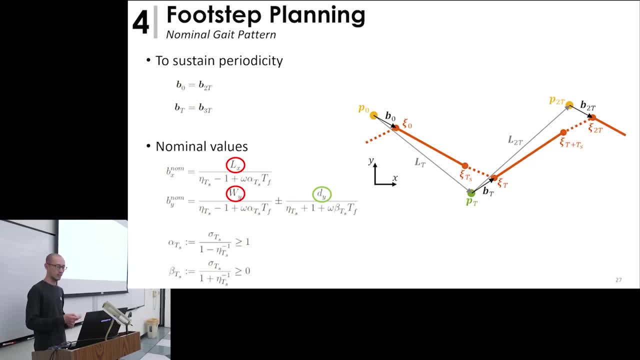 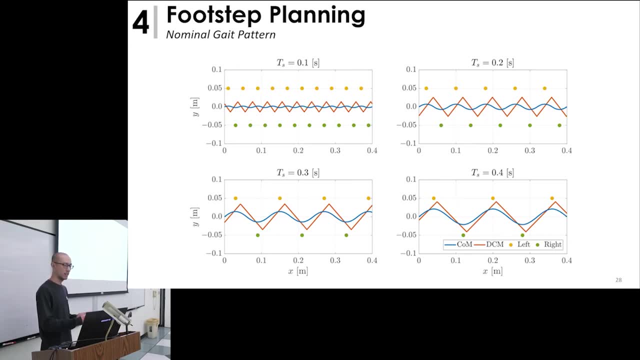 We need to specify a clearance between the two feet to prevent collision. Once we have the nominal gate pattern, we can just plot it, see how it will change once the parameter is changing, And this one is in terms of stance duration, As we can see when the stance duration is increasing. 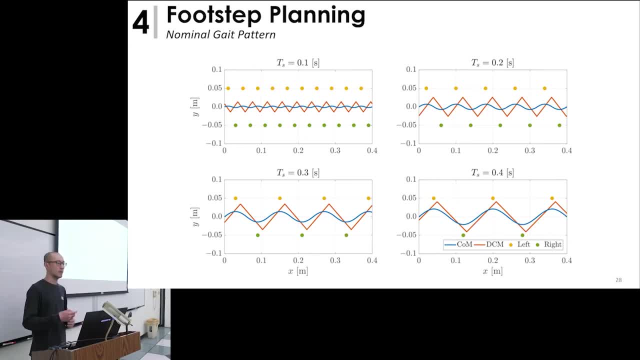 the robot will swing more in the lateral direction. So, based on this, we kind of know how to choose Ts in order to have a good working posture. And meanwhile, when Ts is increasing, we also see that the step lengths increase as well. 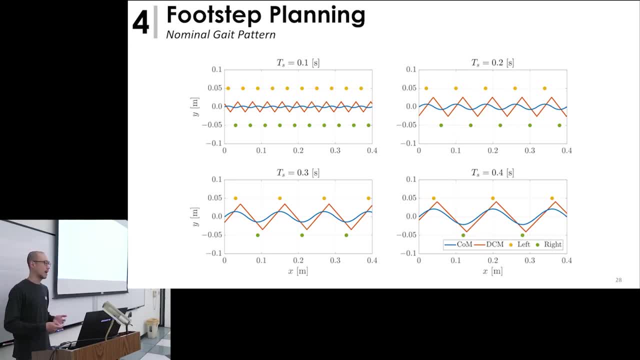 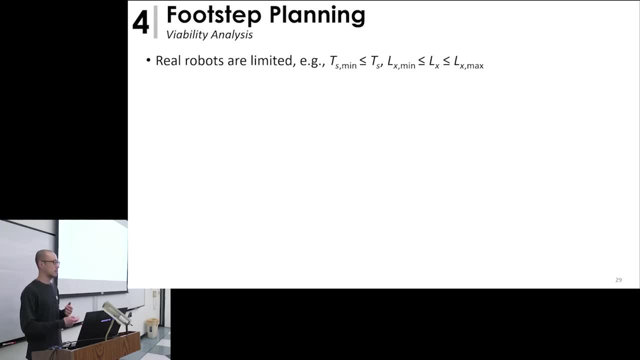 However, for an actual robot, we cannot have arbitrary large steps, neither can we have arbitrary short stance duration, which basically means the real robots are limited. We cannot place the foot to anywhere at any time we want. So this actually is the. Let me ask you a question. 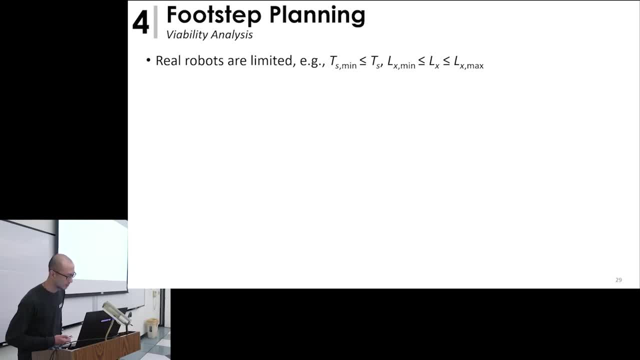 Do you optimize with respect to the step? Yes, In other words, do you? Yes, Well, is that one of the control parameters? Yeah, the control parameter is the step location. Well, OK, But basically the time interval from B. 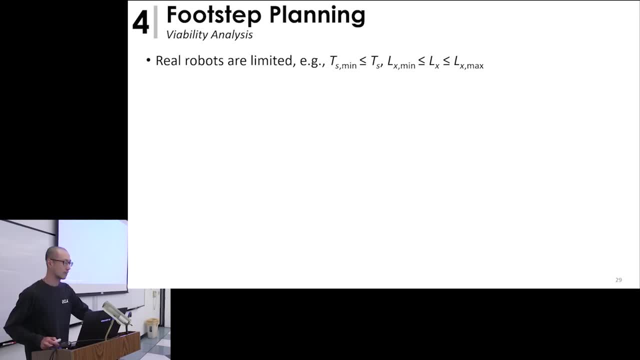 I guess I'm not sure exactly what B is, but from B0 to B2t or something, the time interval between there. is that optimized as well? Yes, yes, For the current gate cycle the time is also optimized, OK. 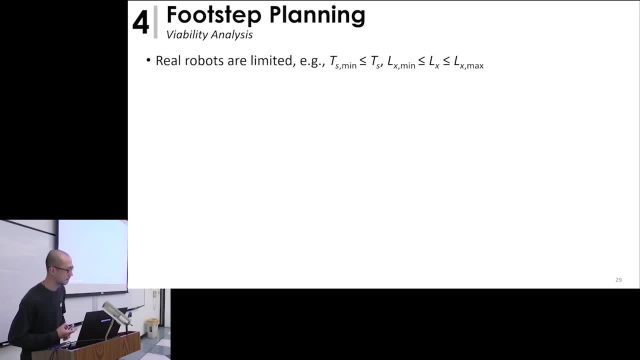 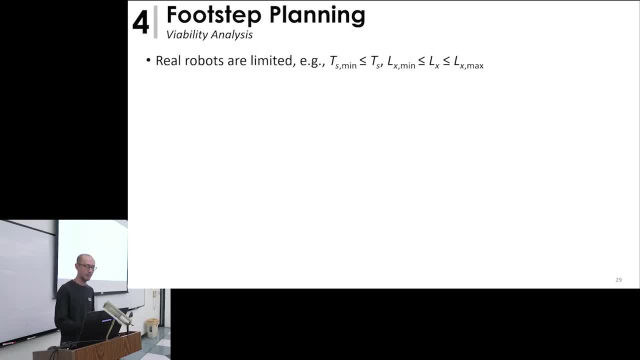 This actually implies that there must exist some boundary, that if the robot stays across this boundary, the robot cannot handle, and And we can try to investigate this limit, And the process is called viability analysis And the tool we're going to use is called n-step capturability. 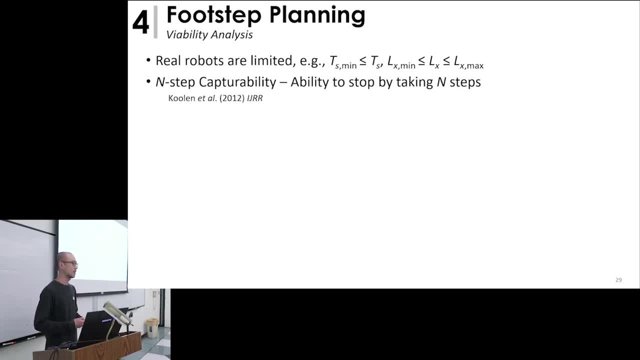 the ability of robot to come to a stop by taking n steps. For example, if my current DCM is right on top of my COP, the offset is equal to 0. Then the DCM will not be pushed to anywhere. Therefore, I don't need to take any step to come to a stop. 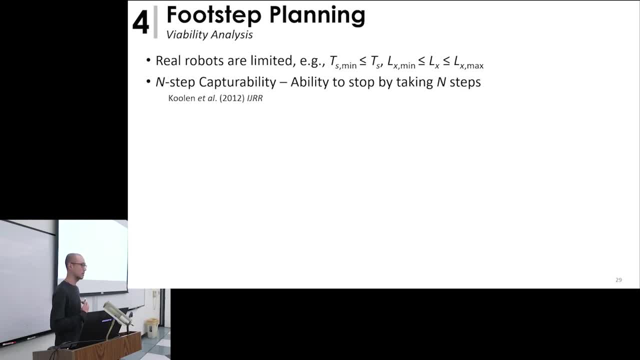 However, if my offset is non-zero, which means I'm starting to tip over, then I might need to take one or two steps to come to stop. However, if my offset is too large, then probably I cannot avoid falling down because the DCM will just diverge too fast. 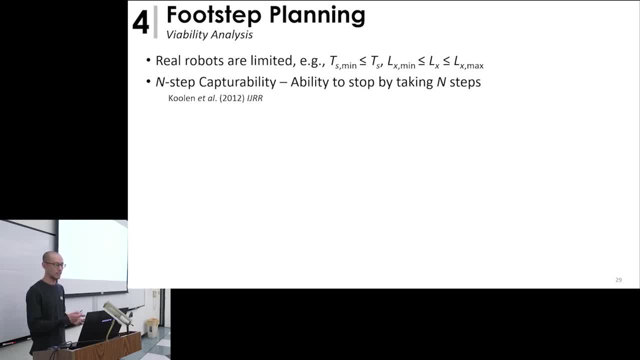 So mathematically, let's say in the x direction, let's say the state is n-step capturable, meaning the initial DCM offset is upper bounded And then up to one gauge cycle the DCM offset is going to be n minus 1 step capturable. 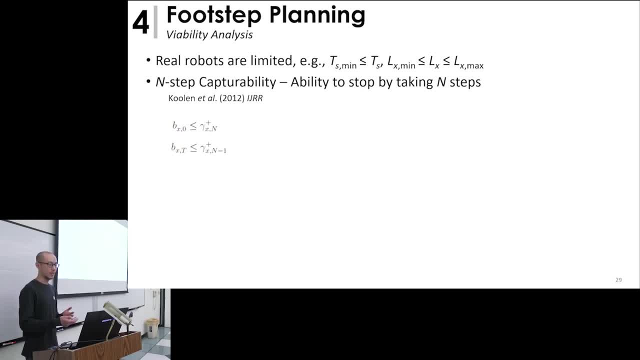 And since we have the dynamical dynamics, we can evaluate bxt using bx0.. And here's, after some rearrangement. this is the result: Now we have a new upper bound, And this upper bound will be maximized when we take the largest step using the shortest step. 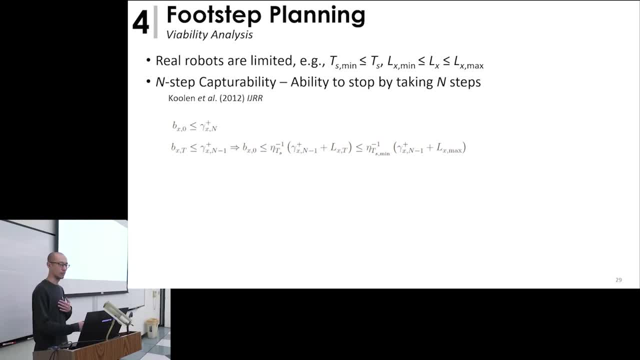 because this is the best we can do in order to prevent falling. And now these two boundaries should equal to each other, which leads to a recursive expression And we can easily solve this geometric series and by taking the limit, We can find the infinite step. capture, ability bound. 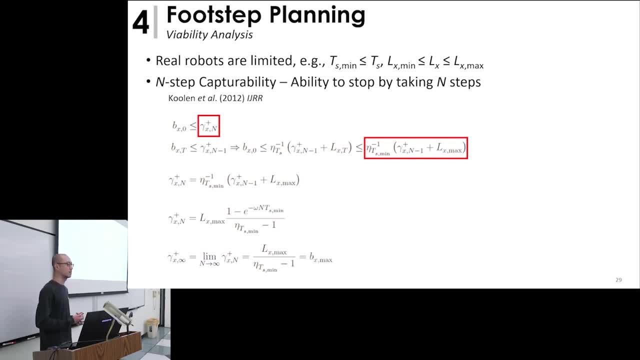 which is equivalent to the DCM offset limit, because theoretically it takes the robot infinite steps to come to stop. Basically it means the robot will not stop at all And any value within that the robot cannot handle and will just fall down. 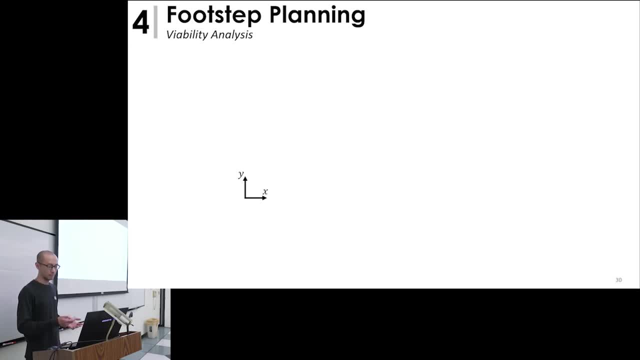 Again, we can use some diagram to illustrate the viability condition. Suppose at some time, Given the left foot position of the current gait cycle, we can first derive the feasible footstep region of the next gait cycle based on the constraint on step length and step width. 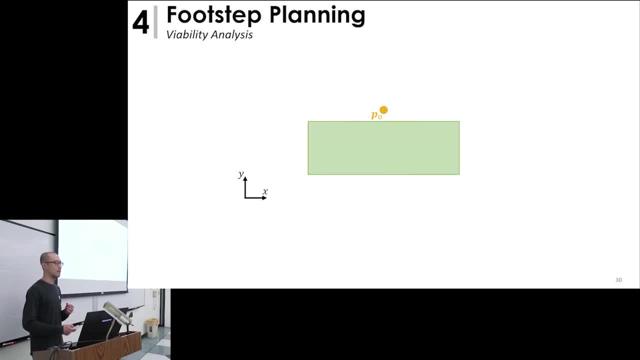 So it's this green box. And then the variable set of the robot state, the DCM state, can be derived by further adding the DCM offset limit. It's this green box. The system is viable. That means the robot will not fall down as long as the DCM offset of the next gait cycle is within this green box. 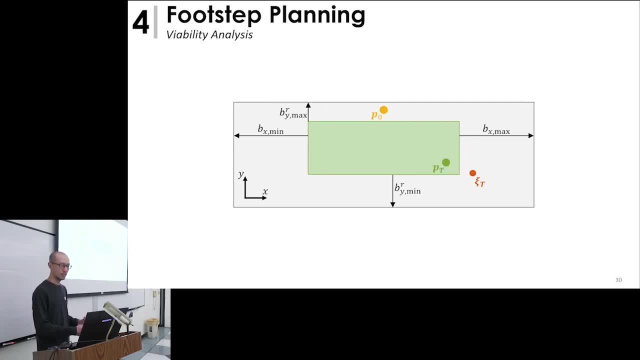 Because I can always try to find a footstep location to make sure the DCM offset is bounded by the limit we find. However, if the DCM is outside of this green box, the best we can do is just step on this corner. 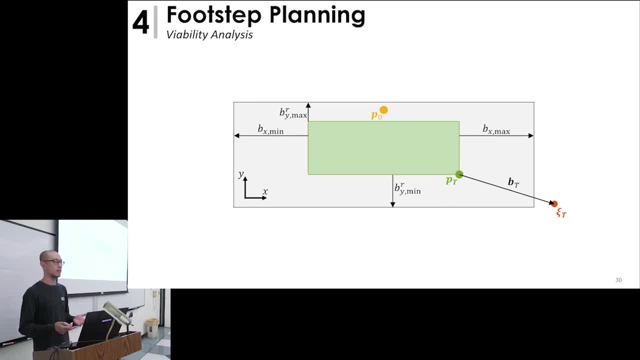 However, as you can see, the DCM offset is still larger than its limit. So that's it. The robot cannot avoid falling down and might need to prepare for that. So that's the viability condition. So now we have talked about the reduced order dynamics, the nominal gait pattern, the viability analysis. 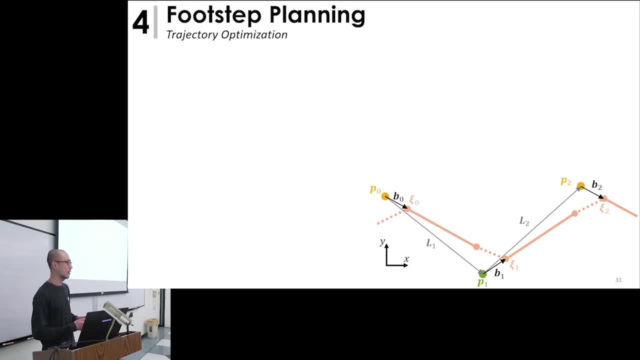 We have everything for our footstep planner, So let's try to formulate this trajectory optimization problem. The footstep planner adapts the nominal gait pattern. The function is going to penalize the state deviation with the nominal values, Of course in the least square sense where the vector norm squared is defined as this. 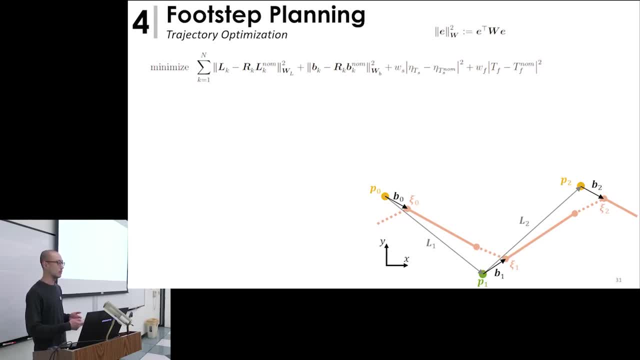 The first term is for the step length and the second term is for the DCM offset. The last two are for the phase duration And also we are considering a few steps ahead of time. So the capital N is the number of previous steps into the future. 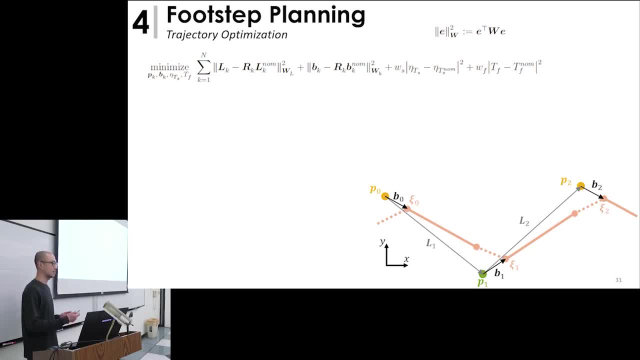 So the DCM variables will be the footstep plan. The first step will be the footstep locations, PK, the DCM offset, BK for the next N gait cycles And meanwhile we are also optimizing the phase duration And note that we are using eta TS, eta TS instead of TS directly to ensure the linearity of the constraints. 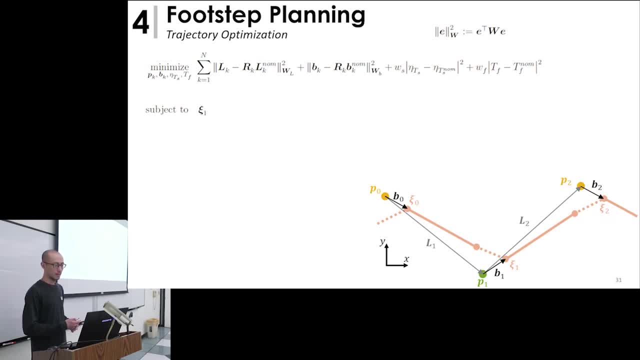 So the constraint is, of course, the system dynamics. So, using the analytical dynamics, we can predict our state KC. KC1 is the state corresponding to the upcoming touchdown moment. Either we are during the stance phase or during the flight phase. we can predict KC1 based on the current measurement. 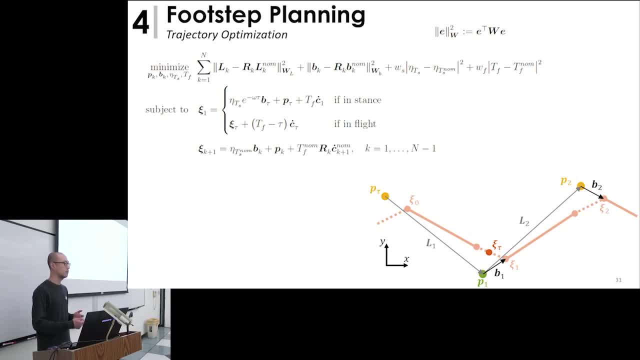 And in the long run we can also predict the DCM evolution for the next N-1 gait cycles. And again, the robot is limit, so we also have some constraints on the step length, Some constraints on the phase durations, like this: 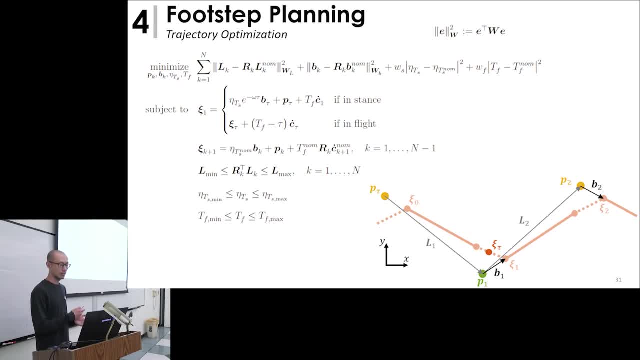 And finally, to ensure the robot will not fall down, we also need to specify the viability constraint. We just talked about it. However, if the robot cannot avoid falling down, adding this constraint can make the problem infeasible, because there's no way the robot can recover. 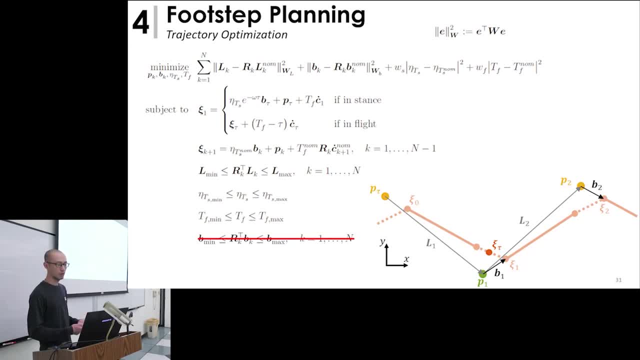 So, in practice, we just remove this constraint And instead we will increase the weight WB so that it will guide the plane DCM offset as close to the nominal value as possible. as close to the nominal value as possible, even though viability is not guaranteed. 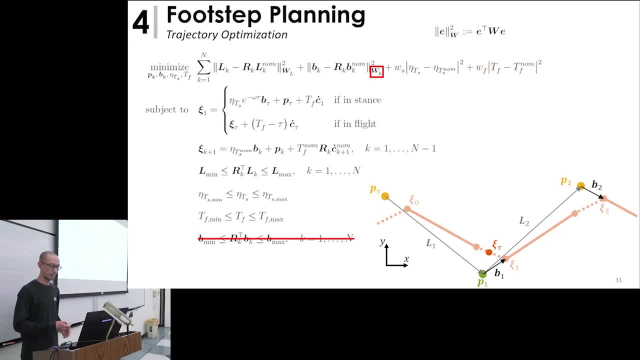 Because in this way we can always have a solution. Hey, can I ask you a question? Sure, When you talk about close, so you have a perturbation which I guess is zeta, zeta, Zeta, And you're comparing that to the nominal path. 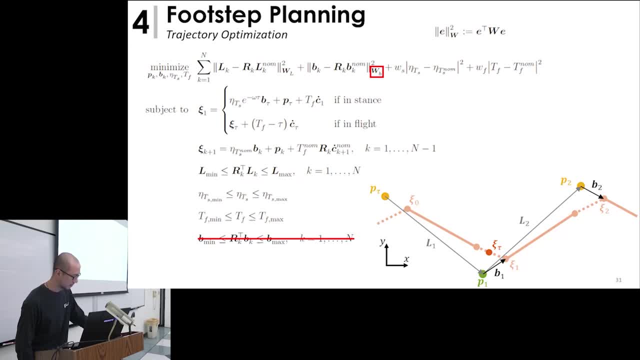 Nominal path, yes, Nominal path, But basically when you do that is the perturbation, basically some projection perpendicular to where the nominal path is, Because the nominal path is in time, You're using time, You don't make a perturbation at the same time. 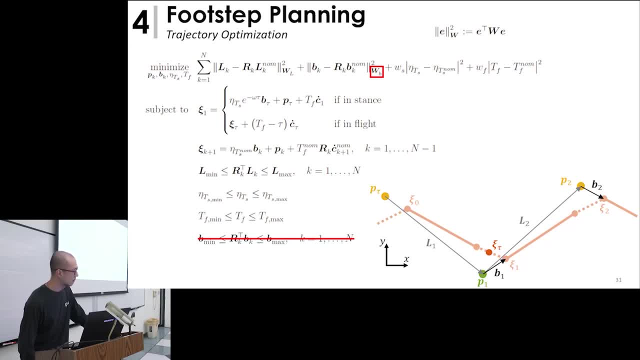 You make a perturbation in a different way. Exactly, how do you compare zeta with the nominal path? I guess is what I'm asking. Can you repeat your question again? Well, what I'm asking is: how do you? the nominal is a time function, right? 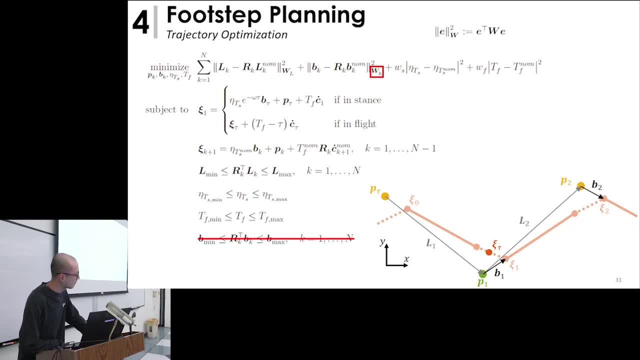 Yes, yes, And zeta is your perturbation's off. You're using time. So when you make the perturbation, how do you make the perturbation? Is it with respect to the same time? Do you make a perturbation with respect to? 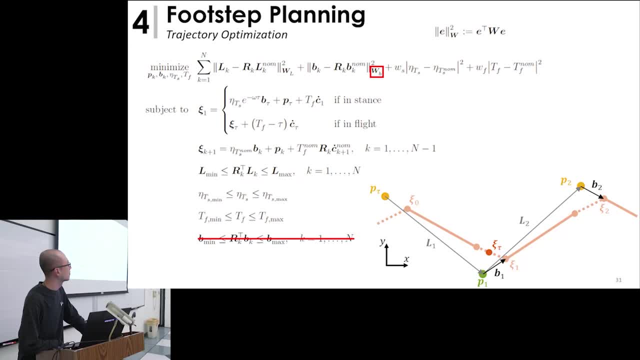 where you are perpendicular, It's away from the nominal path. I'm just kind of wondering how you make, how you decide on what your perturbation away from the nominal path is, given where you are. Yeah, so first the nominal values is not. 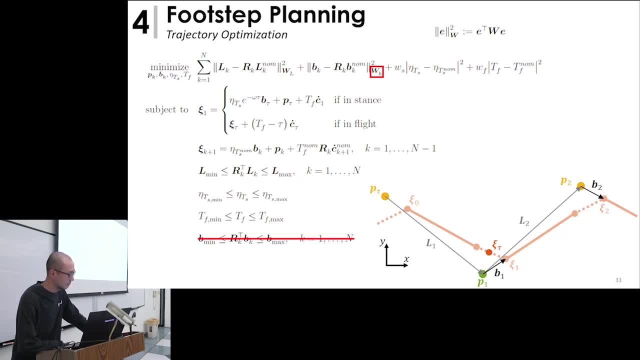 is just a value. It's not a time series, It's just a nominal value. So where on that nominal do you choose? I mean, it's basically general. Yeah, so the nominal values is at each touchdown moment. It's in a moment, right? 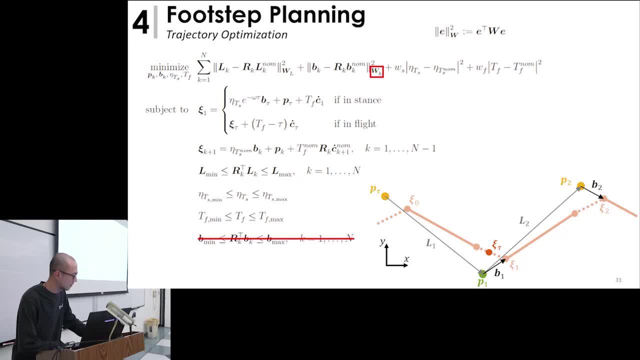 Yeah, It's a function of peak time in some sense, some independent variable. I'm just sort of wondering how you make a perturbation away from the nominal path. How do you define it? All I'm asking is a definition of how you define a perturbation away. 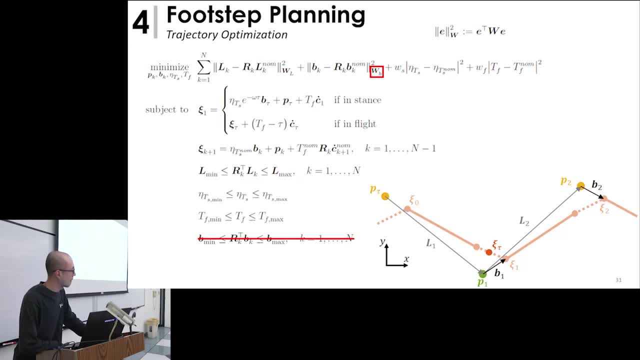 How do you compare where you are with a value on the nominal path? Where do you choose on the nominal path as the value you are going to use to make a perturbation? Is it just maybe an orthogonal perpendicular to the path or some sort or something of that sort? 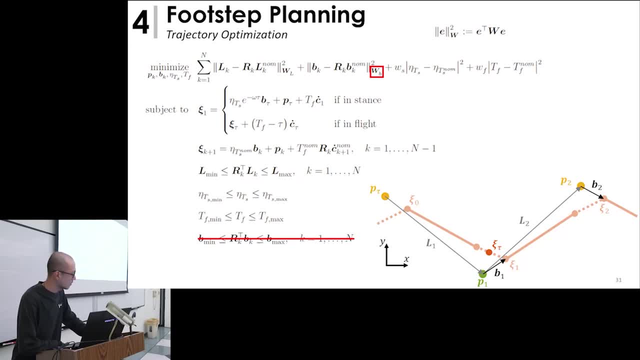 So right now you mean the definition of the perturbation. Yeah, Okay, The definition of the perturbation, The perturbation. right now everything is linear, so you can just consider it in one dimension. So it's just the difference between the current state. 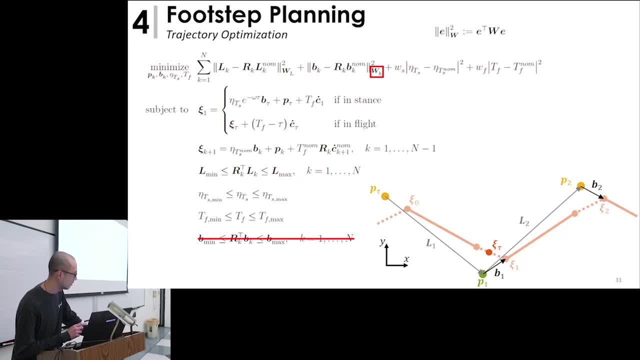 and the nominal state. But the nominal state is a. it could be anywhere, right? Where on the nominal do you pick? As I said, the nominal value is at each touchdown moment. okay, So it's just a value at each touchdown. 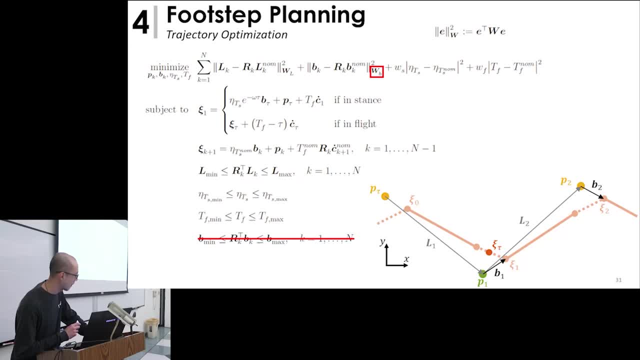 Yeah, but you could pick it at t. you could pick it at p, tau, you could pick it at p1,. you could pick it somewhere in between. Where do you compare the data to? That's all I'm asking. Yeah, so we are picking either zero. 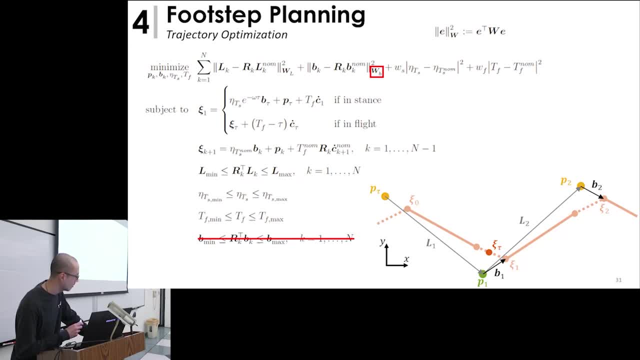 either t equal to zero or t equal to the capital T. Yeah, that's actually the boundary. Okay, Could he be asking where the nominal time comes from? Is that from the previous analysis that you were doing Like tfnone? where is that coming from? 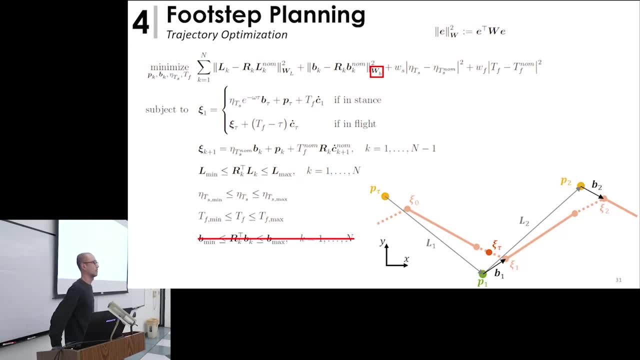 No, tfnone is just a nominal value you define by yourself. Yeah, I think, is that what he is asking. He's trying? I think he's trying to ask the definition of the perturbation. at which time? Well, you're at the current time, now right? 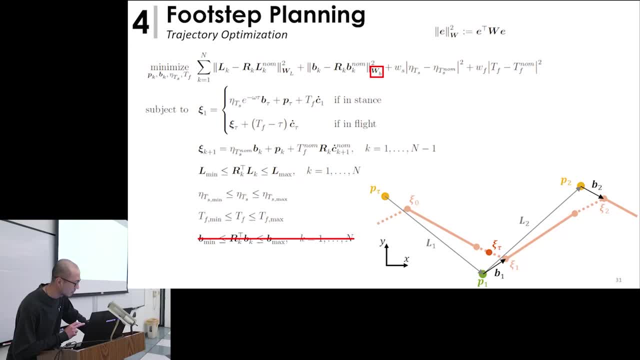 Yeah, You've got the actual state. Yeah, I'm just asking. you're at that state and you want to compare it to your nominal trajectory. Yes, And I'm just sort of wondering: what point on the nominal trajectory do you choose in order to make the perturbation? 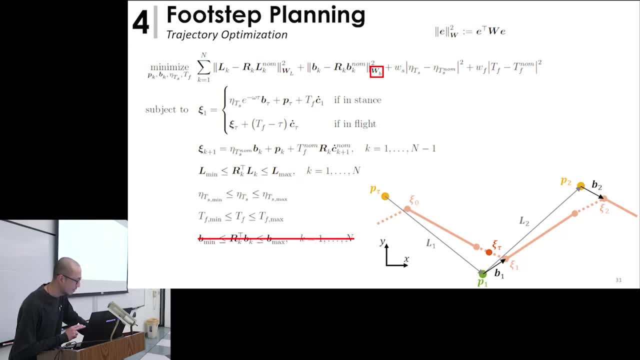 Yes, So right now the time is tau. Okay, Right now the time is tau, but I'm comparing the state at touchdown. So that's the end of the nominal trajectory, That's the final state, So you're at. 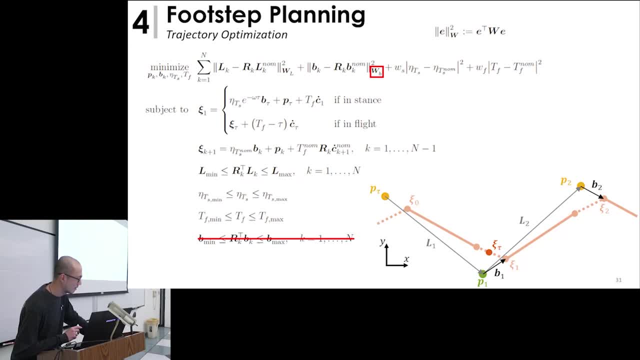 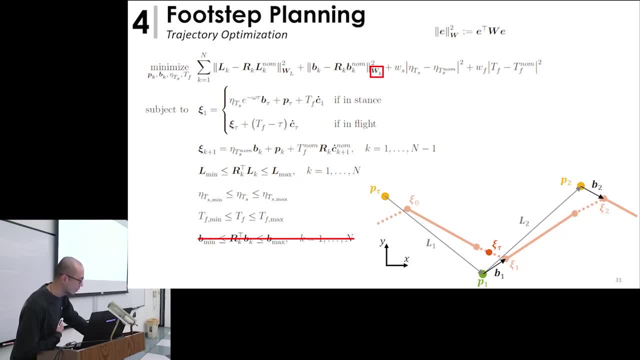 Yeah, Right now we are at zeta tau. Yeah, But we are comparing at- But zeta tau is compared with where Zeta tau is from the current measurement. We are using the dynamics to predict zeta one, Right, Yeah? 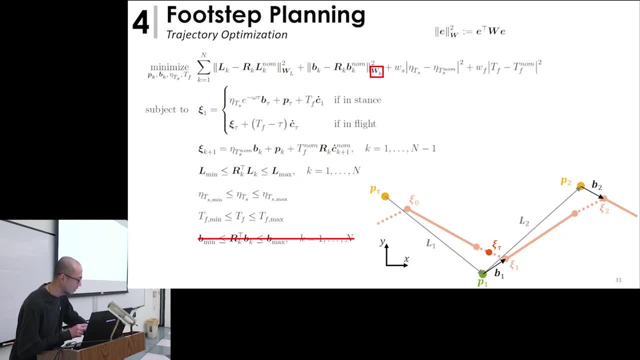 Okay, You're going to predict zeta one. Yeah, Zeta one is. I compared this to the nominal values. I tried it- But. but basically you are making a perturbation, so don't you compare it somewhere which is: 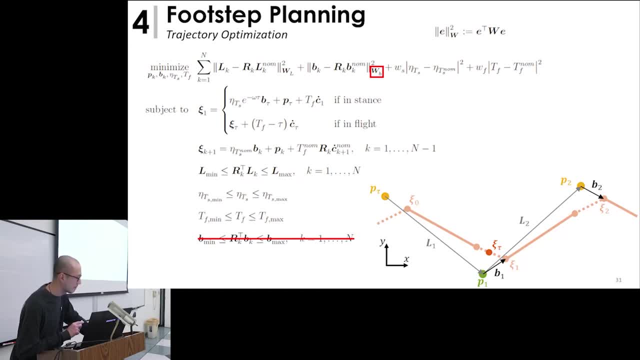 a perturbation with respect to the to the normal path. Oh yes, I see the confusion is so, basically, zeta 1 is equal to b1 plus p1.. And, as you can see, the decision variable is actually p, the location. 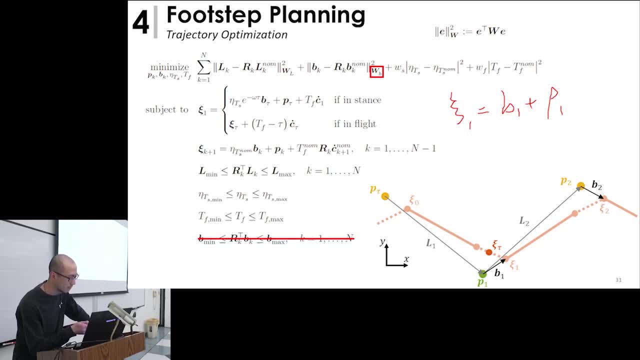 We are not comparing zeta 1.. We are actually comparing b1.. Because b1 is the actual nominal value, We're going to compare it with the nominal trade group And b1 is at what time? At the touchdown, at the next touchdown. 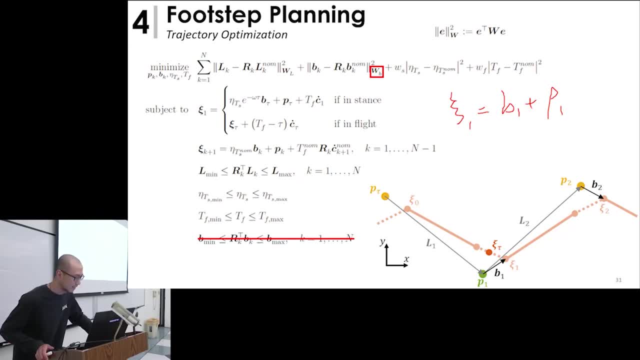 Right now the food is in the OK, so it's at the touch point. It's the touch point. Yeah, Right now we have b1 below there, So zeta tau is somewhere there. So you're going to use b1 plus and row 1 is what. 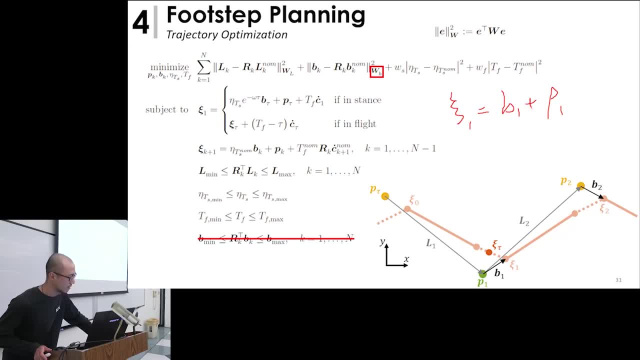 This is p1.. p1 is the next food set location we're going to optimize. Yeah, we try to optimize p1 and b1 simultaneously. p1 is the next food set location. OK, well, you're generating a brand new. so, in a sense, 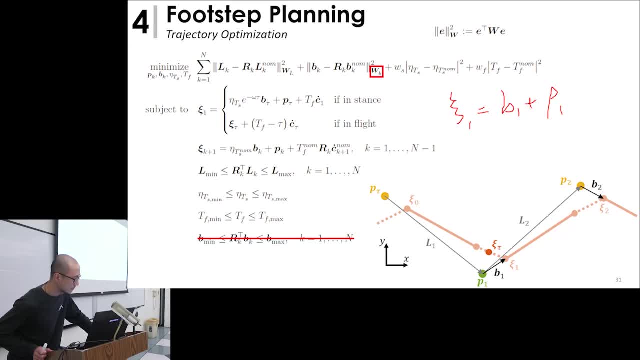 you're generating not a perturbation but a brand new trajectory. Exactly, exactly. I'm trying to re-planning a new trajectory as close to the nominal. OK, As close to the nominal trajectory as possible. OK, then that's all in your cost function. 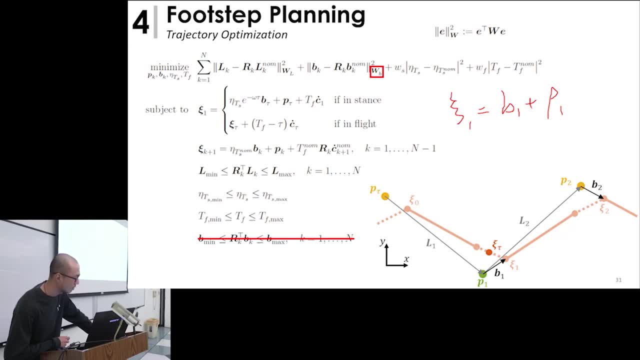 Yes, yes, I see So the cost function keeps you close, Keep you close, But what you're doing is finding the underlining parameters that are associated with each of those points, like b1 and things like that. Yes, things like that. 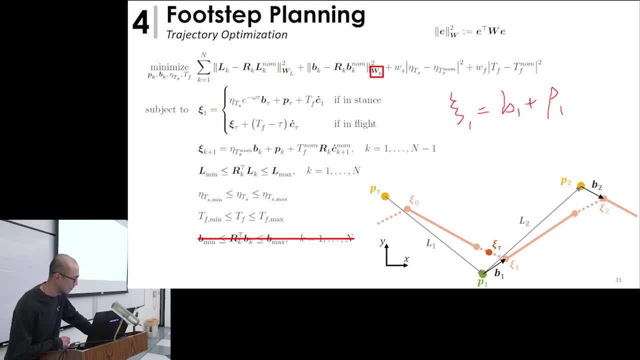 Which we had before. I see, Yeah, OK, Yeah, so the food stamp planner is trying to, you know, re-planning the trajectory as close to the nominal trajectory as possible. Yeah, but it's based on the current measurement. 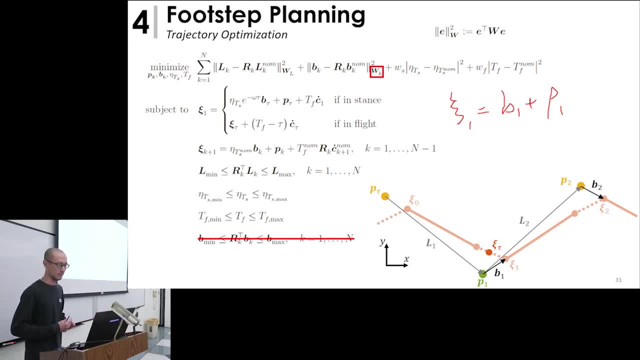 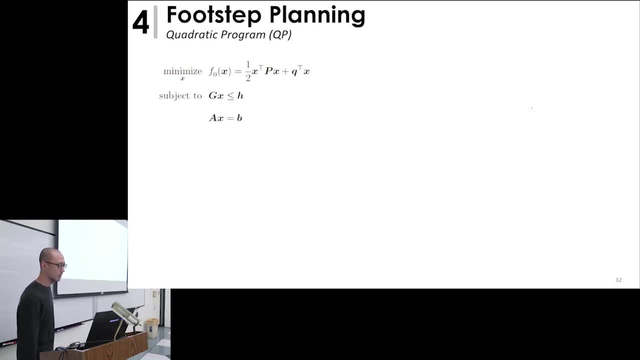 the current state of the robot. OK, OK, OK, thank you. So essentially, the food stamp planner, the optimization program, can be transcribed into a qualitative program, because the cost is in a qualitative form and all the constraints are there. 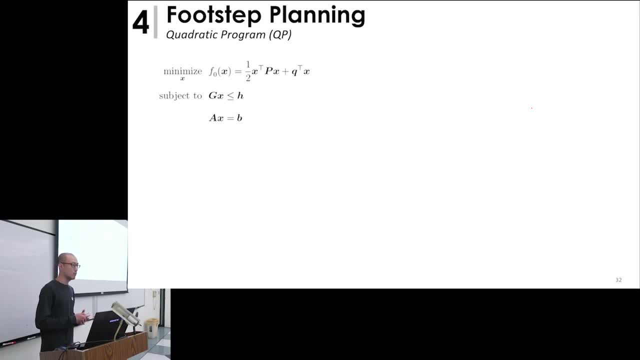 OK, OK, OK. The reason why we want to do it in this way is because, if feasible QP can be solved very efficiently and with guaranteed global optimality- And there are a lot of QP solvers we can just utilize- 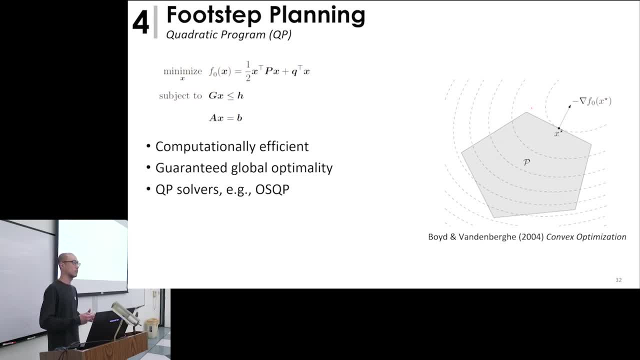 For example, QoSQP, which has proven to have a very good numerical stability. And finally, based on our formulation, our food stamp planner is really a small-scale QP problem, even with multiple steps, So it can be solved in practice at a rate of 500 hertz. 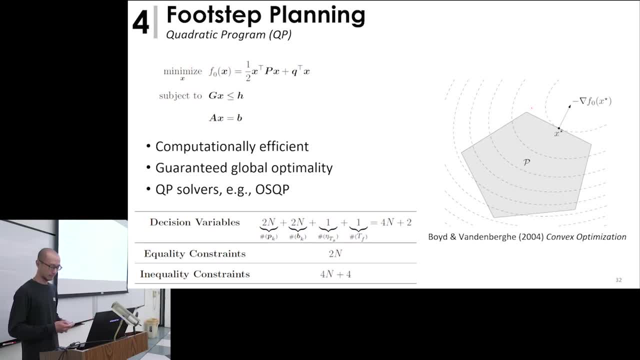 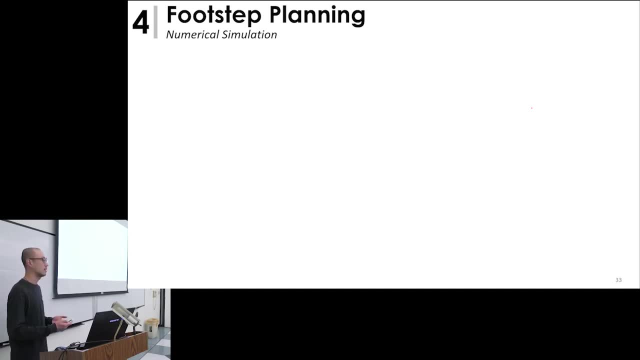 sufficient for real-time re-planning. So now let's just test the food stamp planner. We first implement it on the reduced-order model, meaning the model the controller uses is exactly the same as the simulation model, And meanwhile we have a timing gap magnet. 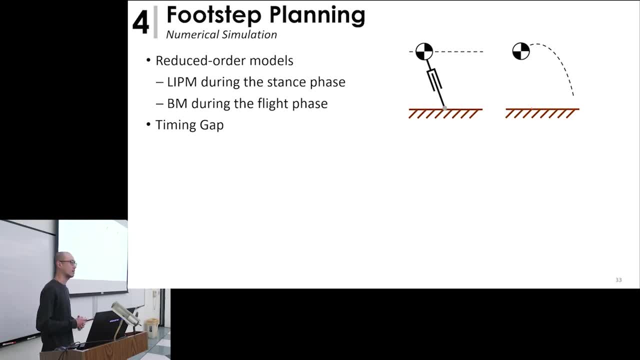 Because we don't want to move the load at the end of the gate cycle, so we actually stop planning some time before the gate cycle ends. OK, And these are just some parameters of the simulation, For example, the weight of the robot, the height of the robot. 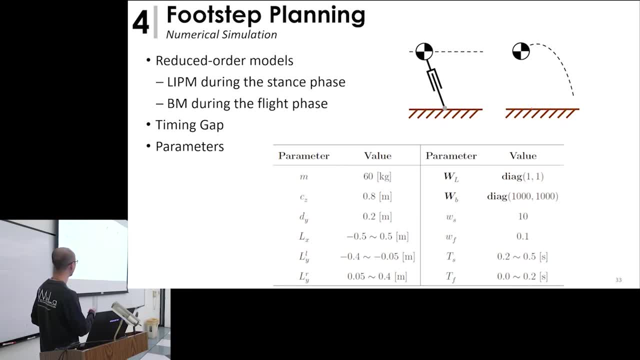 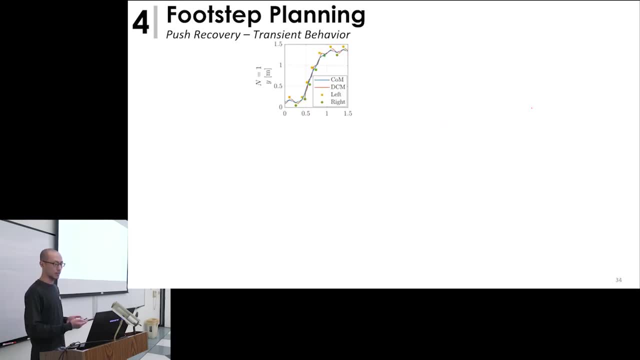 And, as you can see, this WBA is set significantly larger than other parameters in order for the viability. OK, now let's just run the simulation. When the robot is moving in the positive x direction, we push it to its left. As you can see, the push is very strong. 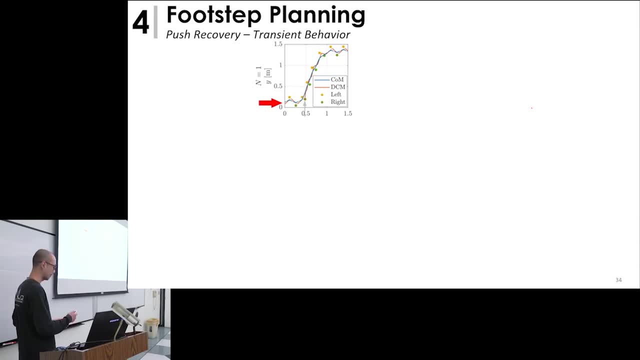 And the robot took several reactive steps to come to a stop. And here's the optimized phase duration. You can also see that when it's first pushed, the phase duration drops significantly, which means the robot is taking a very fast step in order to prevent falling down. 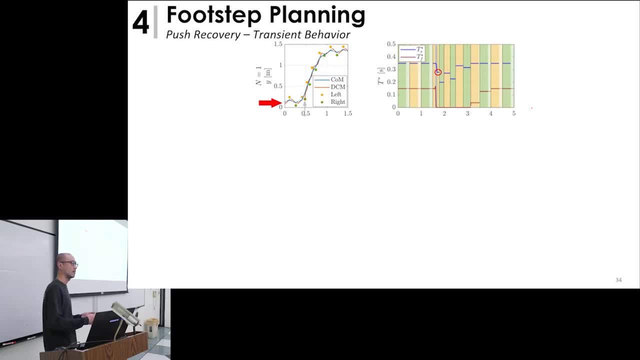 And also due to the timing gap mechanism, it stops planning sometime before the gate cycle. OK, And basically we verify our full-stem planner works. And, by the way, this is only for the result n equal to 1, meaning we are only planning for the next step. 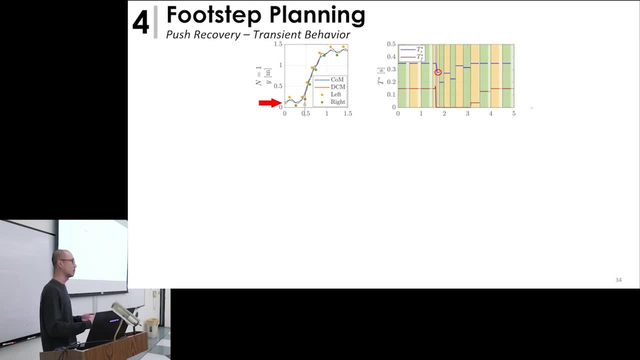 We also try to investigate the number, the effect of the number of previous steps on the system. And here's the result: for n equal to 2. We can see the performers improve significantly, The robots can recover faster and it's closer to its original path. 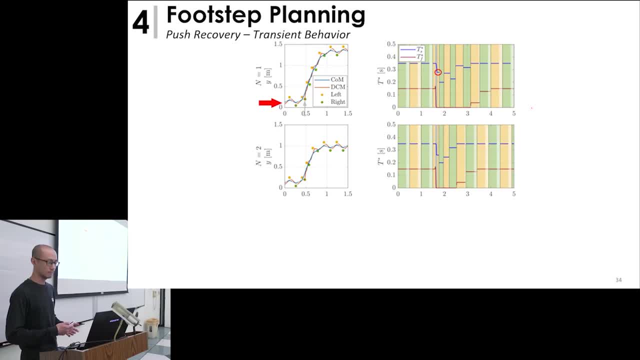 And the planned phase duration is also less chaotic. OK, This is due to the fact that the full-step planner is more aware of future information to have an overall better plan. OK, Because right now we are not considering the lag crossing scenario which will limit the feasible start region in the lateral direction. 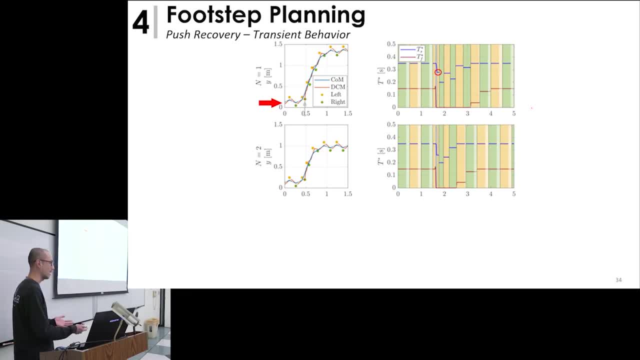 If the full-step planner knows OK, in the next gate cycle I cannot compensate. I cannot catch the fall too much. it will make more efforts in the current gate cycle And this is the result for n equal to 3. And, as we can see, it gets even better. 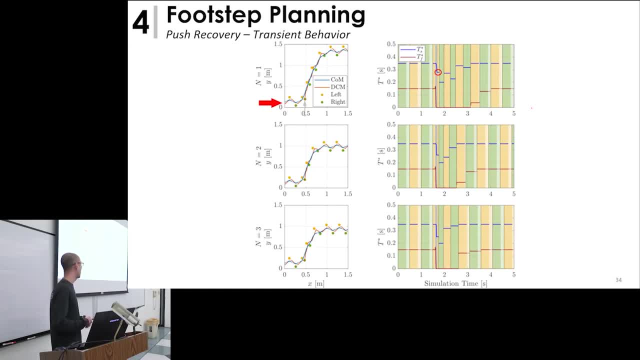 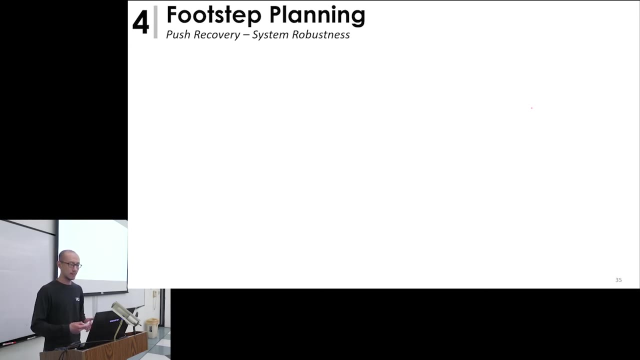 We also tried n greater than 3. However, it will not significantly improve any more, So you can see kind of it converged. OK. We also try to investigate the system. robustness: that is the maximum push the robot can resist before falling down. 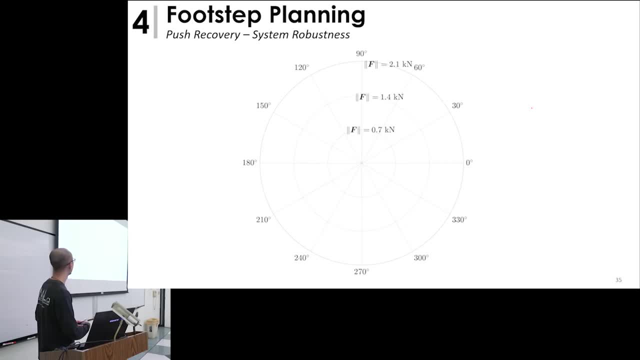 So in each push direction we gradually increase the speed And- this is very interesting- We gradually increase the force until the robot falls down. So with phase duration fixed, if we do not optimize the phase duration, the force region is like this: 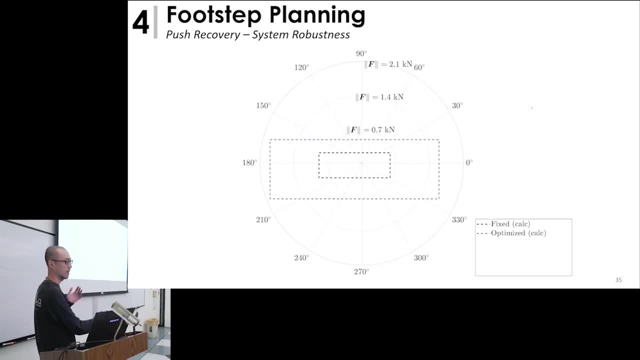 If we optimize the phase duration as well, the force region expands significantly. So from this we can conclude that optimization phase duration is as critical as full-step location to bipedal locomotion. And, by the way, these are only the theoretical boundary. 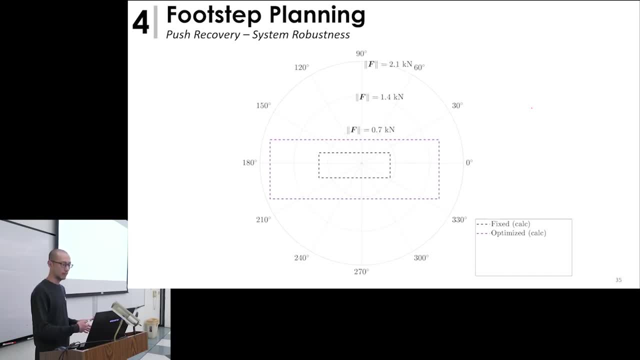 Based on the bipedal analysis. we can easily verify these theoretical boundaries using simulation And with phase duration fixed, the simulation results will match the theoretical boundary, no matter how many steps you play, Because the best you can do is just take the largest step. 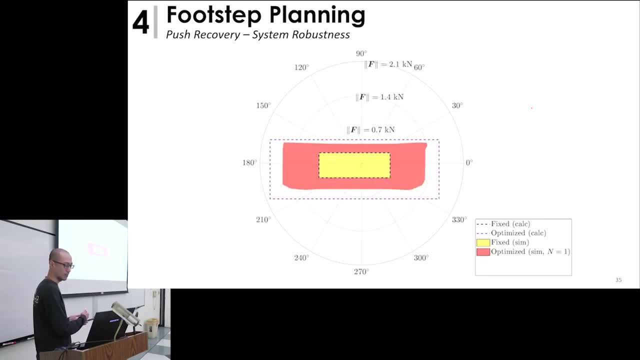 With phase duration optimized the phase duration, the force region gets bigger and bigger as n gets bigger. However, they do not quite match the theoretical boundary. Again, due to the timing gap mechanism, it stops planning some time before the gate cycle ends. 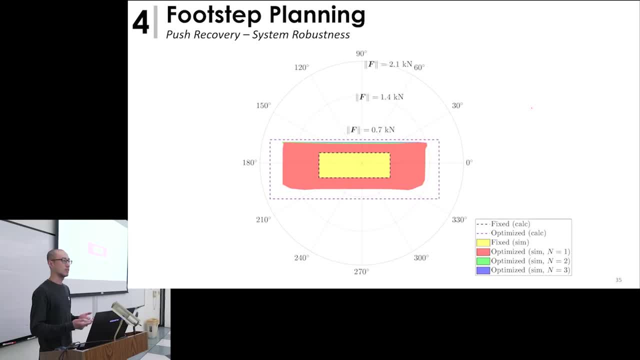 And there's no response during that time, which will essentially decrease the system stability margin. So, based on these simulation results, we can say: n equal to 3 is a wise choice in terms of system robustness, transient behavior and computational efficiency. 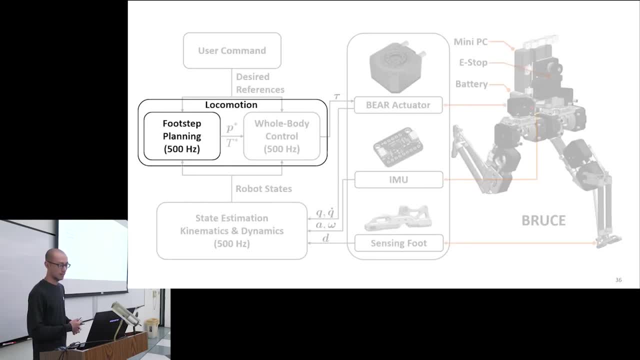 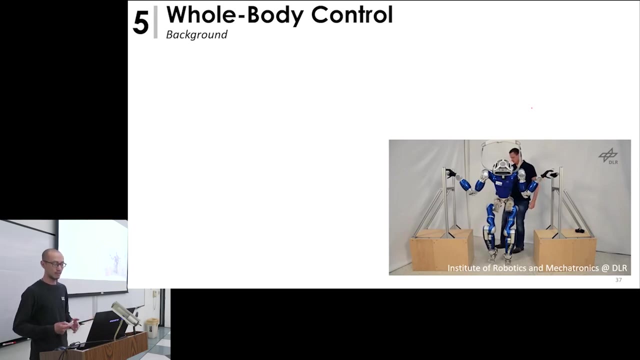 So that's pretty much about the full-stem planer. Now let's move on to the next step. We have a discussion on the whole-body control, which actually makes the robot move. Whole-body control is a good candidate for simultaneous execution of multiple tasks. 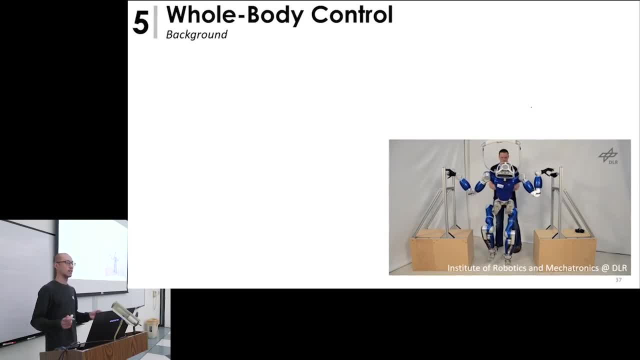 for a redundant floating-based robot interacting with the environment. In addition, it can create very fast, agile, compliant motions, yet without sacrificing accuracy. It typically uses inversely-controlled dynamics to properly handle the counter-force interaction with the environment. However, you know ID-based whole-body control heavily. 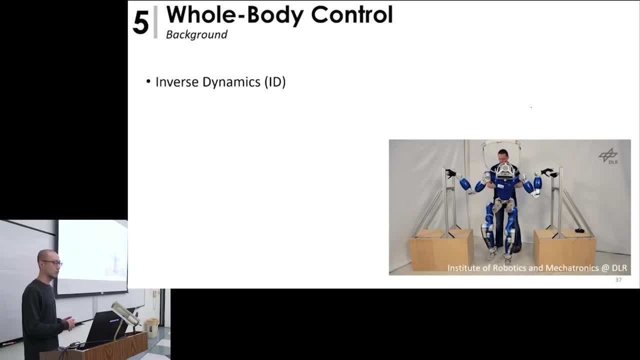 depends on the high quality of the dynamic model, which is often difficult to obtain in practice. In other countries, the robot kinematics model is much easier to get with high accuracy. So examples also exist which are based on the inverse kinematics or even a combination of both. 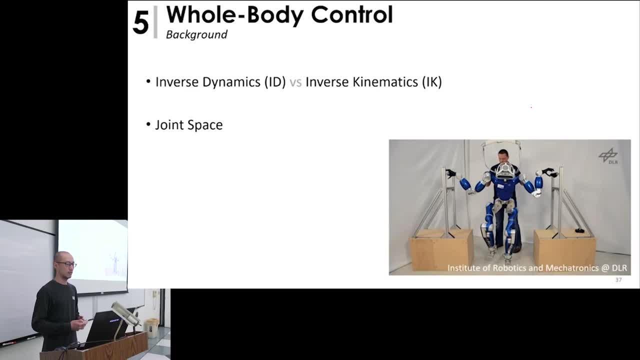 And, in addition, other approaches usually consider trajectories in the joint space, resulting in an incredible amount of motion details, And in other countries, operational space can show easy disburden by designing the trajectories in the intuitive operational space. However, all these methods cannot handle contact stability. 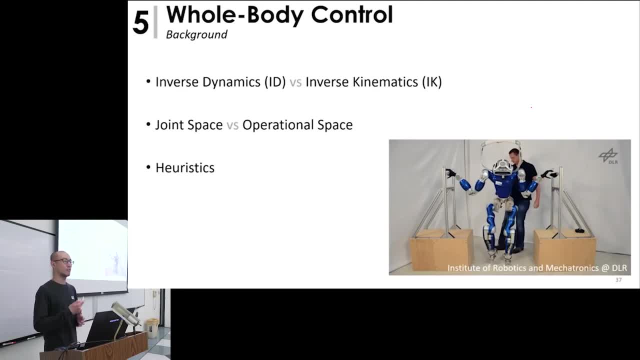 or joint limits well, the violation of which can easily cause poor performance or even control failure. And lately, an elegant way to implement whole-body control- oh-ah-ah can have a HP domain for a retired user- is by doing aなんだ tool where 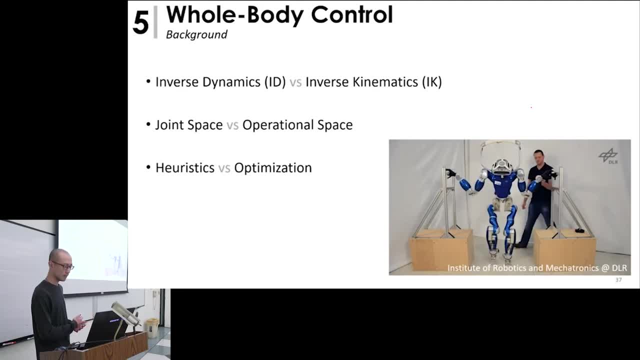 a robot master sets boundaries. The layer of mechanics of the UNW trait. somehow un Individuality Contain You. brown line will do the job. Having that combined with a variety of data routers can grant better productivity to our users and dismiss, make a tests nothing and repeat. 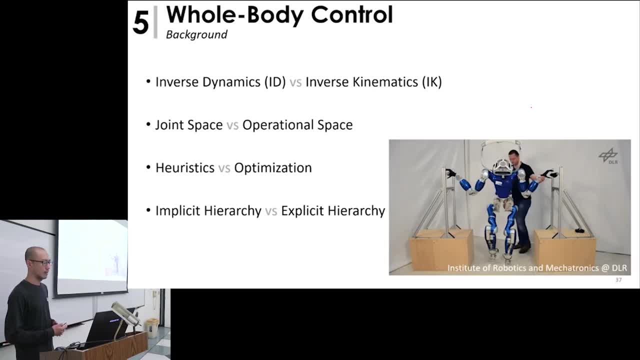 That is not Behavior Design. straighten time and space, And there's used to be only a Beta, too Right. A strictly hierarchical framework serves cascaded qubits from the highest priority to the lowest priority And in our framework we're going to use the inverse dynamics. 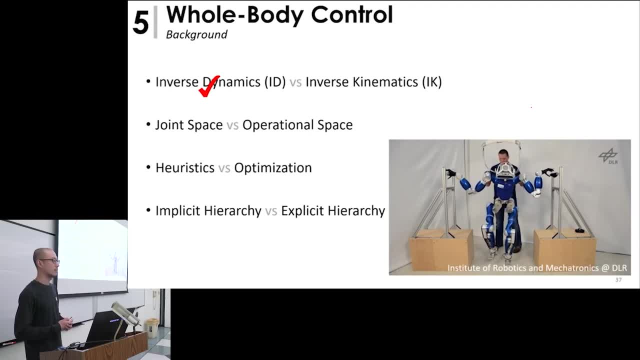 because we actually have a good dynamic model due to the motor transparency. We're going to work in the operational space, because the reduced order plane does not consider the joint motions. We're going to utilize optimization, again, to properly handle the various physical constraints And, finally, we're going to choose implicit hierarchy in consideration of the computational cost. 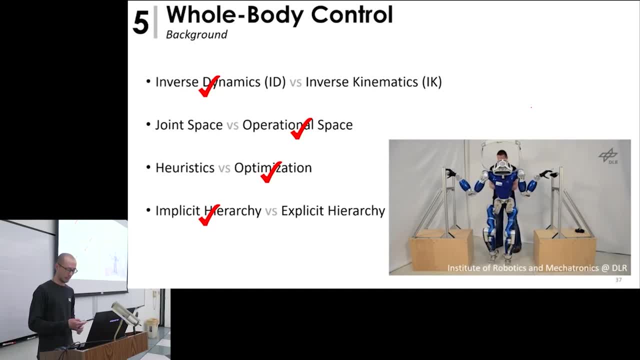 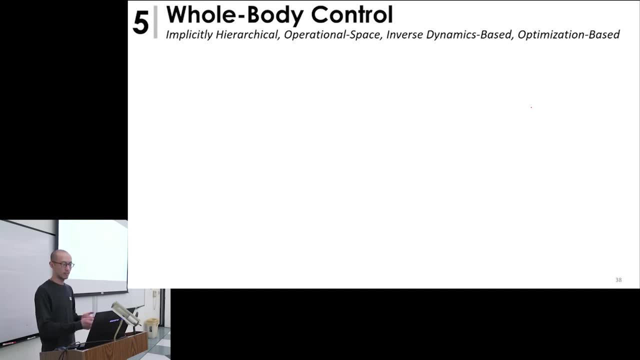 because we only need to solve one qubit instead of multiple ones. Okay, so now let's see how we can actually formulate this implicitly: hierarchical, operational space, inverse dynamic based over the control using optimization. So since we are considering dynamics, we're going to work on the acceleration level. 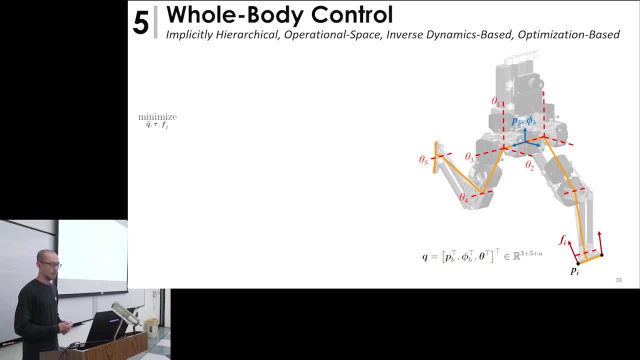 So, given designed operational space acceleration, we're going to work on the acceleration level. So, given designed operational space acceleration, the goal of holiday control is trying to find the instantaneous required, dynamically consistent joint acceleration, joint torques and contact force. Since we're tracking some reference, we're going to penalize the deviation between them. 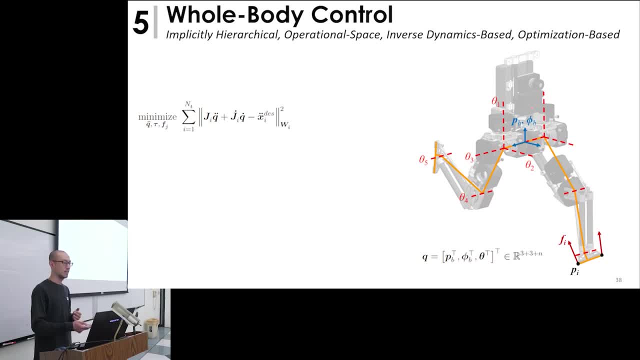 And, as you can see, the I's operational space task is set as a qubit cost, with priority being implicitly enforced with a weight WI, And here JI is the TAS decode beam, And our desired acceleration consists of both feed-forward and feed-back terms in a PD form. 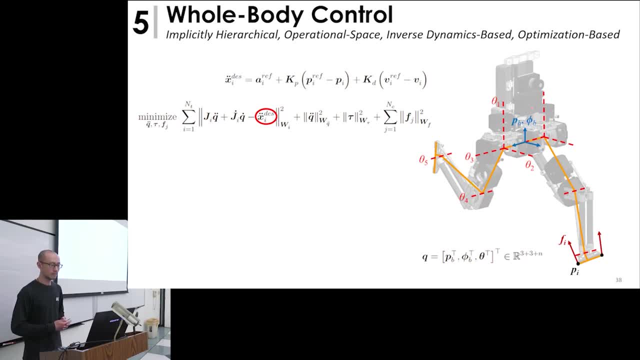 And in addition, we also add some regularization terms to make sure the overall qubit cost is always positive, definite, even if we know the TAS decode beam has some similarity, which can avoid potential numerical issues. And finally, we're going to try and do some ס' integration. 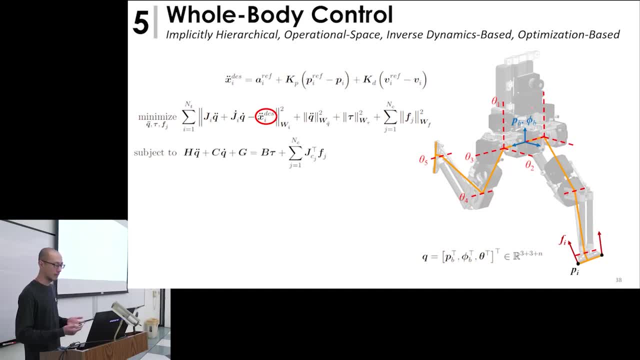 And finally, we're going to try and do some sql acceleration. Finally, the constraints is, of course, our forward dynamics, our floating base model, as well as the contact constraint, zero-contact acceleration and the friction core. So let's take a look at each component. 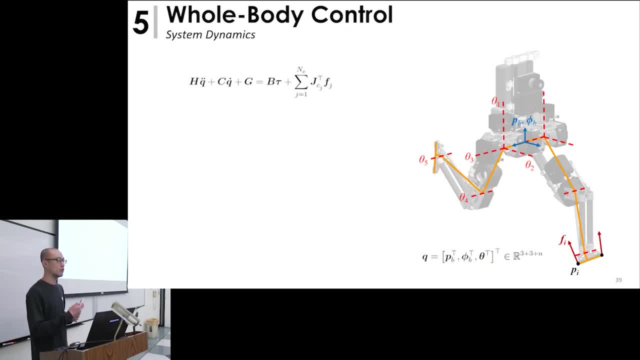 So the first one is system dynamics. We have been talking about the forward dynamics, which is way too complicated for the planning. However, the instantaneous system dynamics is actually linear in terms of the design variables, because the other variables can be obtained from the measurement. 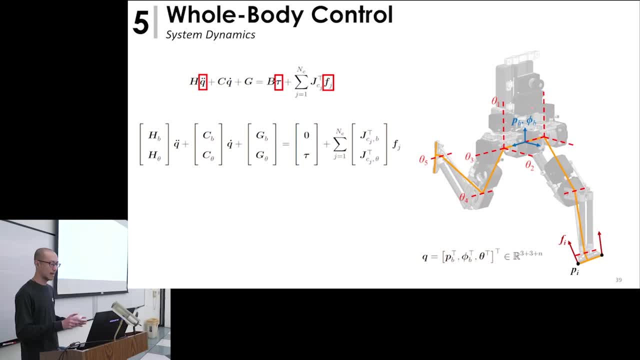 And notably the system dynamics can be split into two parts, the floating base dynamics and the joint dynamics, To accelerate the QP performance. we can only focus on the floating base dynamics, because in this manner n constraints can be removed. Meanwhile variables for the joint torques. 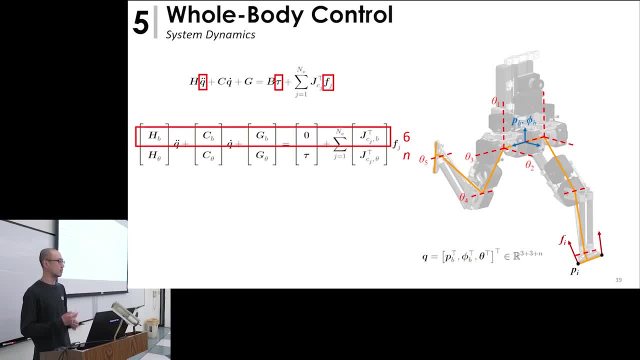 can be removed As well, if we assume that there's always enough torque to achieve the generated motions. And in the end, once the QP is solved, we can easily compute the optimal joint torque based on the optimal joint acceleration and contact force. 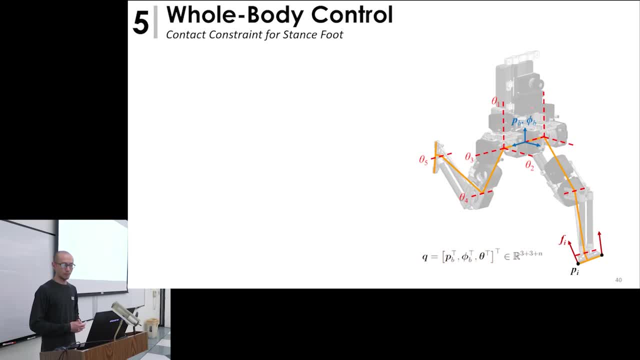 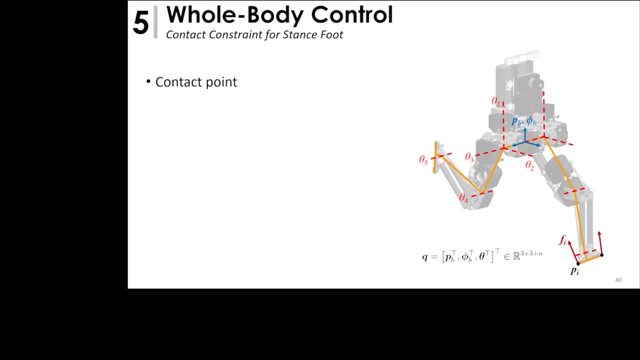 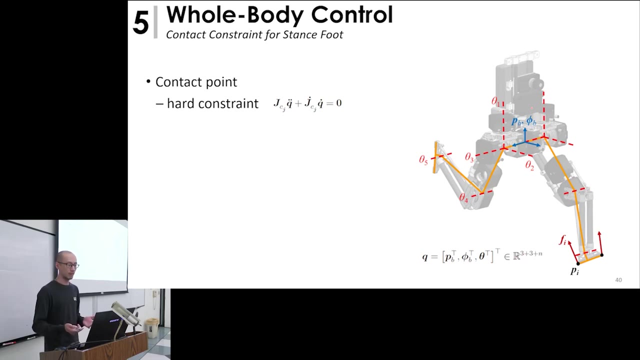 And the next one is the contact constraint For Bruce. with a line feed we consider two contact points for each foot: the toe and the heel. For each contact point we need to specify a zero contact acceleration constraint to prevent the foot from moving. 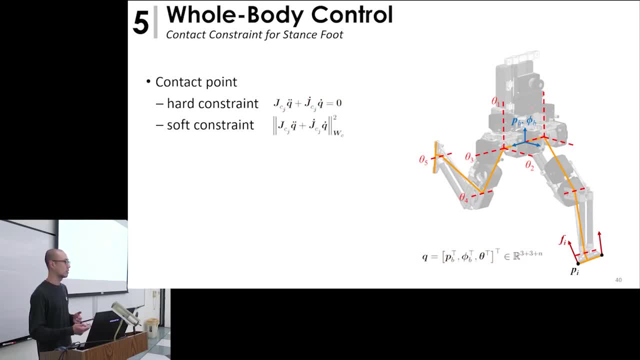 And in practice we can consider it as one of the operational space tasks. That is a soft constraint, because in this manner we can speed up the QP and have better numerical stability. Meanwhile, the contact force is constrained within the local friction cone, which is further approximated. 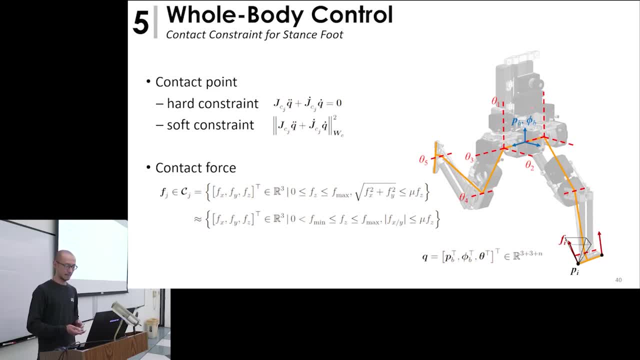 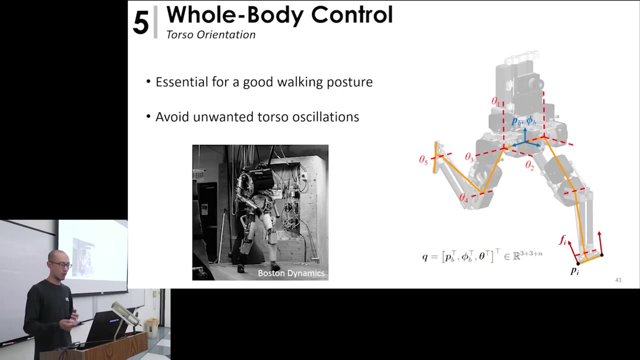 by a square pyramid. So we need to make sure that we have a square pyramid for linearity. So control the torso orientation is one of the operational space tasks because it is essential for a good working posture. Definitely, we want to avoid the unwanted torso oscillations. 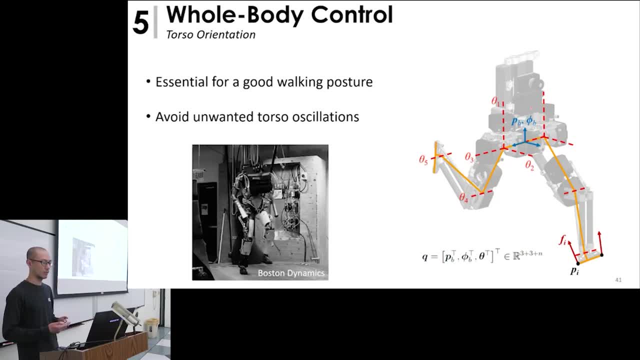 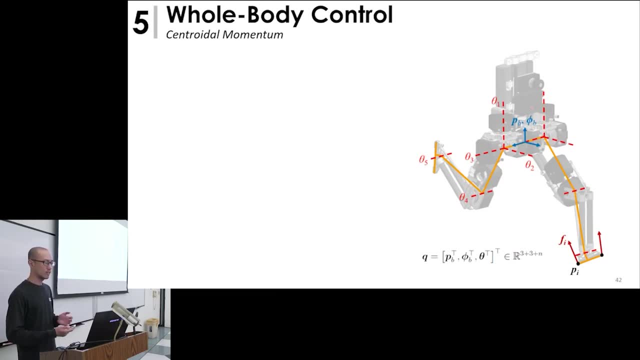 which can largely affect the motion and complicate the control process. And control- the central momentum is also a critical component of the QP. And control- the central momentum is also a critical component of the QP. And control- the central momentum is also a critical component. 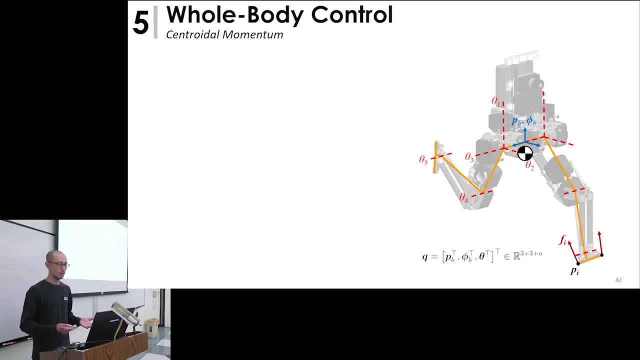 of whole body control. It contains two components: the linear momentum and angular momentum. The linear part has a straightforward relationship with the COM velocity, So in the vertical direction it simply maintains a nominal height to match the reduced order model. In the horizontal plane it's simply tracking the designed 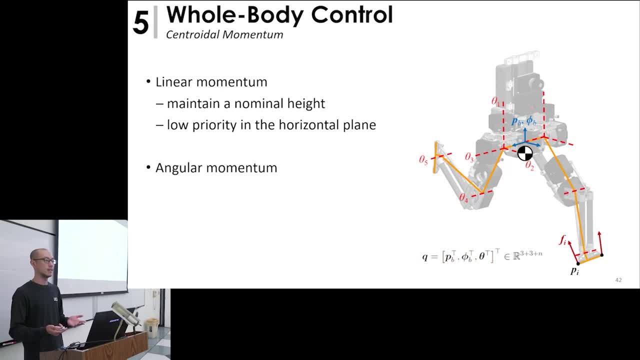 velocity with a low priority, because the robot movement is essentially realized by taking steps For the angular momentum. as we mentioned before, it is well-regulated to near zero for human working. So the task objective is just to damp out the excessive angular momentum. 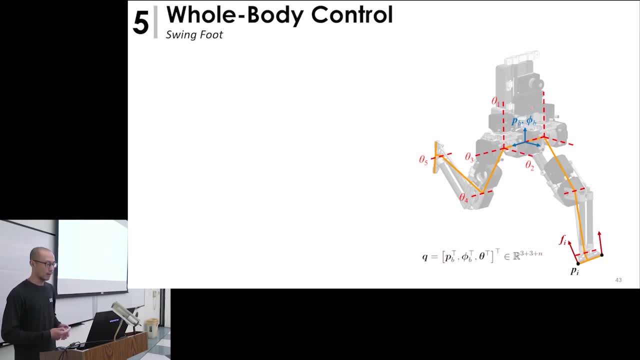 OK, so swing foot task. The reduced order plan is essentially realized by the swing foot task of whole body control And we need to consider both foot orientation and foot position. The swing foot orientation reference can be simply said- is set to some constant. 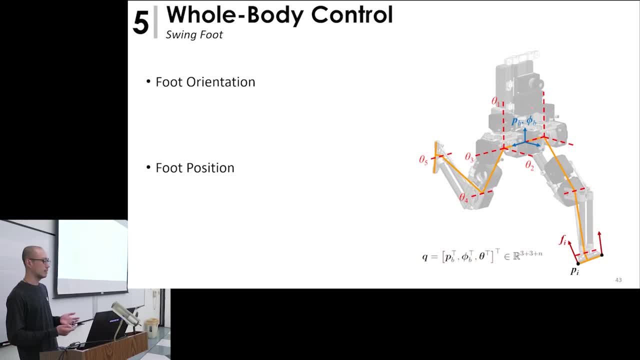 However, recall that each leg of Bruce has only five degrees of freedom, So the real motion is actually not controlled because it has the least effect for a line foot, And meanwhile the robot is actually working blindly with no terrain information. So the gain in the pitch direction. 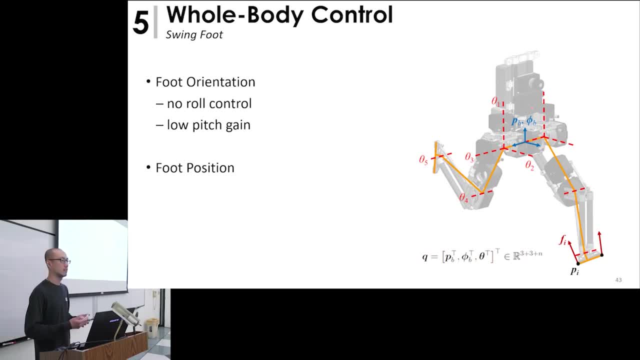 is intentionally set low, which can make the foot adaptive to a certain range of terrain, And the foot position trajectory needs to be carefully designed because it's in order to adapt the changing foot stand location and timing from the reduced order plan So, for example, in the horizontal plan. 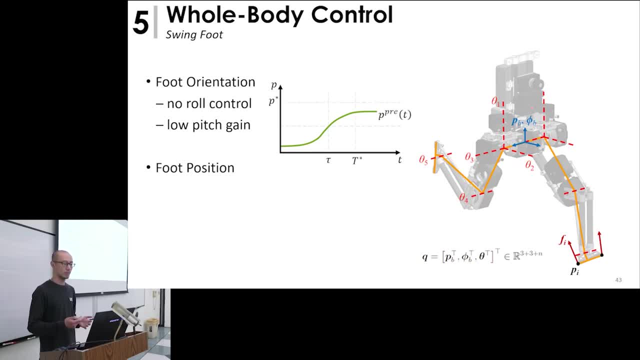 for at some time, tau, when a new step is planned with optimal solution P star and T star, the foot position trajectory is regenerated using a fifth order polynomial which to ensure the continuity up to the acceleration level, OK. And finally, during contact changes, 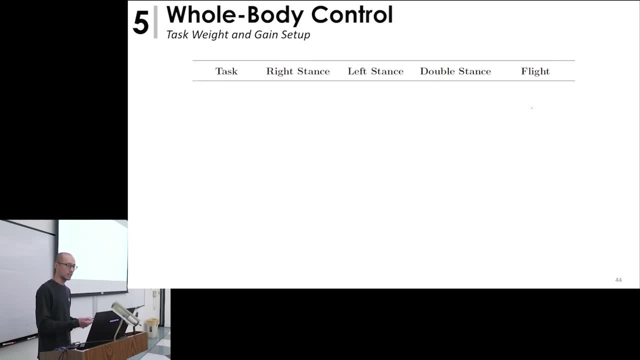 we also need to perform task transitions. This is, for example, the linear momentum cannot be controlled during the flat face right. And another example is when, for a stance foot, its stance counter constraint is activated while its swing foot task is deactivated. 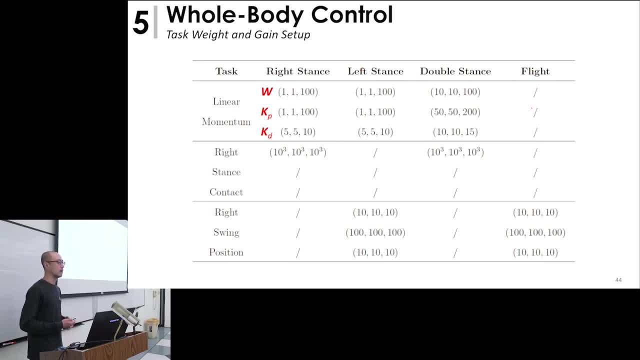 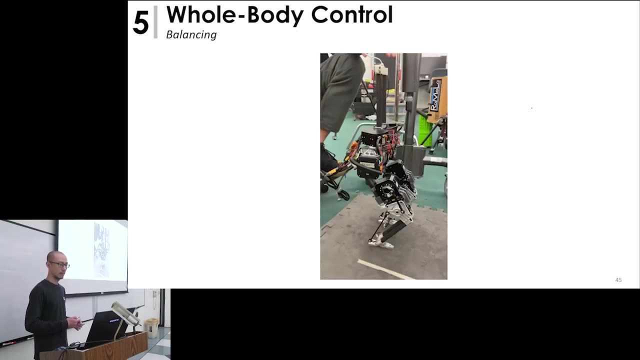 This can be simply handled by changing the relative task weight. For example, if a task is activated, task is deactivated, we can set its weight to zero And we can easily bring it back when it's become activated again. OK, so that's pretty much about our whole body control. 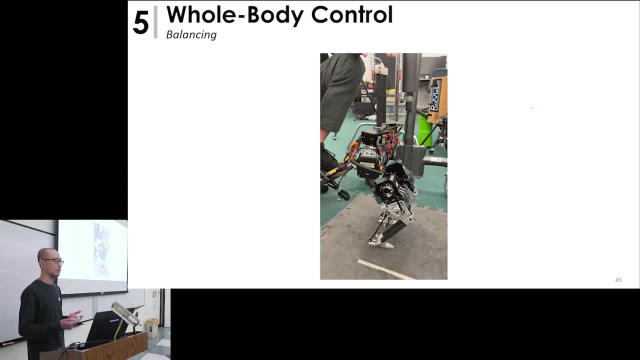 using QP, which can be solved in practice at 500 as well, ready for real-time feedback control. And before making the robot taking steps, we test its balancing performance. And here Bruce is trying to maintain its nominal standing posture with all constant reference. 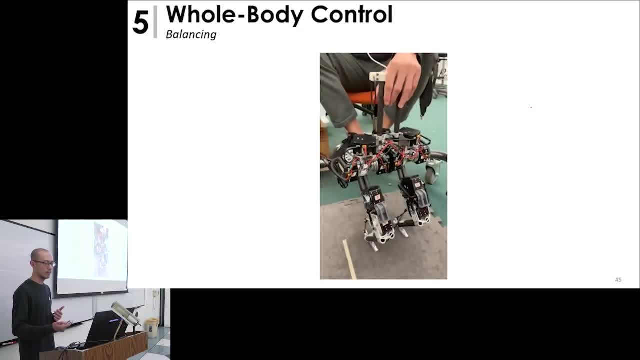 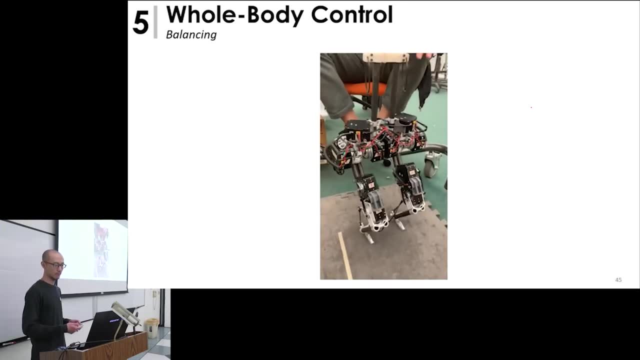 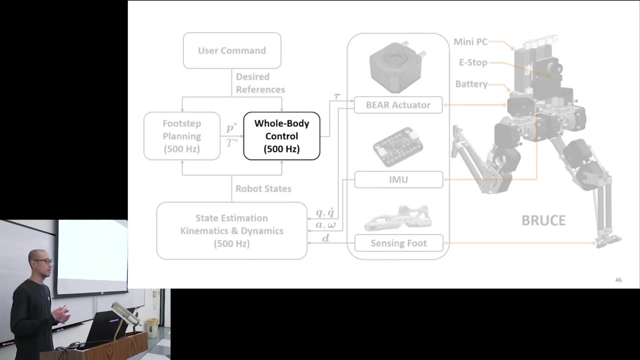 We can see, it can reject the disturbance pretty well in all directions And meanwhile it can produce very compliant behaviors. OK, so that's our whole body control. And finally, the control framework cannot be complete with a state estimation, So let's have a quick discussion on that. 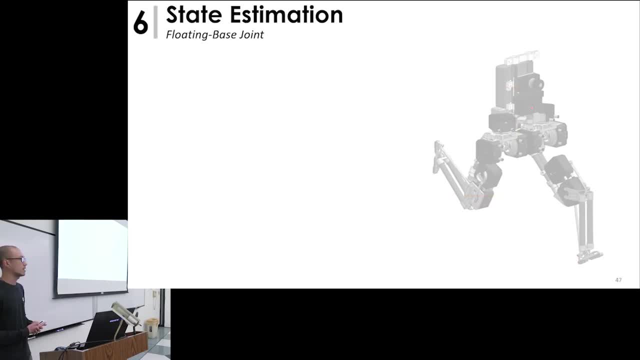 So for bipolar locomotion, an accurate estimation of the folding-based joint is of particular importance because it takes a lead in describing the system dynamics. And while common filter has been implemented in various forms, complementary filter works robustly, as we are in practice. 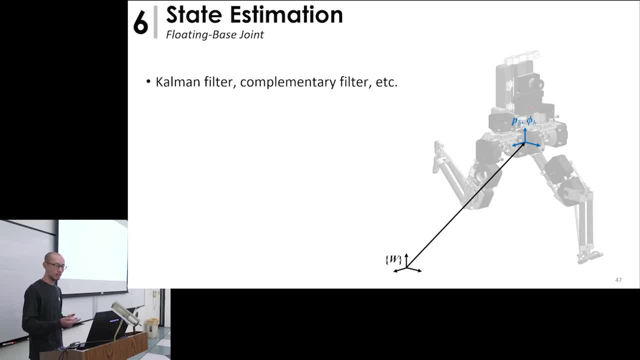 And, unlike other mobile robots, bipolar robot experience intermittent contact with the ground during locomotion, which suggests a unique function. OK, So this is a unique estimation approach by combining the onboard IMU and the robot genetic model, So in particular, the prediction model. 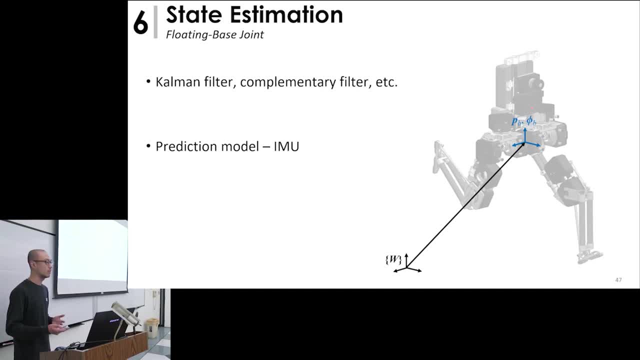 is based on the acceleration model, the acceleration measurement from the IMU, It's integration to get the base linear position and the velocity And usually the orientation information is good to use directly And whenever a foot is in contact with the ground. 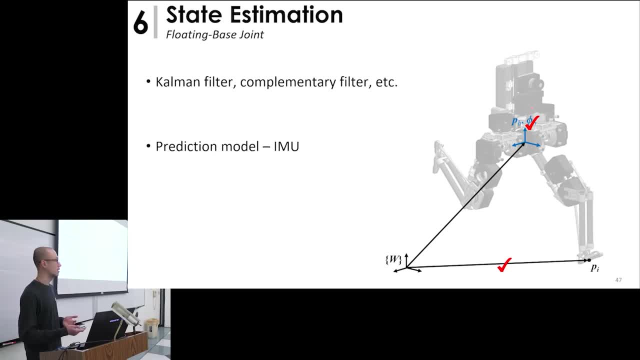 it's assumed to be stationary. But if the ground is fixed the velocity is equal to 0. And with that we can reversely calculate the base linear position and velocity using the Stan-Selec kinematics to correct the a priori estimations. 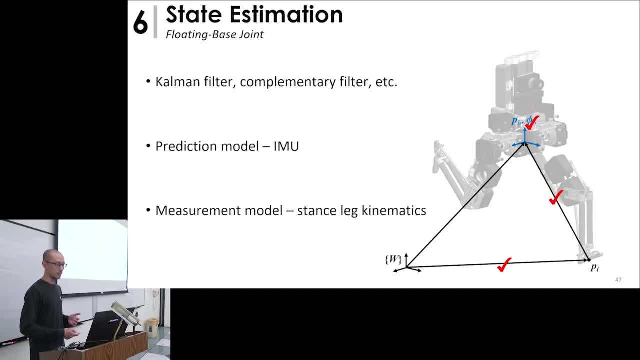 So this is how the bipedal estimation works, And once we have the estimation of the floating-based joint, we can add the joint information to derive the model for the entire robot And from there we can get, for example, the center of mass. 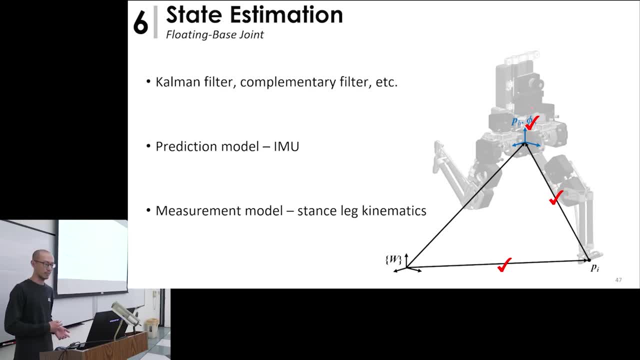 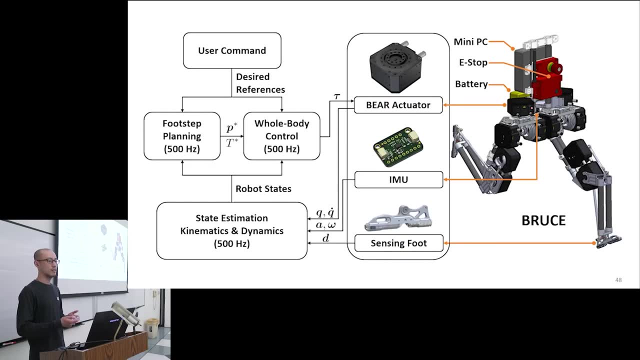 position and the velocity- OK. The swing-foot position and velocity, et cetera, OK, So we have covered everything. Now just combine them together, run the controller and make the robot move on its own, And extensive theories of simulation and hardware. 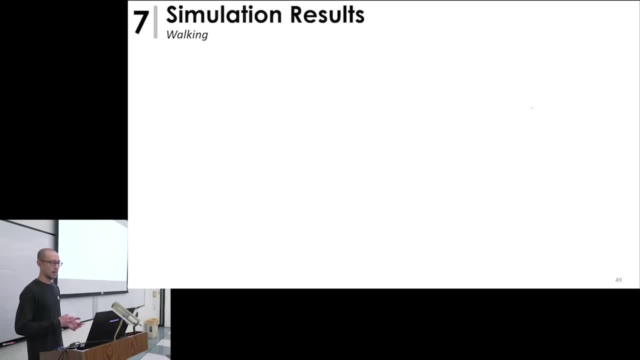 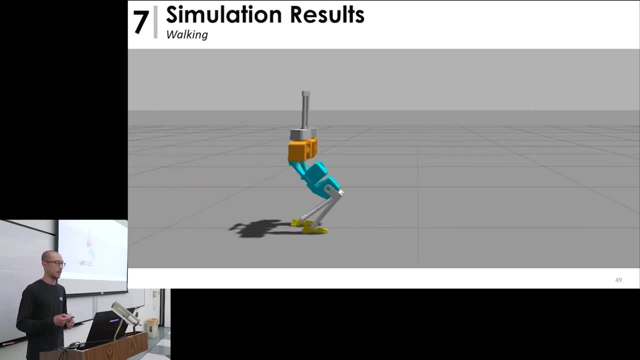 experiments were conducted. Let's start with the simulation result, And this one is working. where we do not consider a flight phase, There's no lag Nationally. The whole concept is the same And we will be able to connect it like this. 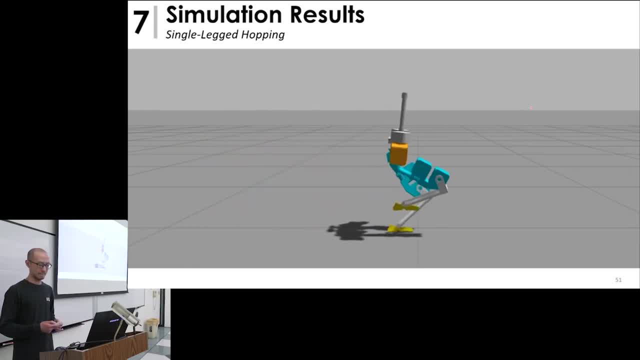 And we will be able to connect this to the robot With a non-zero flight duration. the robot is also capable of running And without alternating the two legs, if we just stick to one single leg, the robot is also capable of single leg hopping. 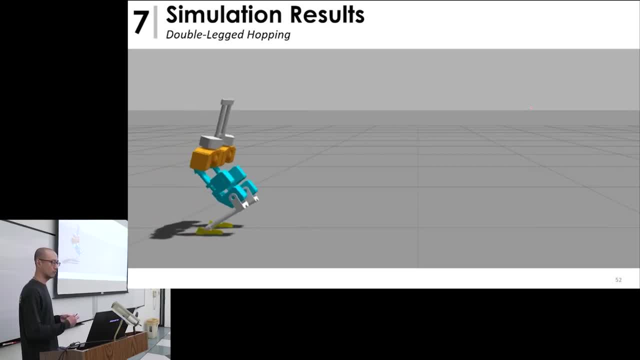 And then if we consider the control limits, for example, if we are able to mount a device to a single board, is a lot easier. Consider: the center of pressure. location is at the middle of the two foot. The robot is also capable of double leg hopping. 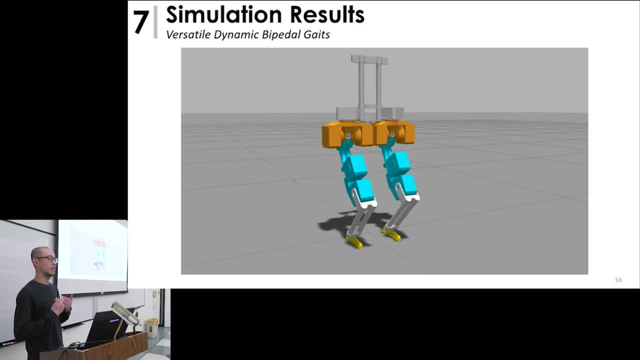 So that's just some typical bipedal locomotion gates. But our framework is versatile, as it is possible to generate any arbitrary bipedal gates by simply changing the nominal gate pattern. For example, we can have a clearance in the x direction. 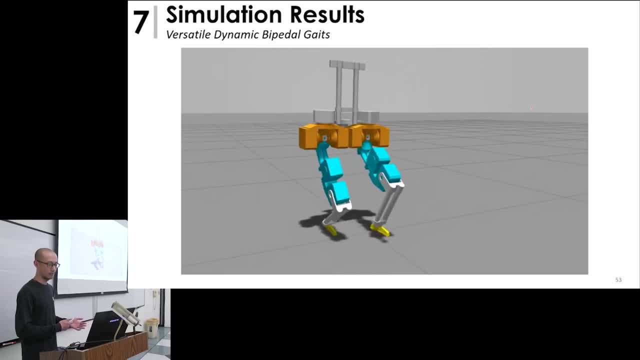 We can have a period of four gate cycles instead of just two. And if we just forget about the collision, the robot can also be capable of some fancy dancing motion. Now we can gauge the system in terms of disturbance rejection And, as we can see, the robot is able to recover within the next few steps after each push. 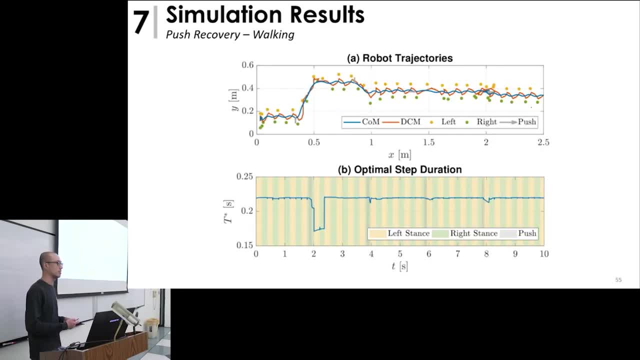 And here's the data. As we can see, the robot was adapting both footstep location and timing in order to prevent falling down Right, And this is exactly what we have seen in the reduced order simulation. We can also try to compare their static state trajectory. 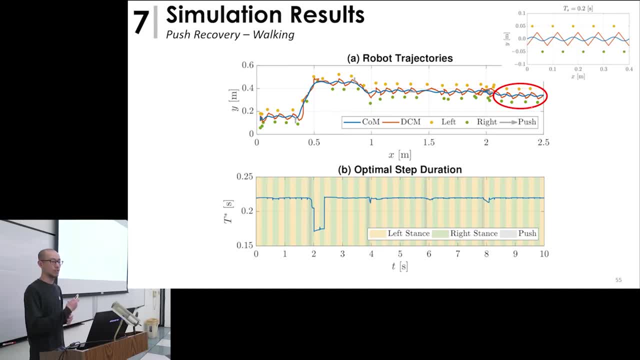 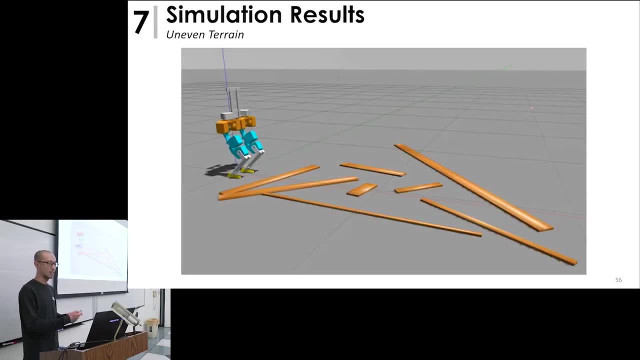 And, as you can see, they are actually very close to each other, which verifies our model simplification assumptions. We can also gauge the system in terms of turbulence, And here's the data, So we can see that the robot is able to cope with the terrain uncertainty. 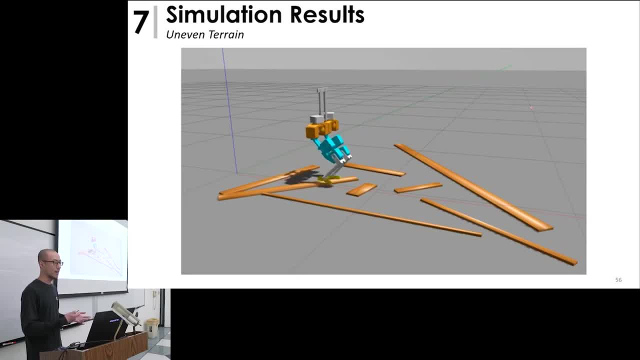 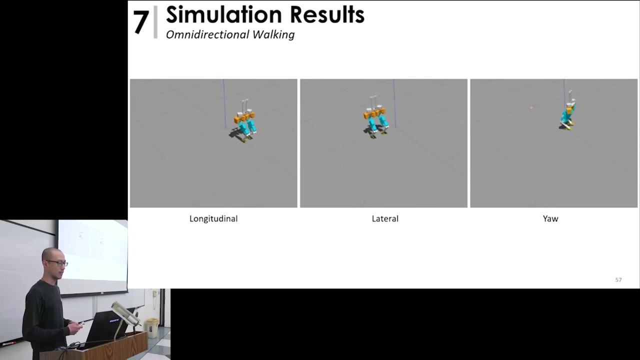 So we challenge boost on some uneven terrain. While the controller is assuming the ground is always flat, it can still handle some ground height variation And of course it's not just stepping in place or forward, It can produce omnidirectional changes. 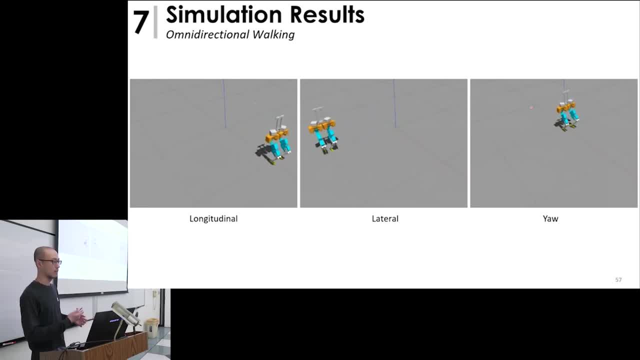 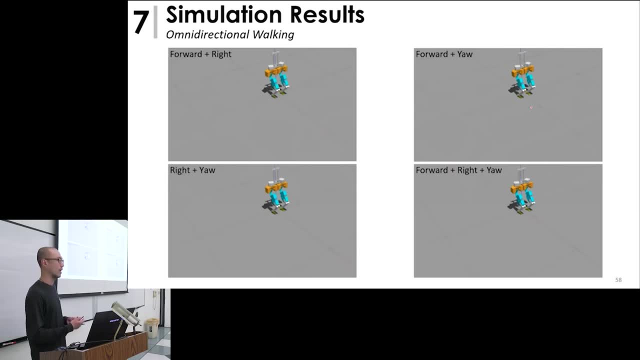 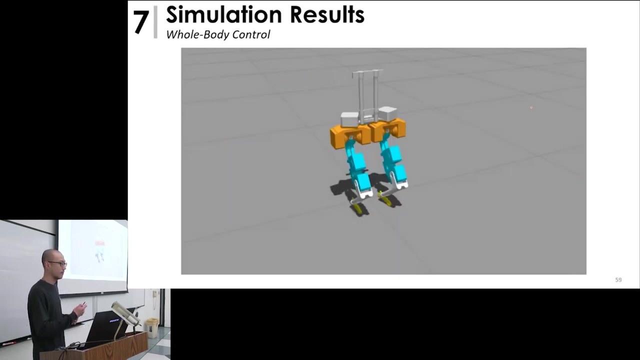 formidirectional working, forward and backward, left and right, and also self-rotation, And from there we can have any combinations of these fundamental motions. And finally, I just want to illustrate how many times our whole body control is regulating at the same time. 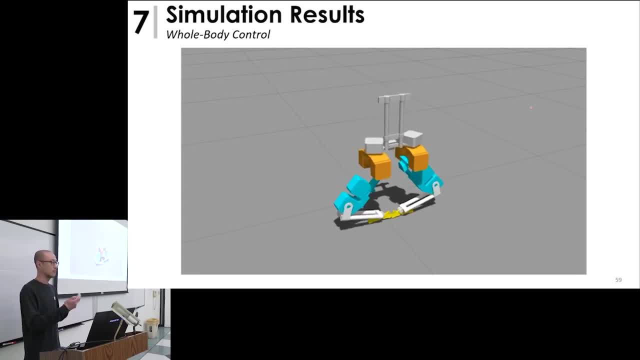 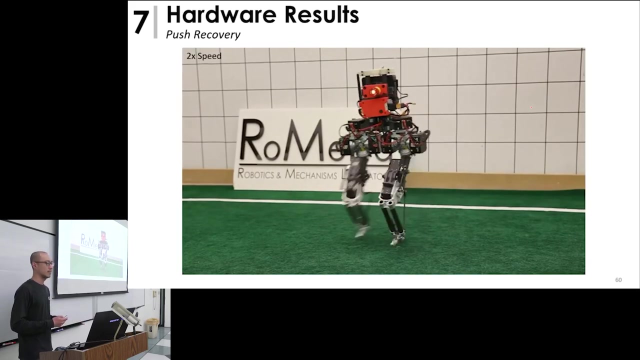 So the first is, of course, the foot orientation, the center of mass height, the foot clearance and, of course, the torso orientation. So, as you can see, our framework can still handle this, this configuration, So the working controller is also implemented on the real physical system, a similar push. 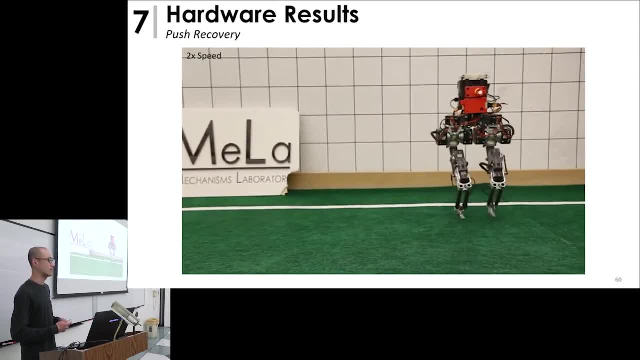 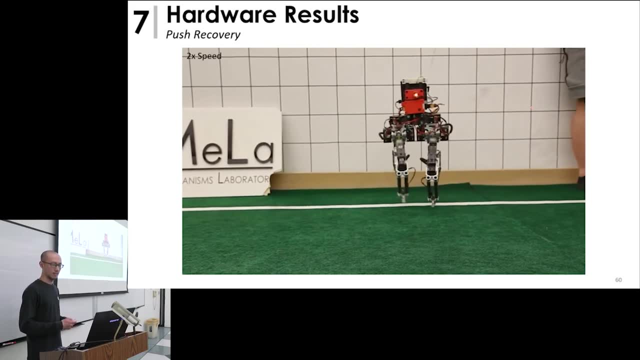 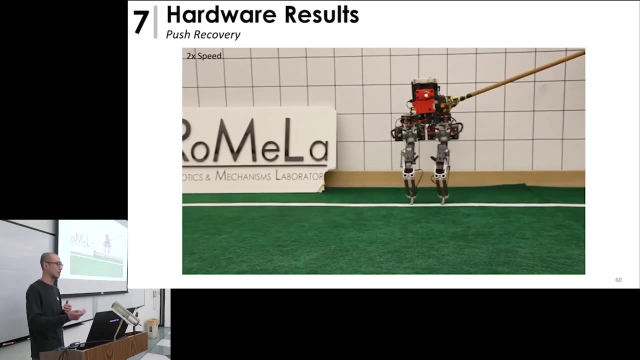 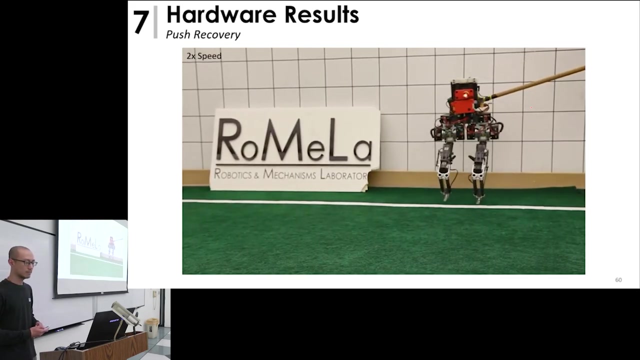 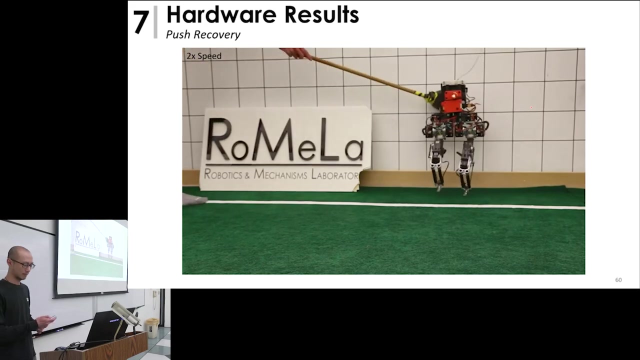 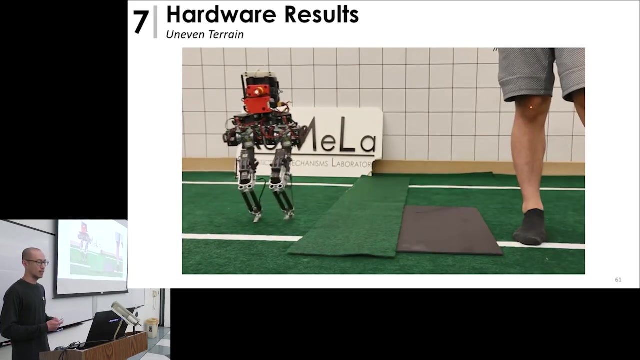 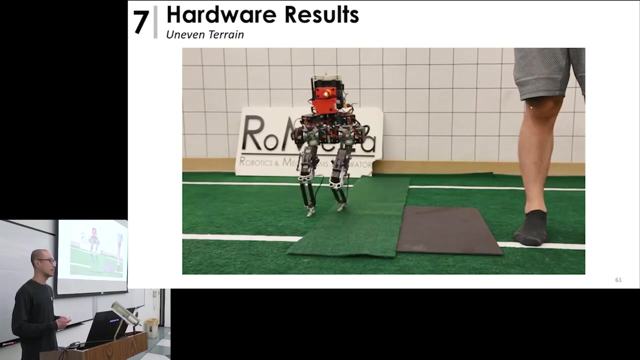 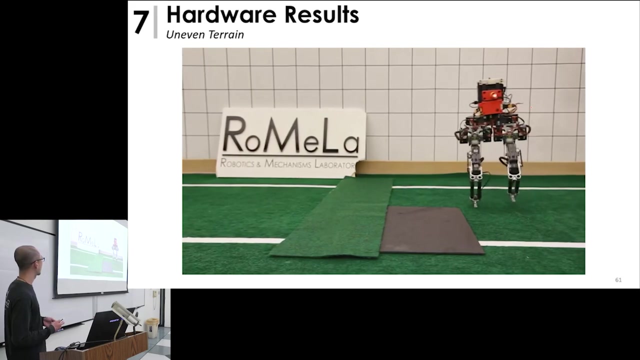 recovery test was conducted, where we push robots in different locations, in various directions and with random time and random duration, and the robot was able to manage and to survive. We also challenged our robot with several irregular terrain. This one is uneven, where the robot was able to work with some ground height variation. 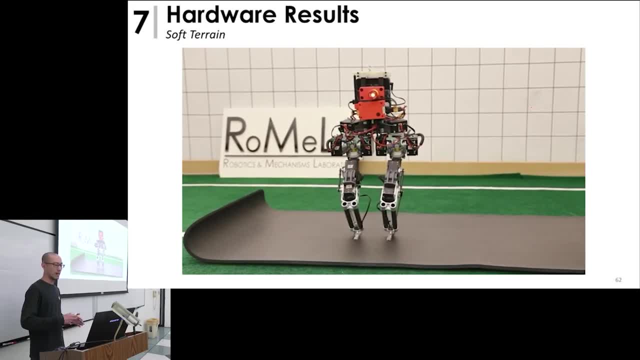 And this one, Bruce was actually stepping on some yoga mat. And this one, Bruce was actually stepping on some yoga mat. And this one, Bruce was actually stepping on some yoga mat. This kind of soft terrain is challenging, as the stance field cannot keep stationary. 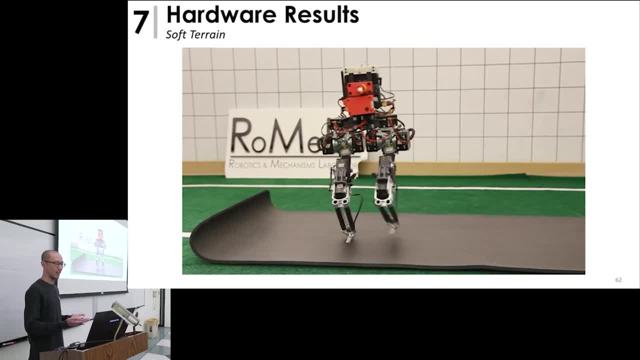 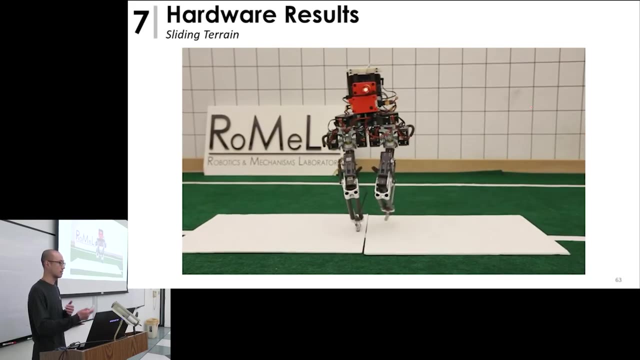 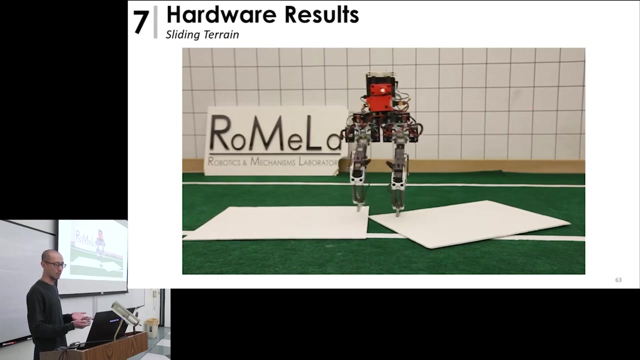 which can easily cause oscillation or even instability of the system. However, our controller can still handle that. And this one Bruce's robot was actually stepping on some foam boards which can easily slide on the ground. The sliding can also mess up the estimation, which assumed fixed contact. 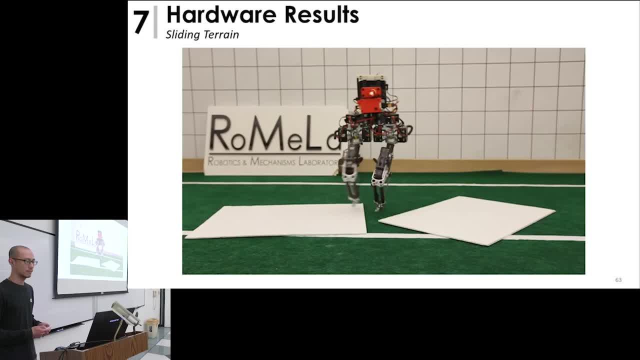 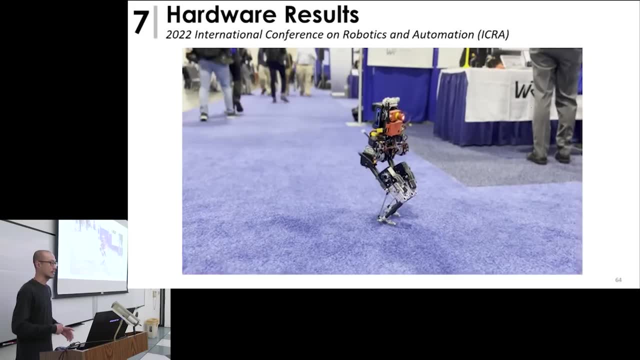 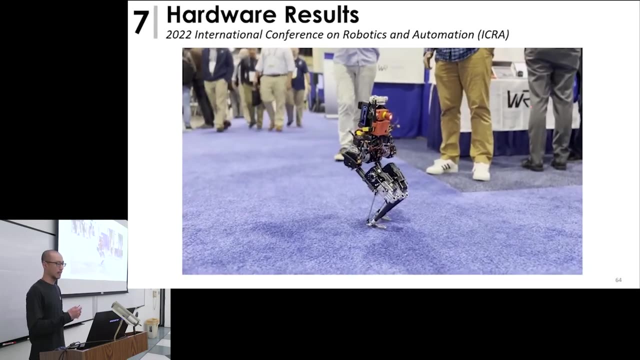 But our framework can still handle. Yeah, the system is robust enough. We were very glad to bring our robot to an international conference in Philly this May And it was a huge success. You know people just loved Bruce because it's so cute when he's doing the stepping. 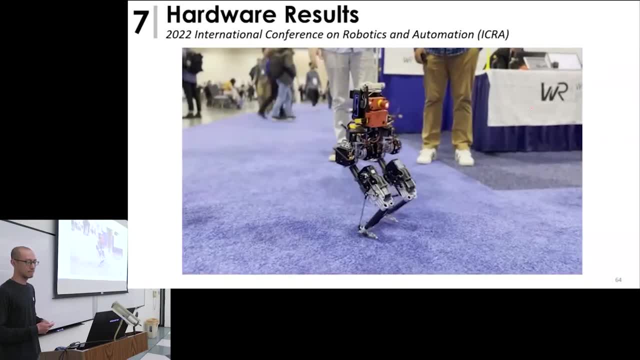 Think of that. Look at this. Maybe this is the head of the group, The head of the group right, So that we have a robot that's with a head of a robot that can fly, like that. So that's pretty much about it. 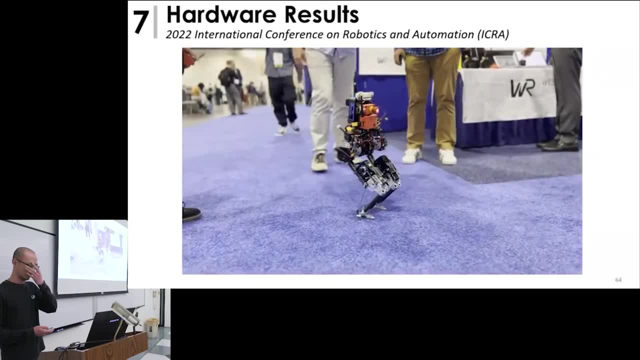 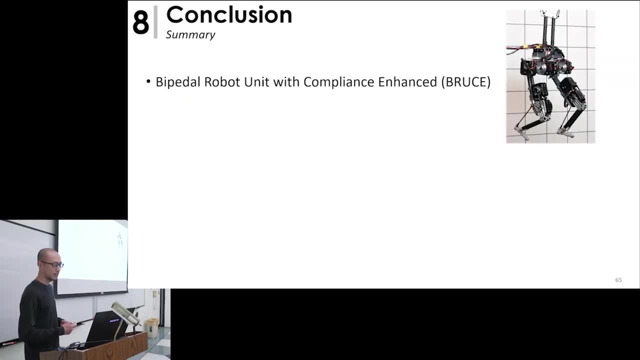 Let's have a quick summary. In this augmentation, Bruce, the next generation miniature bipedal robot is being under development, in specific the cable-driven differential pulley system, And you can see that it allows us to control it by using our hand-operated device. 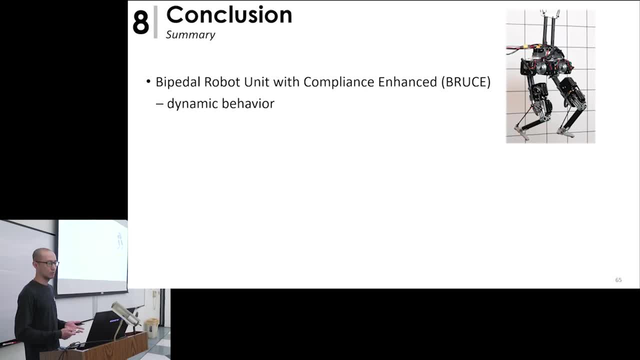 system and the linkage mechanism were designed to reduce the leg weight and inertia, capable of a dynamic behavior, and meanwhile, proprioceptive actuation is also equipped on the robot for compliant interaction with the ground. and second, a dynamic bipedal locomotion control framework is being proposed, where the high level plans the footsteps and the low level 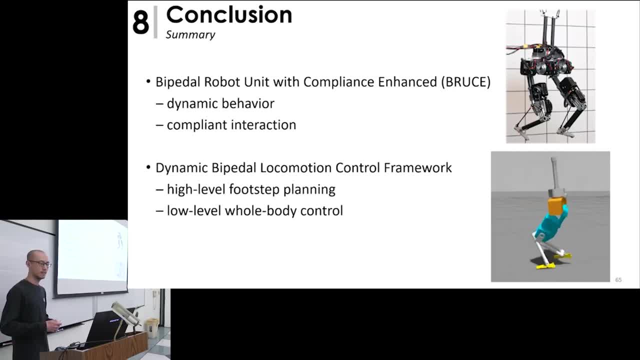 controls the whole body motion while establish the full contact, as planned, which is capable of walking, running, hopping gates, etc. and here's some major contribution of this adaptation. first, as the blue system is reliable and cost effective, we are working on making it an open source platform for the robotics community where, in the near future, which we envision- 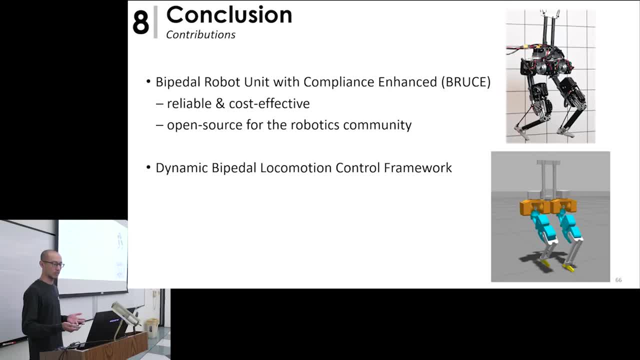 can boost the studies of humanoid robots. as for the locomotion control framework, previous works only concentrate on the working scenario. our framework extends previous works by further constraint of five feet, which is capable of a much wider range of bipedal gates and wherever you design the locomotion. 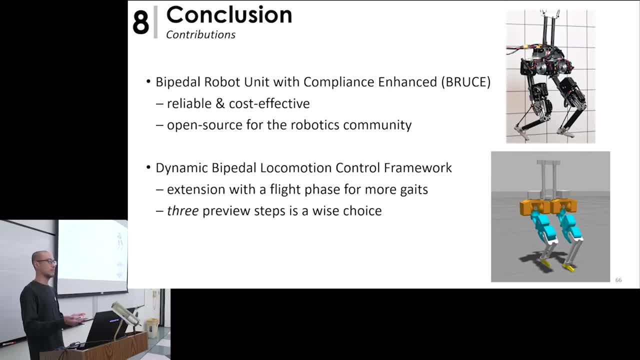 bipedal locomotion control. you always ask the question: how many steps ahead should we plan? while previous studies only consider a preview of adequate steps in order to ensure the system viability, our results indicate three previous steps is enough, and it is actually a wise choice in terms of system robustness, transient behavior and computational efficiency. and last but not the 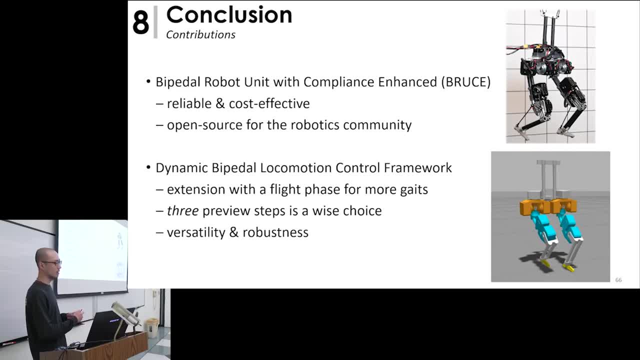 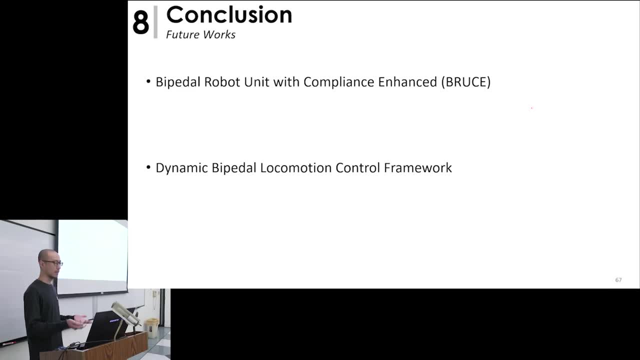 least, an extensive theory of simulation and hardware experiments were conducted to demonstrate the versatility and robustness of the approach and in the future an upgraded upper body with arms will be actually bruised for more capabilities, for example, standing up on its own local manipulation, etc. for the locomotion control framework realizing 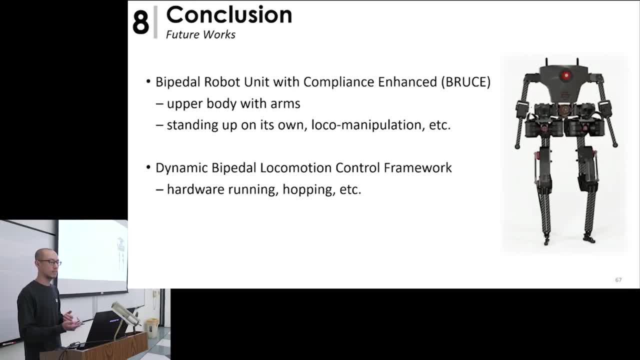 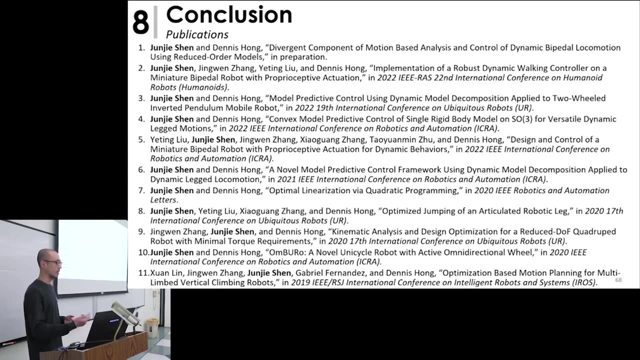 the running and the hopping gates with the physical system is also on the future list and meanwhile, with an upgraded upper body, unassisted locomotion can be invested for for stronger robustness. and here's the publication list, and these five papers are the most relevant to this. 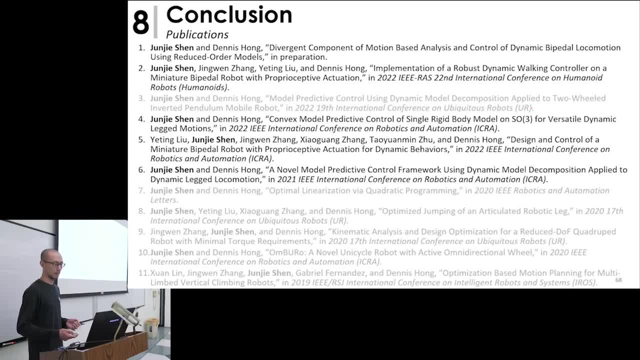 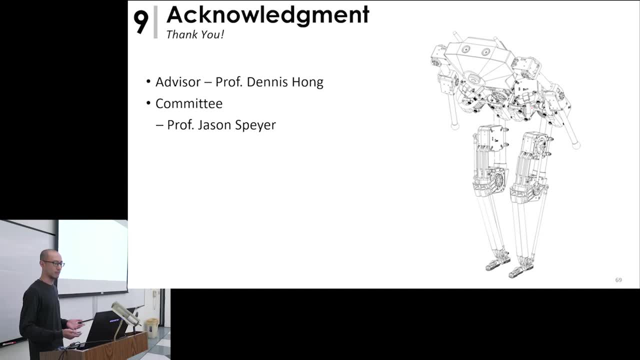 dissertation. yeah and yeah. finally, i want to say thank you, first to my advisor, professor hong, and to my community member, professor spire, professor iwasaki and professor hopkins, and to anyone who, to anyone who is a part of my lab romila, and, of course, to 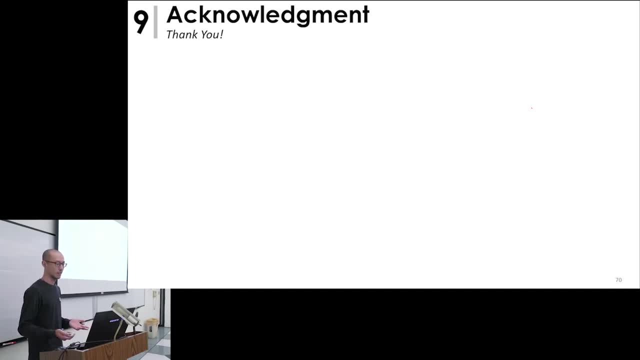 my family and friends and, last but not least, to my boosting, because this, this dissertation, is impossible without your help. uh, because, uh, i cannot do this all alone by myself, in particular every nick hulkery team and me. so it all starts three years ago, when we have only a 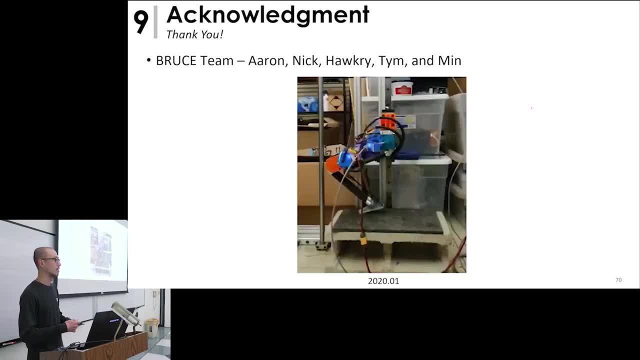 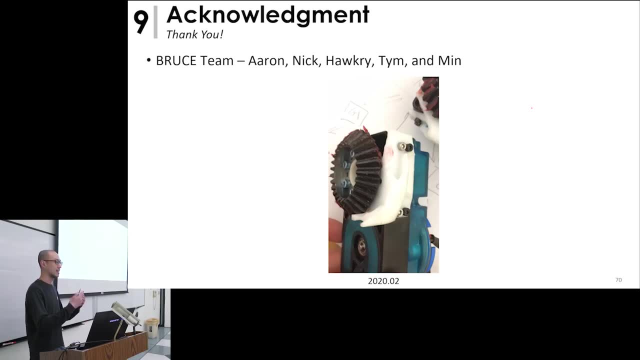 simple, simple concept and at that time we only have a very easy 3d printing lag which can easily break from time to time. and then the pandemic cam. everything was delayed, but at that time we were thinking about we need to change the double gear and the conclusion, as you know, is the cable. 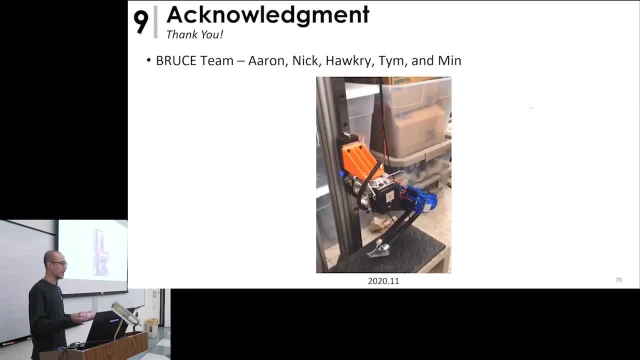 pulley driven system and with that our boost, the lag can finally make its first jumping- and of course, some other concepts we'll cover later, but i think i'd like to thank you for joining us today for the presentation and we'll see you in the next video. 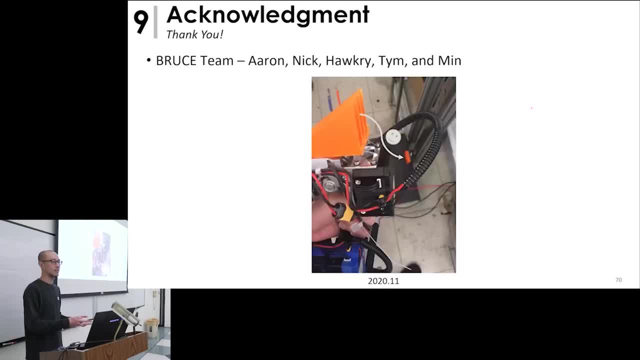 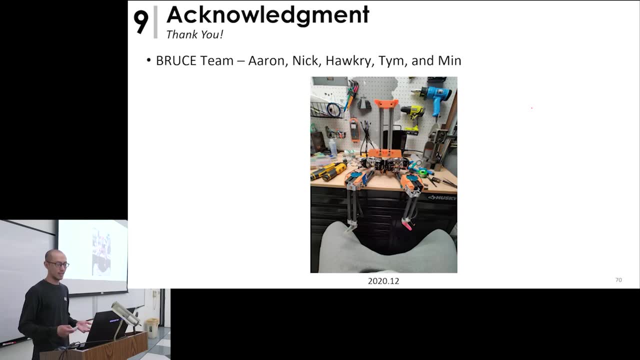 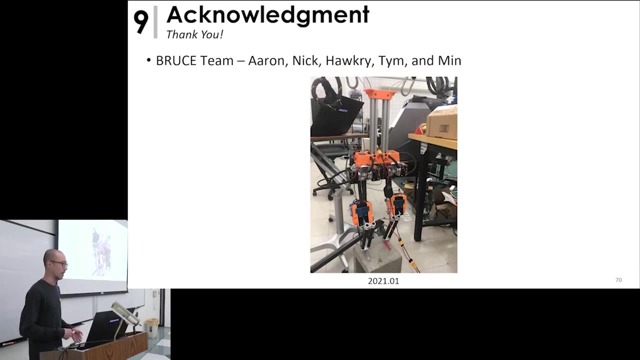 thank you for watching and i'll see you next time. the 3D part can break from time to time, but it's fine. and once we have enough test with a single leg, we finalize the design and build our first version of Bruce. a month later, Bruce can stand on his own, yeah, and then we 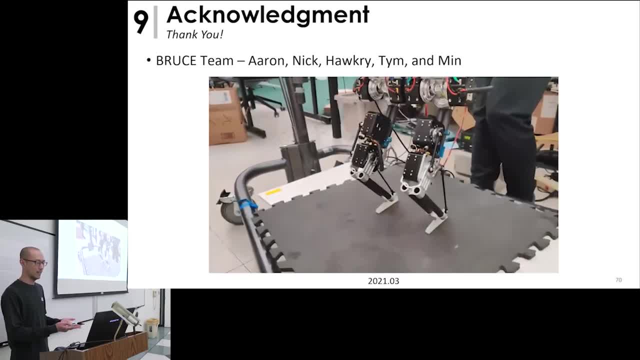 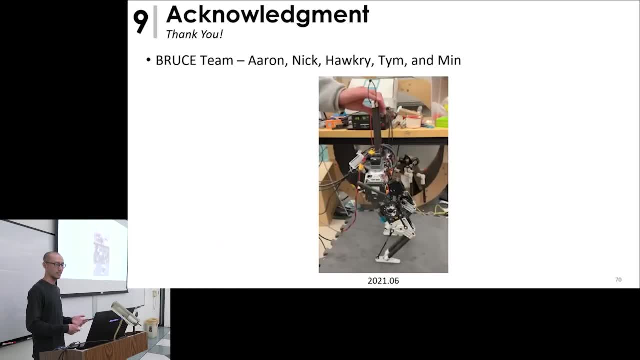 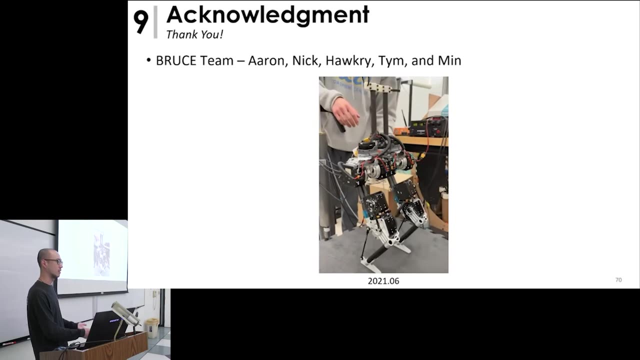 just play with the robots. this one, as you saw, it's a seesaw balancing to verify the kinetic model and this is robot control. but at that time, as you can see, the dynamic model is not accurate enough. the control frequency is pretty low. the games are not well tuned so the performance is kind of weird. but 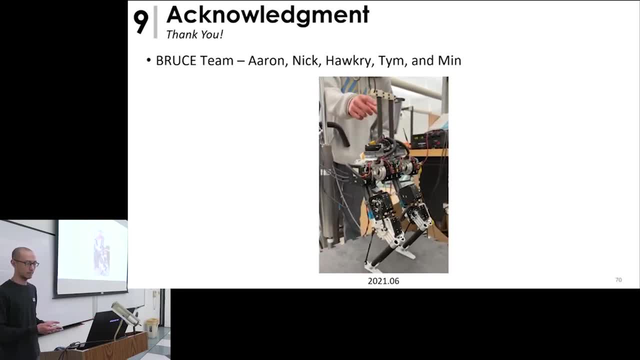 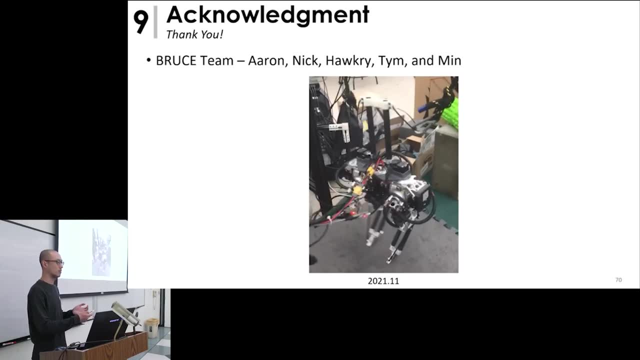 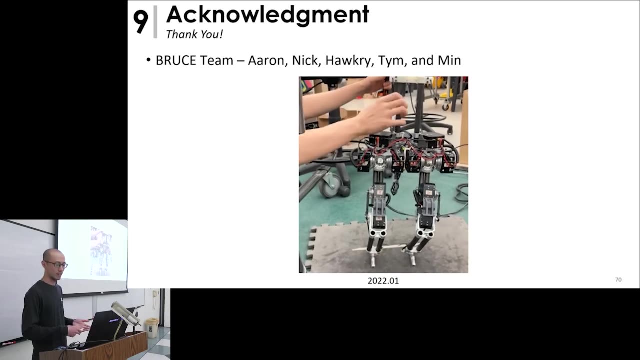 you know it's doing something. and then we just study the locomotion. we first test an open-loop trajectory, you know, just to feel the robots, to see how it will behave, and we just start testing this current framework at the beginning of this year- and, by the way, this is for Bruce first. 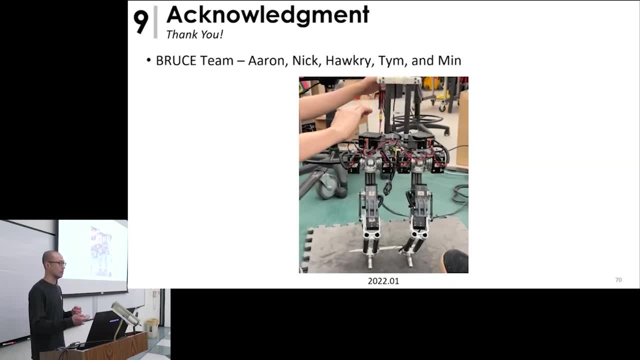 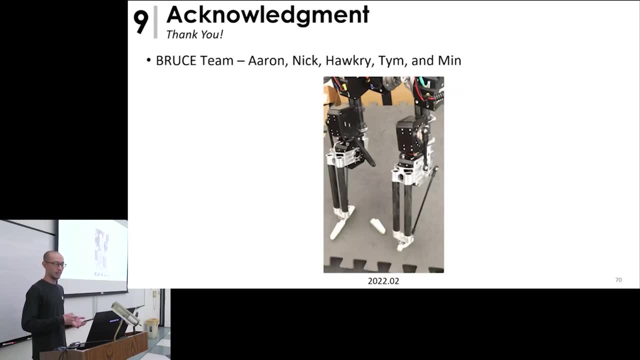 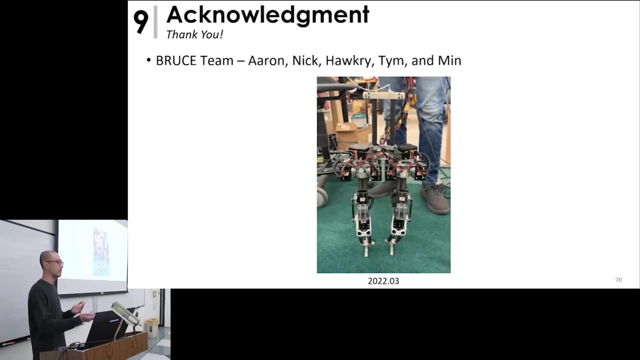 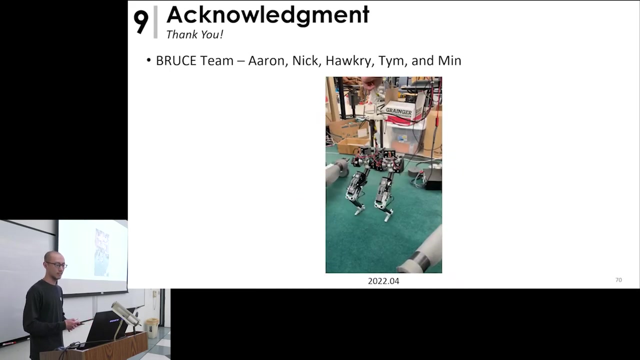 step. and just when we try to add more steps, apparently there's some bugs in the code- the robot went crazy and break its foot, and a month later Bruce can make 10 control walks. and after that we just you know, kept increasing the steps, kept breaking the feet and eventually we have something close. 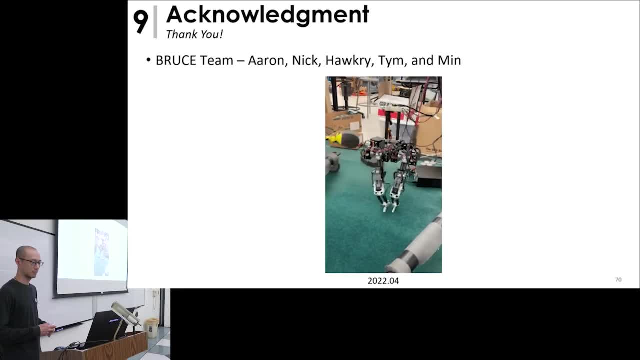 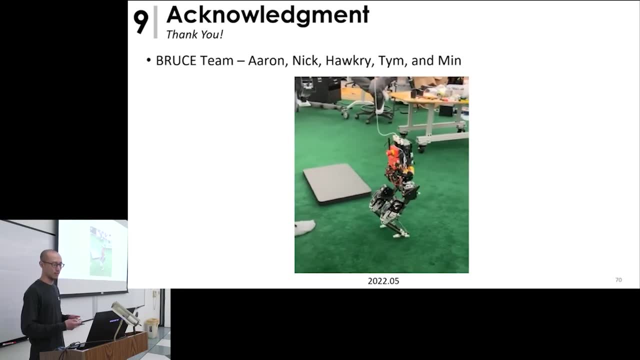 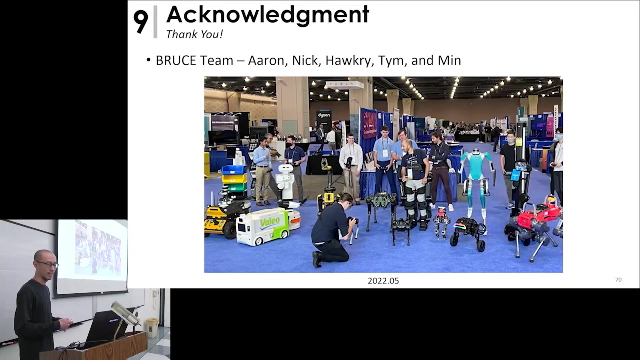 yeah, and Bruce went fully untethered this May and the controller, you know, was more or less finished and it was just before our trip to the conference where Bruce made its debut, surrounded by all the big names you know, uh, Boston Dynamics, Unitary, uh, animals, agenda, robotics, yeah, and, by the way, Bruce was here. 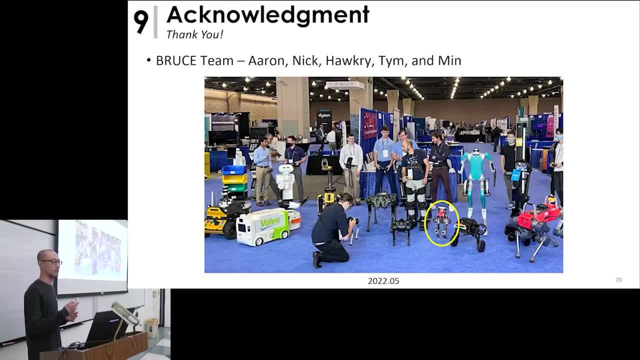 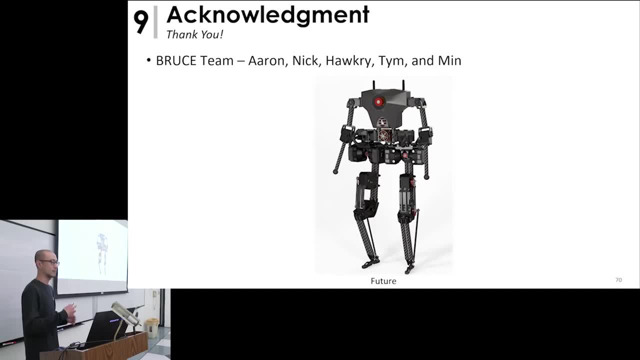 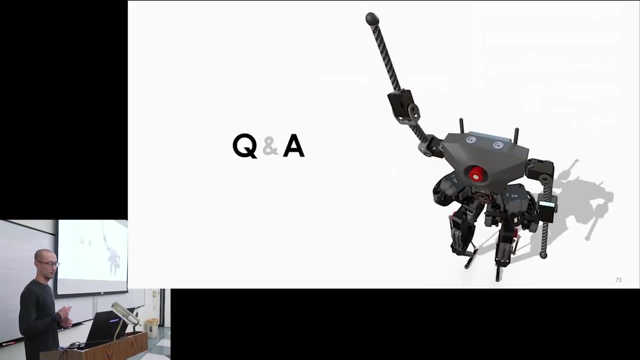 and that concludes and that ends the story of Bruce, chapter one, because I believe this is just the beginning of start. this is just the beginning of something big. we see a lot of potential in this robot, so stay tuned, everyone. and with that I'm ready for Q&A. thanks for listening. 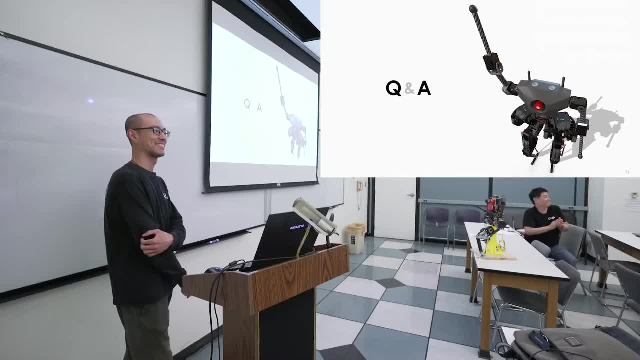 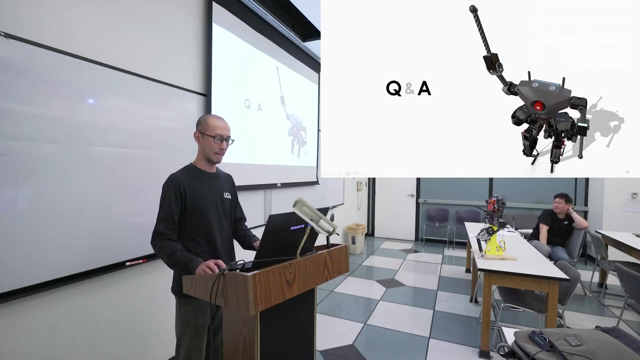 thank you very much. let's uh, we're gonna open up to the audience for any questions or anybody on the Zoom. if there's any questions, I'll hear you. yeah, are you open for questions? is that the point? yes, I'm open for questions. okay, hey, tell me about the. 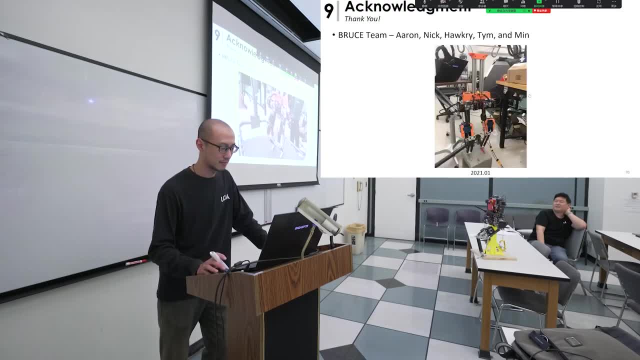 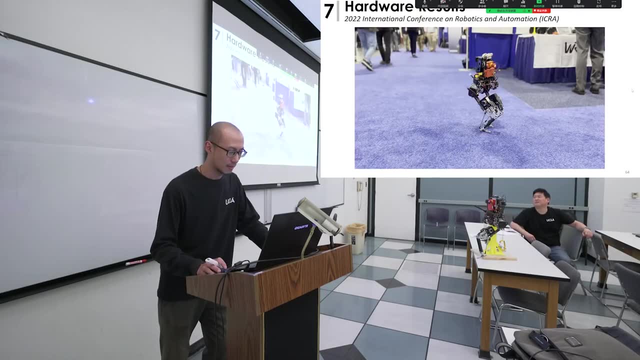 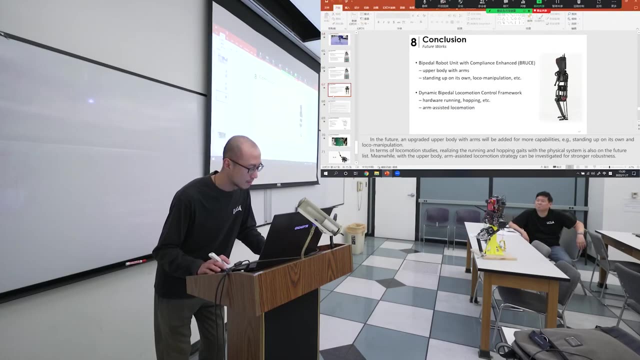 uh, IMU. um, yesterday, in terms of IMU there's a drift. uh, do you have any problems with it? uh, in terms of balance, so in terms the IMU, yeah, yeah, very small. yeah, usually the IMU, uh, yeah, usually, if you just integration of the acceleration. 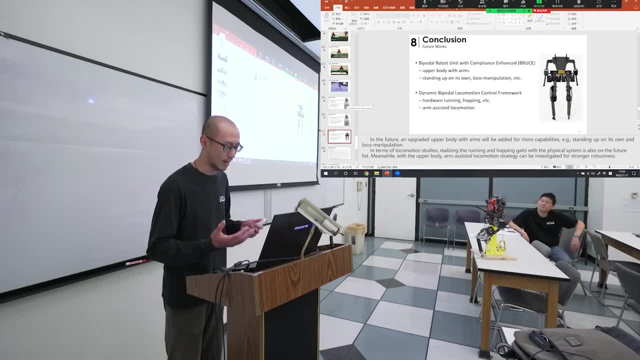 you will have drift. but you know, we also correct the estimation using the stance, like in the kinematics. so it works pretty well. you correct, you calibrate it. but no, we correct the April estimation using the robot kinematic model. so when the food is in contact with the ground, the contact point, 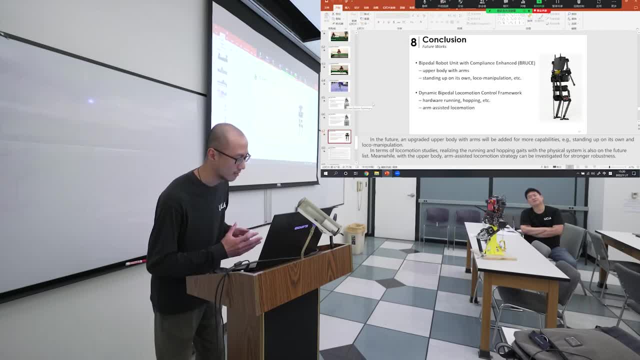 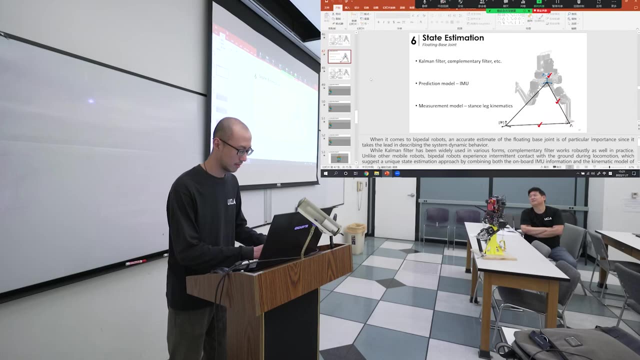 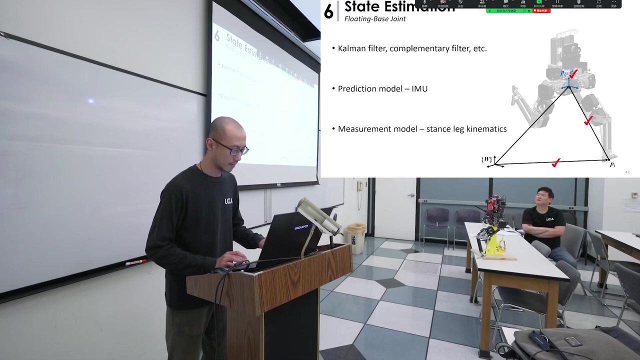 is assumed to be stationary, so we can inverse, reversely calculate the base position, position using the using the robot kinematic model. I'm not sure what you're saying. are you sure? are you saying you, you correct the IMU somehow, is it? is it a recalibration? or is it just the, just the calculation of some of the biases, or what? 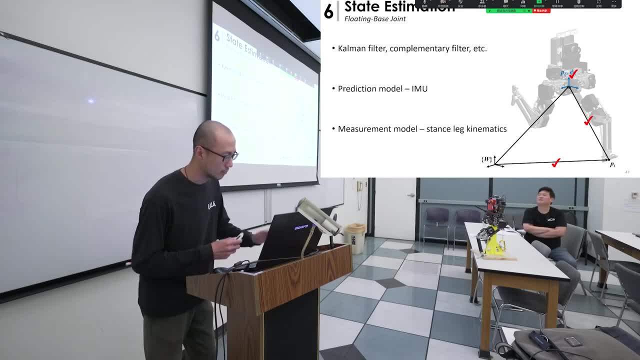 uh, we are not calibration, the IMU. so the prediction model is using the IMU, you know, integration- to get the velocity and position, and then the measurement model is using the It's dense, like kinematics, So we can correct the IMU drift Because when a foot is in contact ground, the contact location can be assumed stationary. 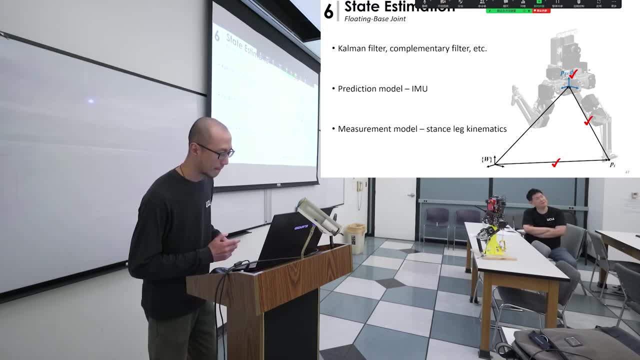 Okay, so if the IMU is an error, you correct the IMU because you know where the because the foot is in contact with the floor. is that right? Yes, The contact location is assumed to be fixed. In a sense, you are calibrating the IMU, right. 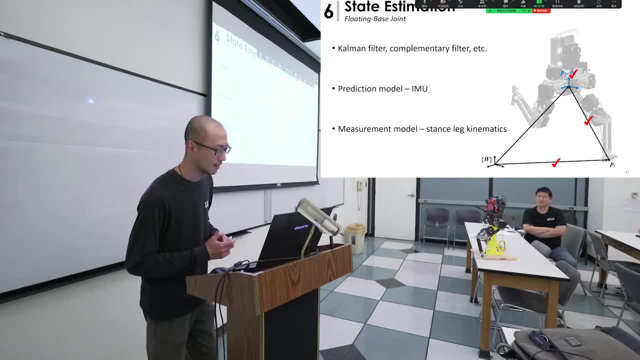 Yes, Okay, By using that. so that's one way of calibrating it, But that's. is there any problems with attitude or things of that sort as well? I think it works pretty well in practice. yeah, But you're saying it drifts. 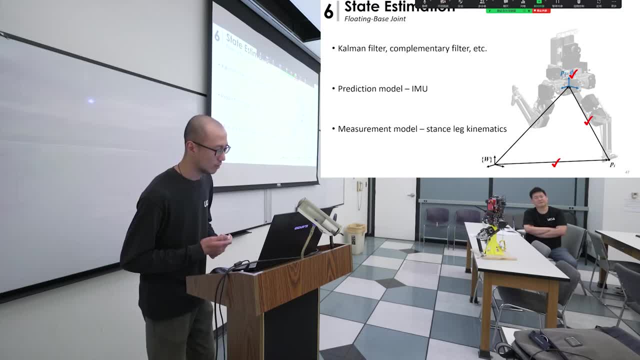 What is the kind of the drift like? Yeah, So, as I said, if you're just using the IMU integration it will drift, But you correct, with the lag kinematics it will not drift. Well, that's just. you know. I mean the drift. you know you have accelerometers that can. 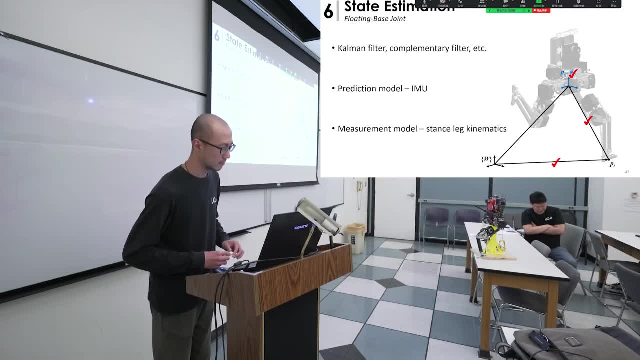 be drifting. You have gyros. that drift. That doesn't correct at all, does it? Does it correct the attitude and things of that sort as well? Oh so the attitude you mean? you mean the height of the robot, The yaw. 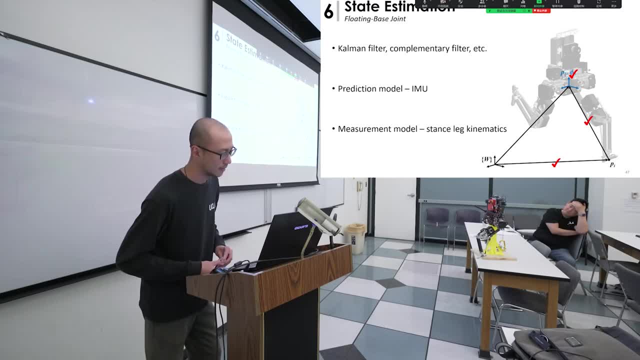 The yaw of the robot, The pitch, the roll, the height sort of part of the. Yeah, usually the pitch and the roll will not drift. because, yeah, usually the roll and the pitch will not drift, The yaw will drift a little bit. 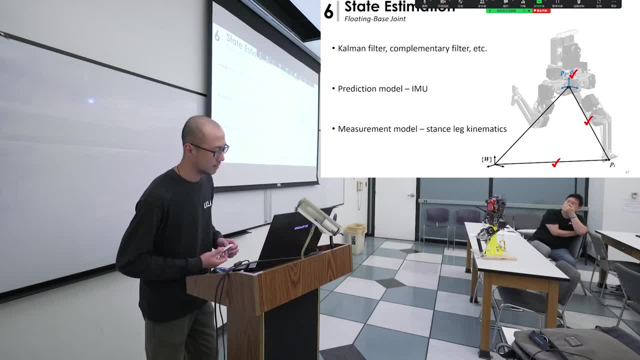 But yeah, Okay, Why doesn't? why doesn't pitch and yaw roll not drift? Because you can. yeah, so for the orientation part, you can, either using a very expensive IMU, they can calibrate for you so the roll and the pitch will not drift. 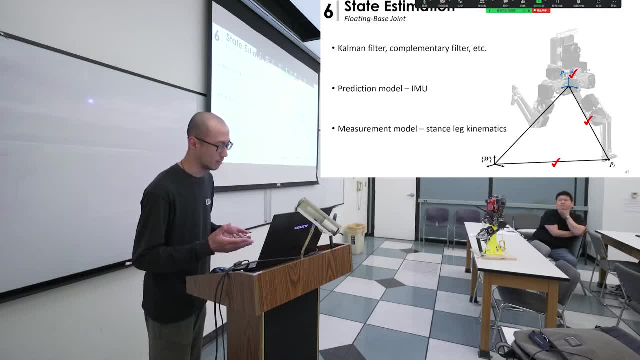 You can also try to do it yourself. For example, you can using the acceleration, because the acceleration Okay, So if the robot is assumed have a low acceleration then then you know it's always pointing downwards. Then you can use the acceleration measurement to correct for the pitch and roll as well. 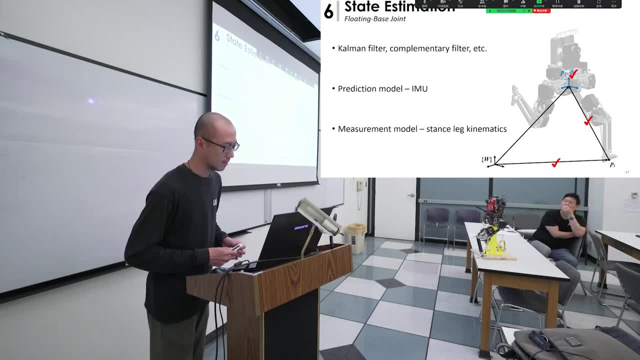 And so all of that is basically implemented in your robot, right? Yes, Everything is implemented. Yeah, But it's just too much detail so I didn't cover everything. Yeah, It's a lot of detail, Too much detail, Yeah. 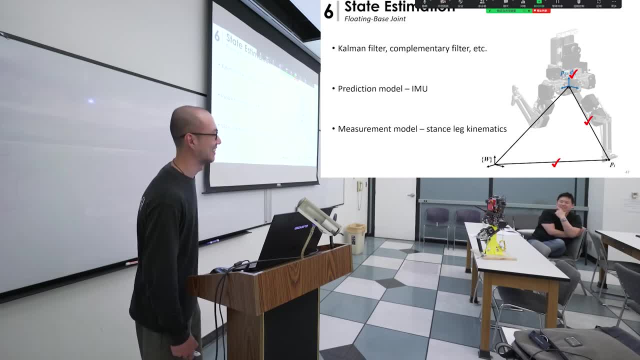 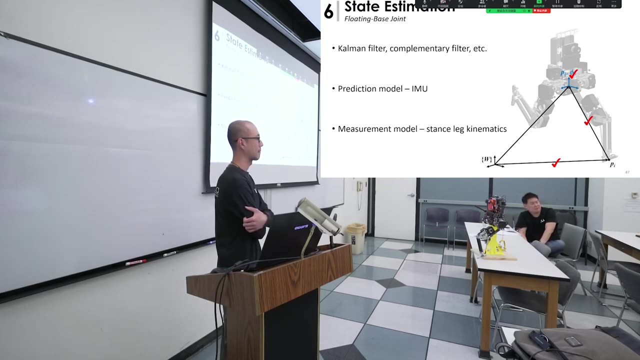 It's a whole laboratory of detail. Yeah, Yeah, Yeah, Okay, Okay, You're good, Cool. Any other questions from the audience? Yeah, Thank you for presentation And we asked a question about, like the structure for your overview of the boost, like the upper. 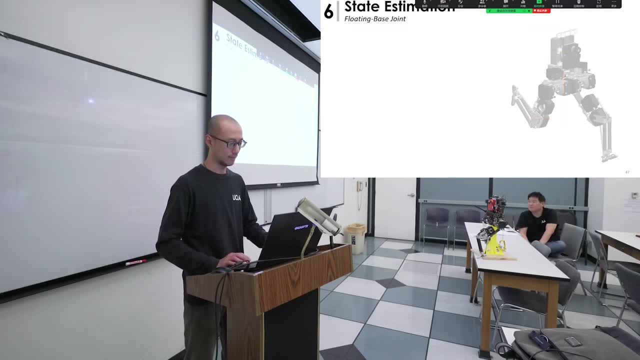 level control and low level control for the footstep. Yeah, This one, Okay. So, like, as you mentioned, the high level is footstep planning, right, Yes, And the low level is the whole body control. But I just wonder like the frequency for these two controllers are seemingly the same on. 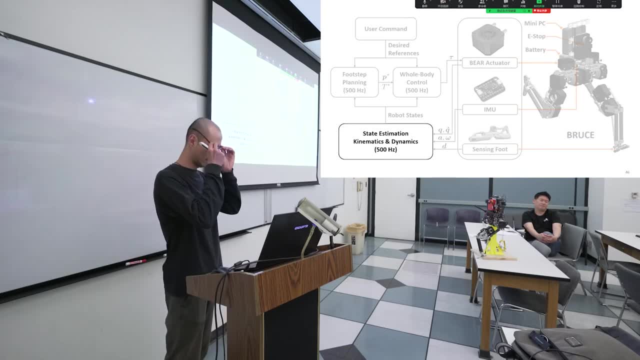 your presentation. I don't know. like maybe for the low level control should it be a little bit higher, like the frequency should be a lot higher than the, you know, the upper level controller, so that the lower level controller can actuate the command completely. 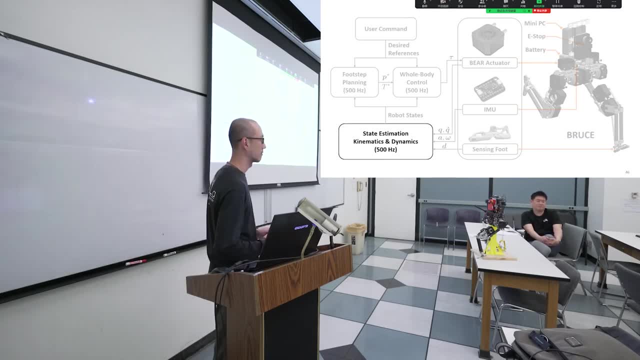 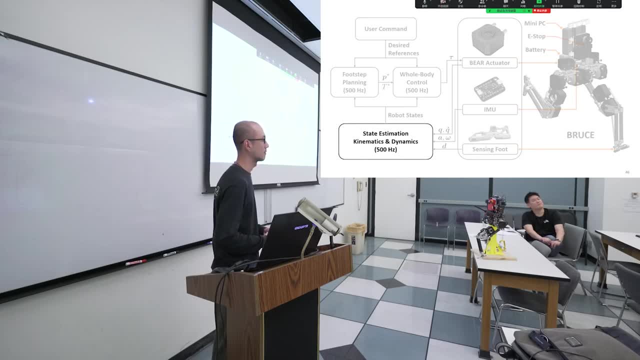 I mean before getting another command from the higher level control. So, uh, I just wonder what you just set it up to be the same, or? Yeah? Yeah, I know your question. So thank you, Yeah, Yeah, So usually in the footstep planning you can set um, you can try to have, let's say, the 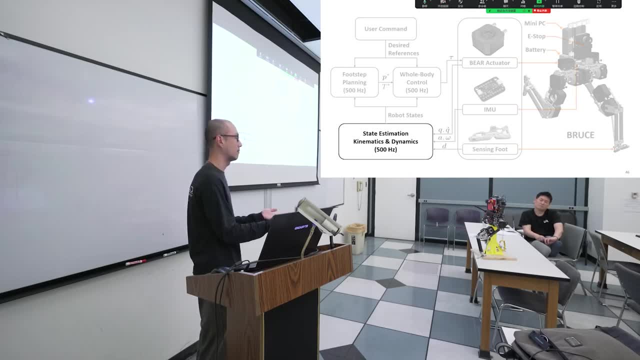 100 bars, Maybe it's good enough, But of course, the faster, the faster, the faster it is, the better you can recover, right, Yeah, Yeah. So that's the reason why we want to have as fast solution as possible. 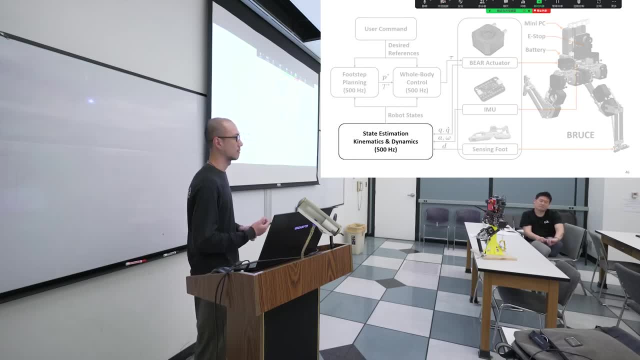 So the higher level frequency cannot be greater than the frequency for the lower level control, right, Yeah, so if it's greater than that, then the low level cannot actually catch all the information from the panel plane. Logically, the whole body control. the lower level you have, the higher frequency you should have. 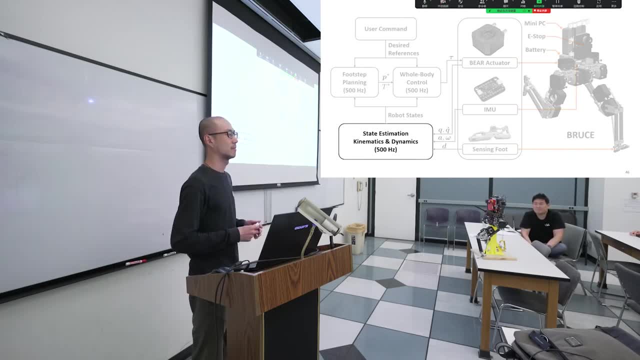 Thank you. Can I ask one question? Yeah, go ahead. So does the whole body control also control the swing foot, or not? Swing foot is just like kinematics. Yes, yes, So the whole body control controls everything, also the swing foot. 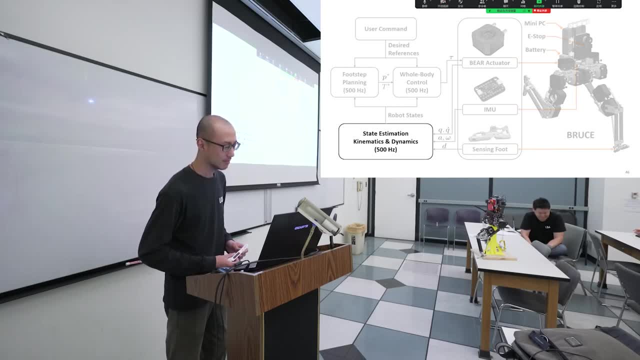 So, since they have the same frequency, so you plan one foot step and then you control one time of your body motion in your main loop. Oh, yeah, yeah, So it's the same time for controlling both the foot and the orientation. 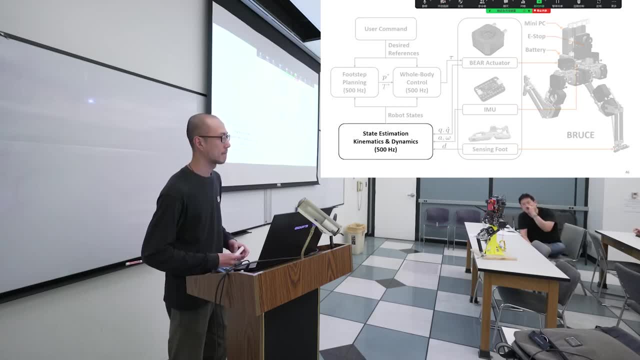 Okay, We miss you, Shen. Yeah, Hi, how are you? This is my former brother. Yeah, Also, he's not very happy. Okay, We'll talk about it later. Okay, Sorry, Thank you, Thank you. 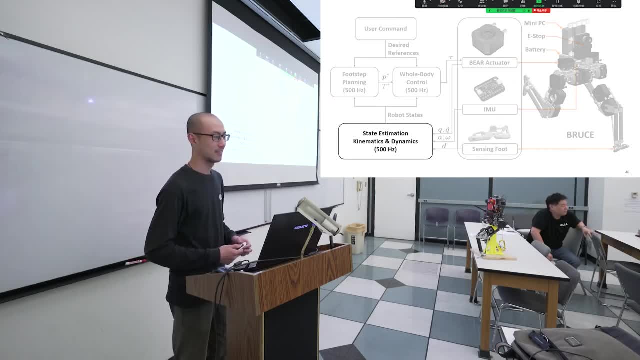 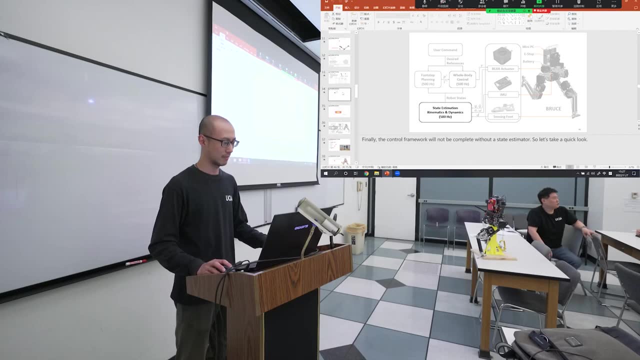 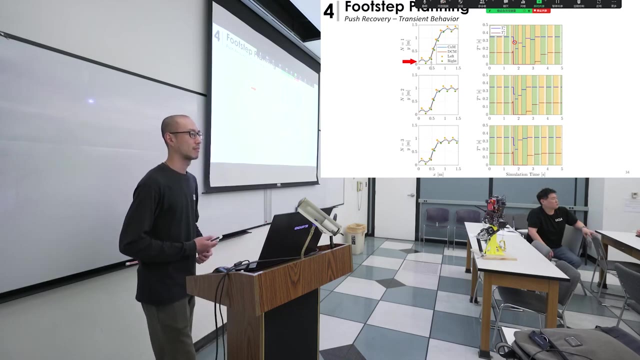 So I think you said three-step prediction is beyond three steps. You didn't see much performance increase. Yes, And regarding that. so I have a question about that. One is: what's your metric of performance? Oh, the metric of performance. 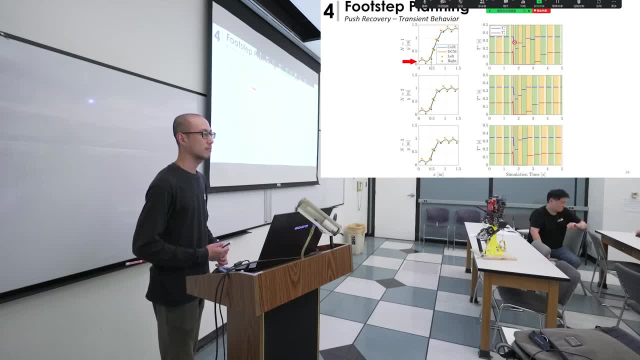 Yeah, yeah. But what are you looking at to say, oh, I'm not seeing much. Second is: so all this is based on some nominal height, some nominal mass, where they were in the Yes, Is that correct? Yes? 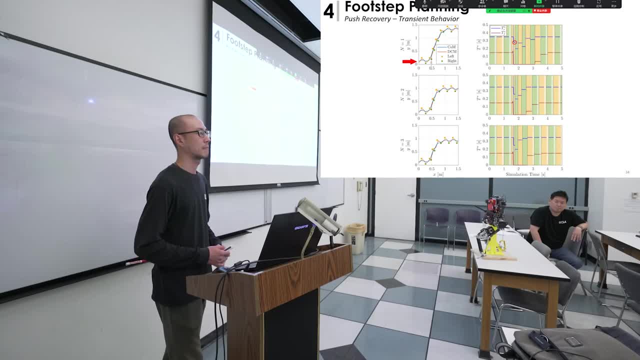 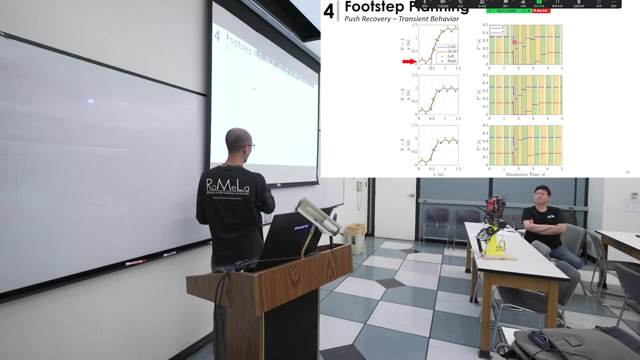 So, depending on the height difference and the mass difference, can that number, do you think that number would change? First one is for the metrics. So I say three steps is a wise choice in three perspective. The first one is for the training behavior because, as you can see first, as you can see the trajectory is, the robot can recover faster and the trajectory is more close to its original path. 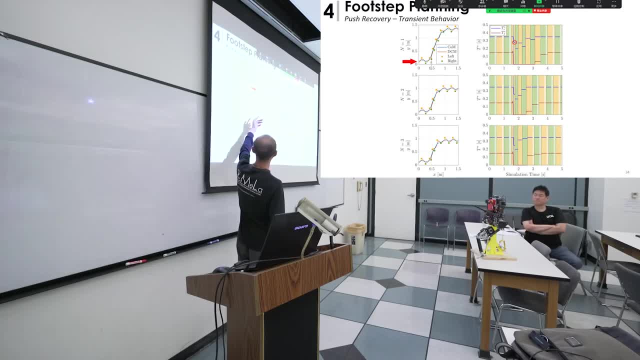 And from n equal to 1 to n equal to 2 is. the improvement is very significant From n equal to 2 and to 3, and you can see it's only a little bit. Yeah, You can also try to for n equal to 4,, 5,, 6, they're almost the same as n equal to 3.. 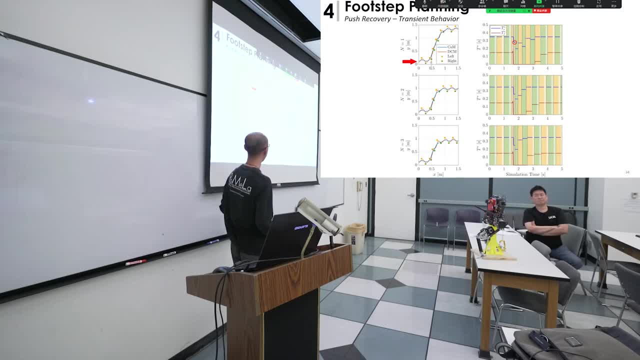 So that's why I say it's kind of converged to something. And this is always for the training behavior, and also it's the same thing for the optimized phase generation. As you can see, it's more or less the same, It's converged to something. 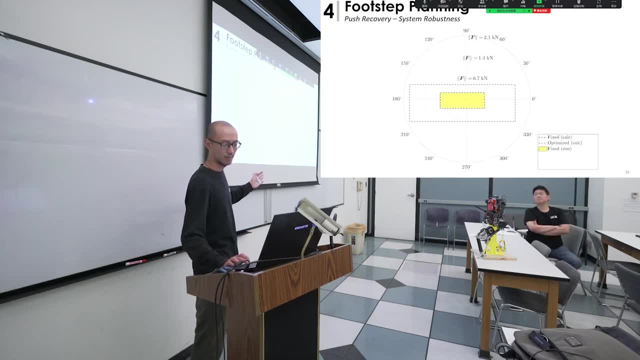 And this is only for the system robustness. So again, when n is increasing, the force, region expands, But, as you can see, it's also approaching some sort of converged to something. Yeah, So that's for the system robustness. 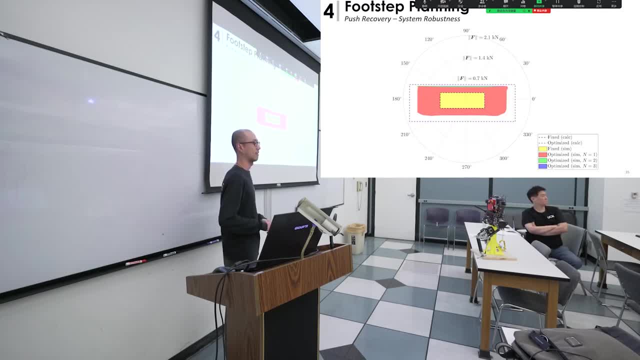 So if your height and your mass change? Yeah, that's a good question, So I didn't check, but I will just assume they should be close. And lastly, based on building up this would you say, the inverted pendulum model is a. 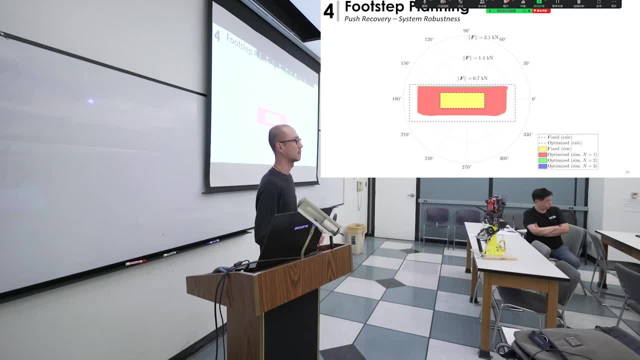 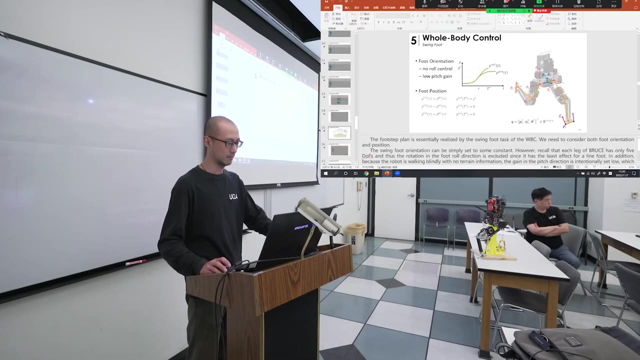 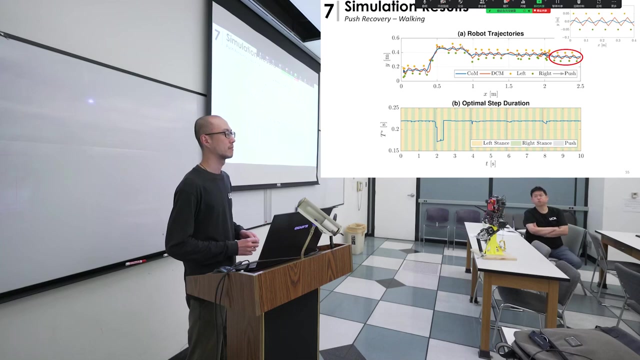 so at one point you showed your simulation model and your actual graph. Yeah, And they were similar. Yes, What motivated you to choose to pursue the inverted pendulum model as opposed to some other more complex model? Okay, So I guess my question is: 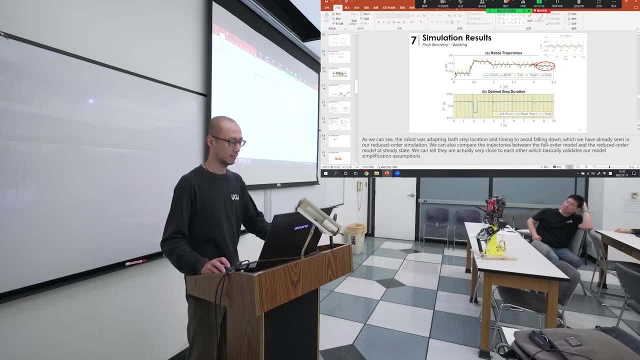 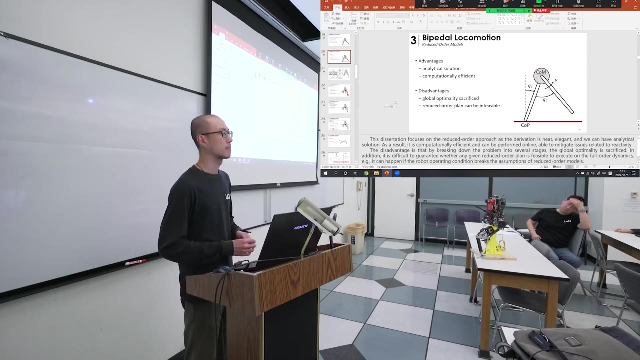 Yeah, We know that the model can capture some dynamics of the model. Yes, But it's not. obviously, it's still incorrect. However, I guess what gives you the hint that this is good enough? This is, the model is good enough. 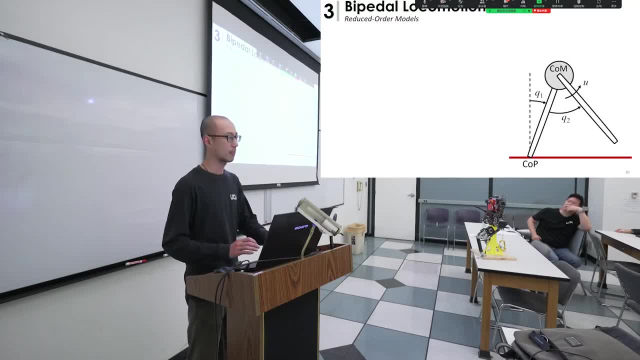 Yeah, the model. this model is good enough. We don't need anything more complex. So we definitely need more complexity, But given the current computational power, this is maybe the best we can do. Okay, So the first thing why I choose to reduce all the model is because this is the advantage. 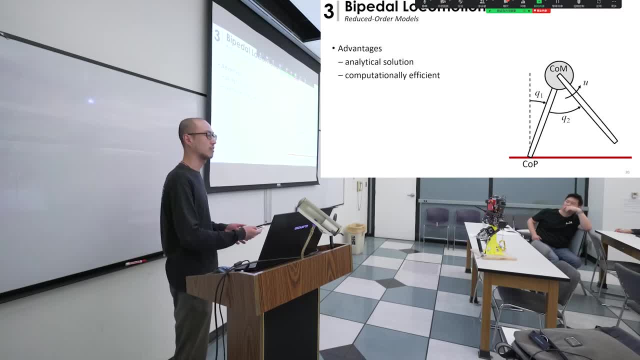 Because we have analytical solution. It's computation efficient. Okay, Everything is optimal. So this is so. this is at the beginning. it's only for working. Okay, At the beginning, the model is only for working. But once I add the flight phase, I'm still using this model.